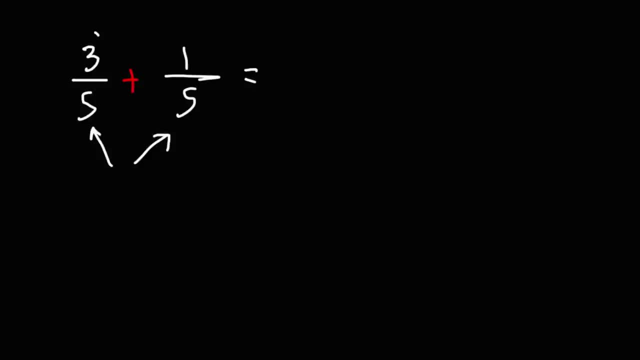 If the denominator of the two fractions are the same, you can simply add the numerators of the two fractions. So 3 plus 1 is 4, so this is 4 over 5.. So let's say if we have 7 over 8, and we want to subtract it by 3 over 8.. 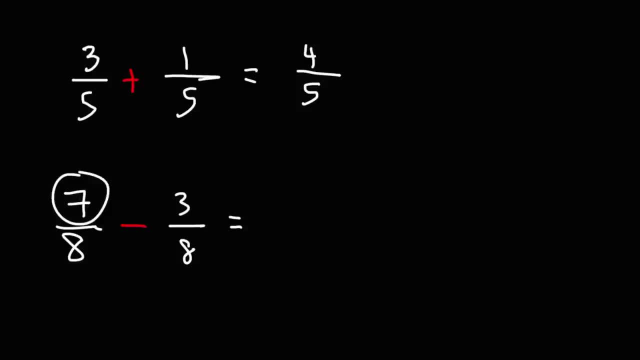 Since these two are the same, we can go ahead and subtract 7 by 3.. 7 minus 3 is 4, so we get 4 over 8.. Now, 4 over 8, we can simplify this fraction. We can reduce it. 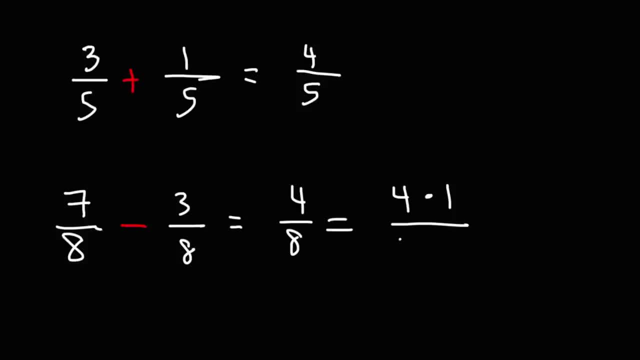 4 is the same as 4 times 1.. 8 is 4 times 1.. 8 is 4 times 2.. If we cancel the 4, then we get this fraction 1 over 2.. So that's the answer to the second problem, That's 7 over 8 minus 3 over 8.. 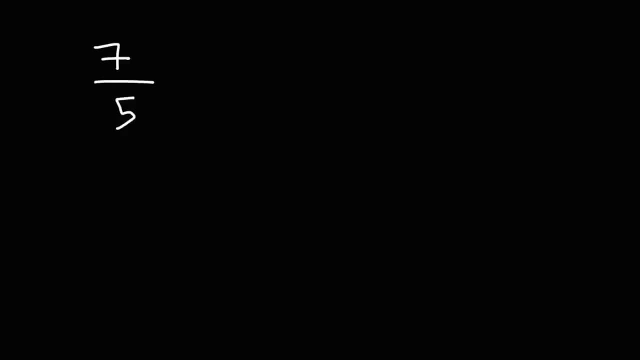 Now what about adding two fractions with unlike denominators? Let's say, if we want to add 7 over 5 with 1 over 4.. How can we do this? In order to add two fractions with unlike denominators, you need to adjust the fractions to get common denominators. 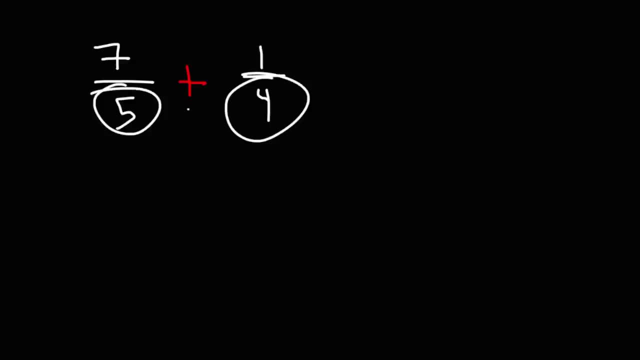 So we'll need to find the least common multiple of 5 and 4.. Multiples of four are 4,, 8,, 12,, 16,, 20, and so forth. Multiples of five are 5,, 10,, 15,, 20,, 25,, 30, and so forth. 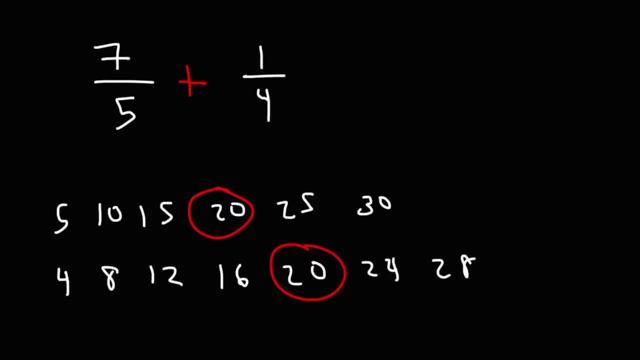 And the common multiple here is 20.. 20 is the least common multiple of 5 and 4.. If we were to continue this, another common multiple will be 40. But 40 is not the least common multiple, So we want to get the denominator to 20.. 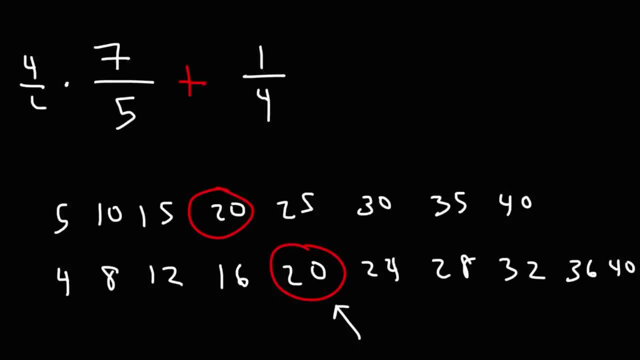 In order to do that, we need to multiply the first fraction by 4 over 4, and the second one by 5 over 5.. 4 times 7 is 28.. 4 times 5 is 20.. And then we have 5 times 1,, which is 5.. 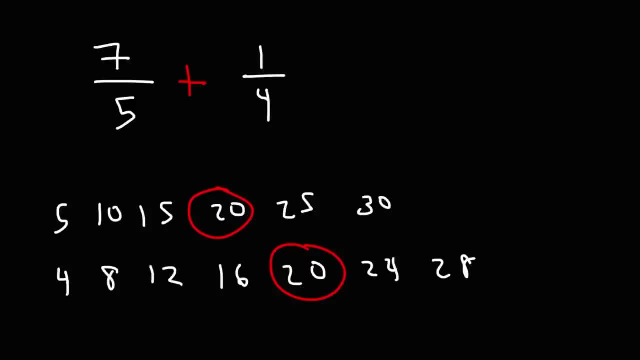 And the common multiple here is 20.. 20 is the least common common multiple of 5 and 4.. If we were to continue this, another common multiple will be 40, but 40 is not the least common multiple, So we want to get the denominator to 20.. In order to do that, 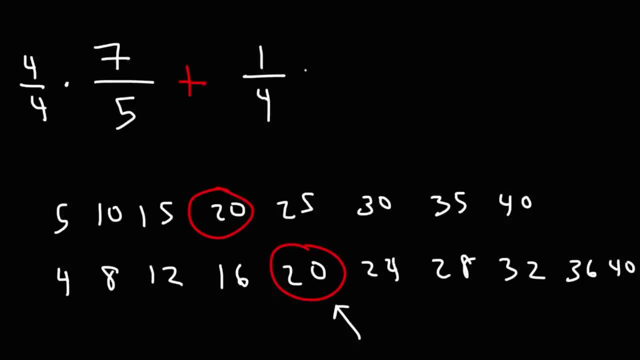 we need to multiply the first fraction by 4 over 4, and the second one by 5 over 5.. 4 times 7 is 28.. 4 times 5 is 20, and then we have 5 times 1,, which is 5.. 5 times 4 is. 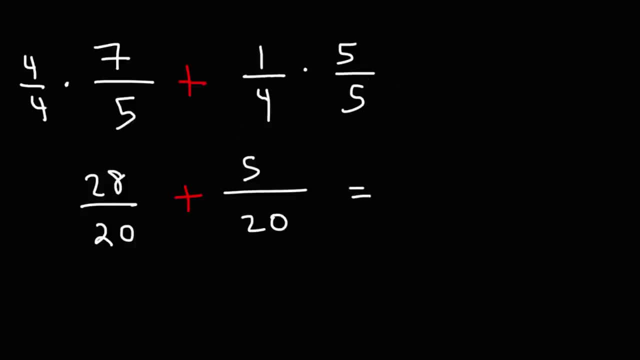 20.. So now that we have the same denominator, we can go ahead and add the numerator to the two fractions. 28 plus 5 is 33. the final answer for this problem it's 33 over 20. now what about this problem? what's 3 over 4 minus 2 over 7? feel free to try that, so we'll. 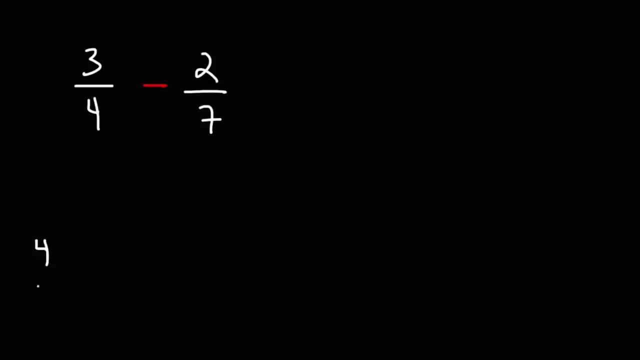 need to get common denominators. we could use any common multiple of 4 and 7. we could use the least common multiple or the next higher common multiple. one way to quickly get a common multiple in 4 and 7 is simply to multiply the two: 4. 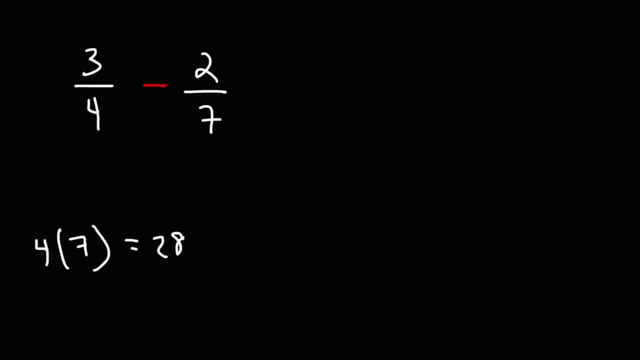 times 7 is 28, so we want to get a common denominator of 28, so we're going to multiply this fraction by this number, that is, by 7 over 7. we're going to multiply this fraction using this number, that is, by 4 over 4. 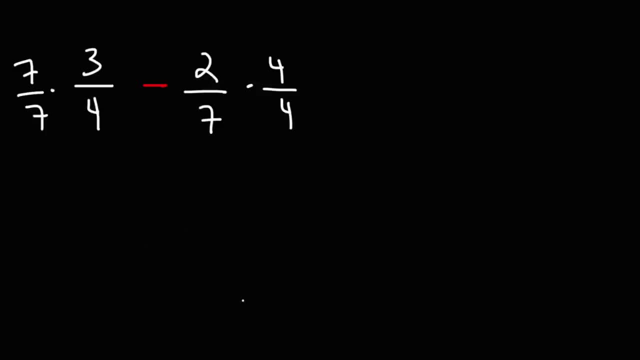 7 times 3 is 21, 7 times 4 is 28, 2 times 4 is 8, and 7 times 4 is still going to be 28. so now that we have the same denominator, we can subtract 21 by 8: 21. 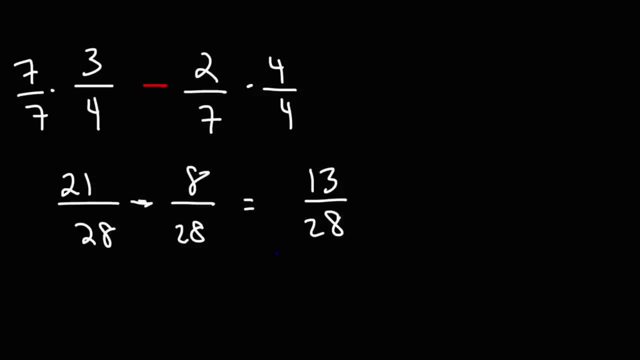 minus 8 is 28. so we can subtract 21 by 8. 21 minus 8 is 28. so now that we have the same denominator, we can subtract 21 by 8. 21 minus 8 is 13. so the final answer is 13 over 28. for this problem, now let's work on an 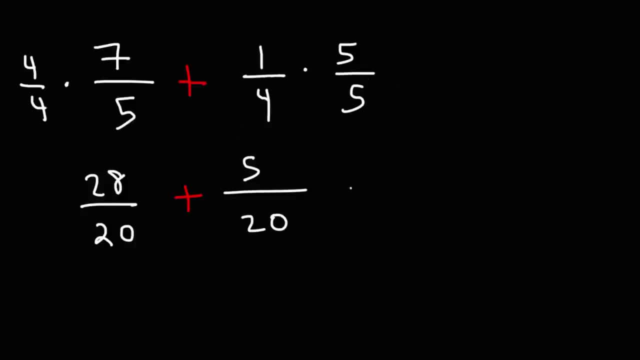 And then 5 times 4, which is 20.. So now that we have the same denominator, we can go ahead and add the numerator to the two fractions. So 28 plus 5 is 33.. The final answer for this problem it's 33 over 20.. 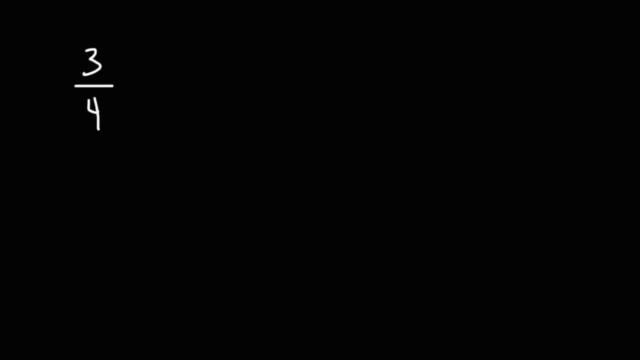 Now what about this problem? What's 3 over 4 minus 2 over 7? Feel free to try that. So we'll need to get common denominators. We could use any common denominator. We could use a common multiple of 4 and 7.. 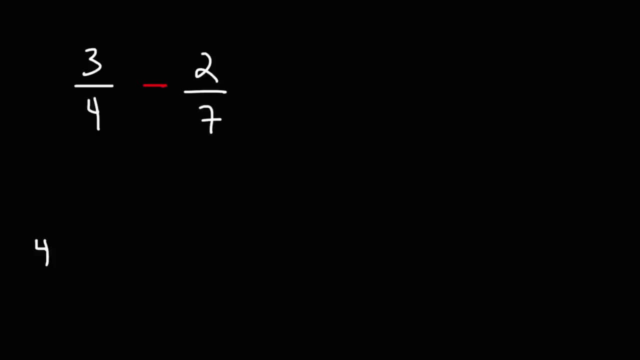 We could use the least common multiple or the next higher common multiple. One way to quickly get a common multiple of 4 and 7 is simply to multiply the two. 4 times 7 is 28.. So we want to get a common denominator of 28.. 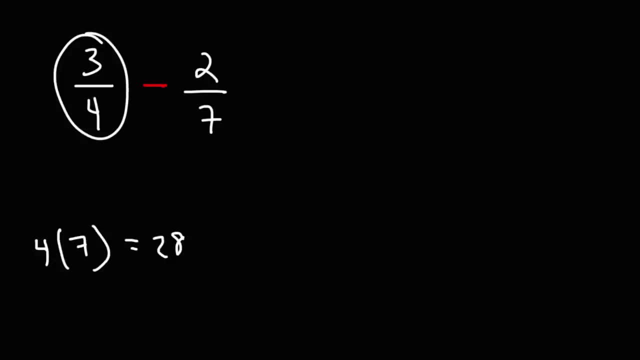 So we're going to multiply this fraction by this number, That is, by 7 over 7.. And we're going to multiply this fraction using this number, That is, by 4 over 4.. So we're going to multiply this fraction by this number. 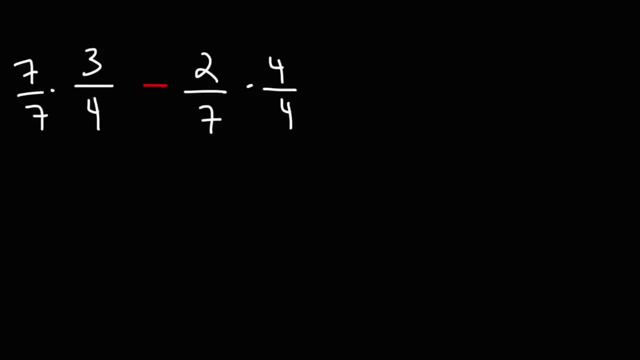 And we're going to multiply this fraction by this number. So we're going to multiply this fraction by this number: 7 times 3 is 21.. 7 times 4 is 28.. 2 times 4 is 8.. 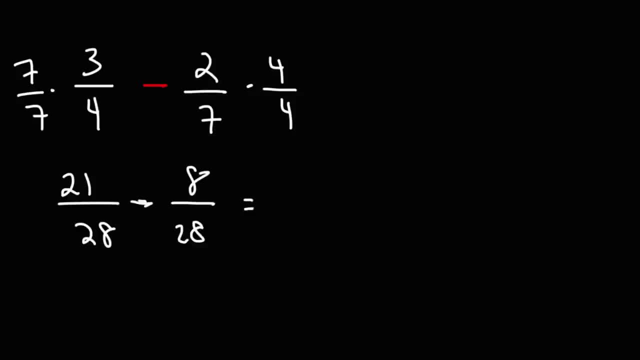 And 7 times 4 is still going to be 28.. So now that we have the same denominator, we can subtract 21 by 8.. 21 minus 8 is 13.. So the final answer is 13 over 28.. 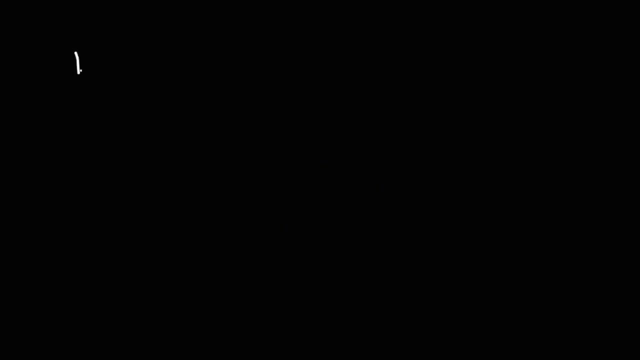 For this problem. Now let's work on an example with three fractions. So let's say we want to add 1 over 3, plus 2 over 5 and then minus 3 over 4.. Go ahead and combine those three fractions. 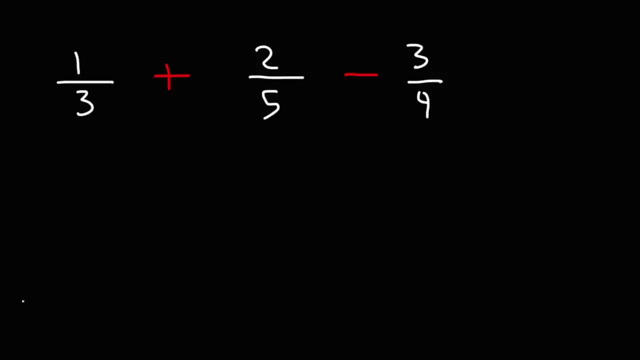 So what we need to do is we need to get common denominators. If we multiply 3 by 5, by 4, we can get a common multiple of the three fractions. 5 times 4 is 20.. 20 times 3 is 60.. 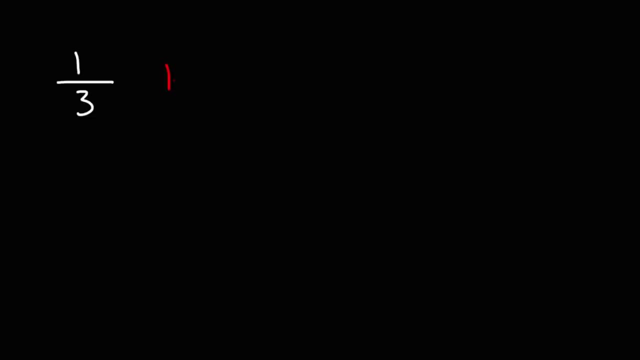 example, with 3 fractions. so let's say we want to add 1 over 3 plus 2 over 5, minus 3 over 4. go ahead and combine those three fractions fractions. So what we need to do is we need to get common denominators. If we multiply 3 by 5, 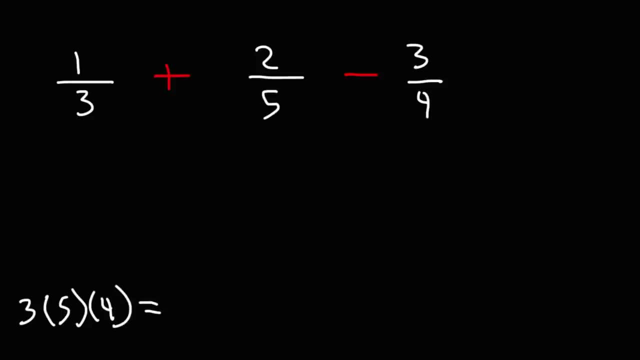 by 4, we can get a common multiple of the three fractions. 5 times 4 is 20.. 20 times 3 is 60.. So we want to get a common denominator of 60.. 60 divided by 3 is 20.. So I'm going to multiply this. 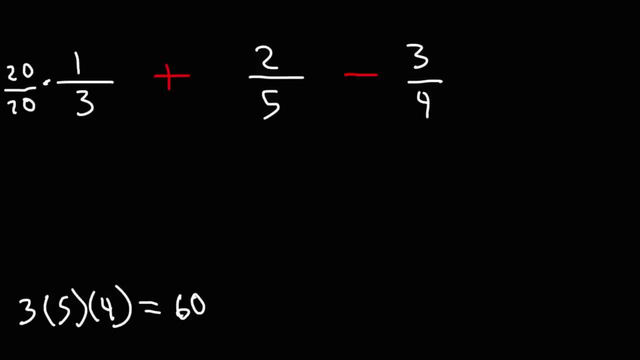 fraction by 20 over 20.. 60 divided by 5 is 12.. So I'm going to multiply this fraction- the top and the bottom- by 12.. And 60 divided by 4 is 15.. So I'm going to multiply this fraction by 15 over. 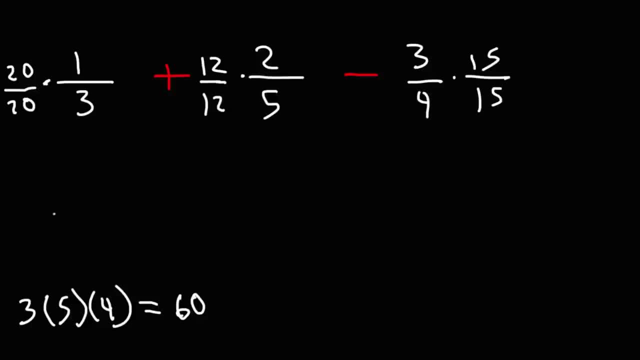 15.. So here I have 20 times 1,, which is 20, and then 20 times 3,, that's 60. Next I have 2 times 12 is 24.. And we know, 12 times 5 is 60.. 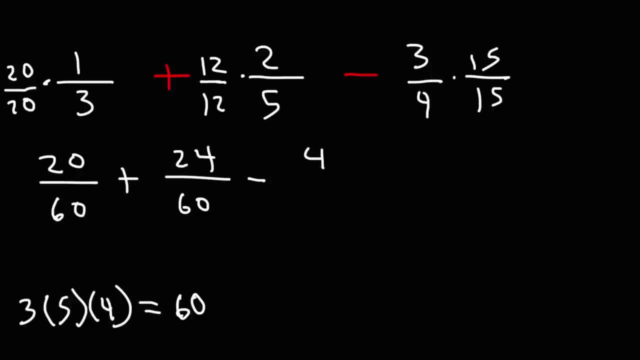 And then 3 times 15 is 45.. 4 times 15 is 60.. So now we can add 20 plus 24, that's 44. And then 44 minus 45 is negative 1.. So the final answer is going to be negative 1 over 60. 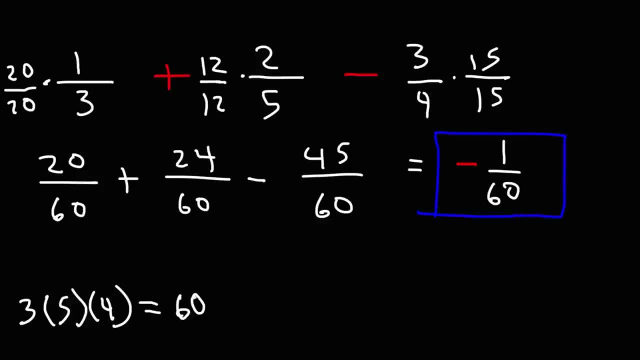 So the final answer is going to be negative: 1 over 60.. So the final answer is going to be negative: 1 over 60.. So that's what you can do if you need to add or subtract three fractions. Let's try another example. So let's say we have 2 over 3,. 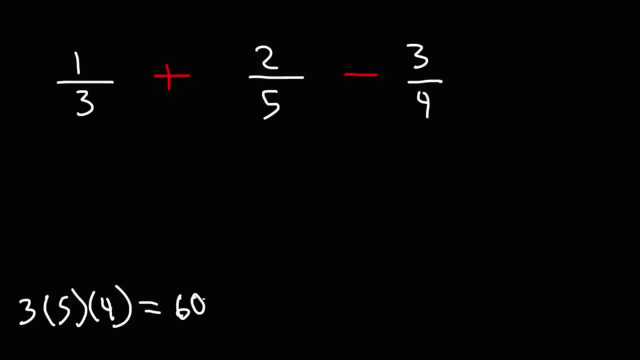 So we want to get a common denominator of 60.. 60 divided by 3 is 20.. So I'm going to multiply this fraction by 20 over 20.. 60 divided by 5 is 12.. So I'm going to multiply this fraction. 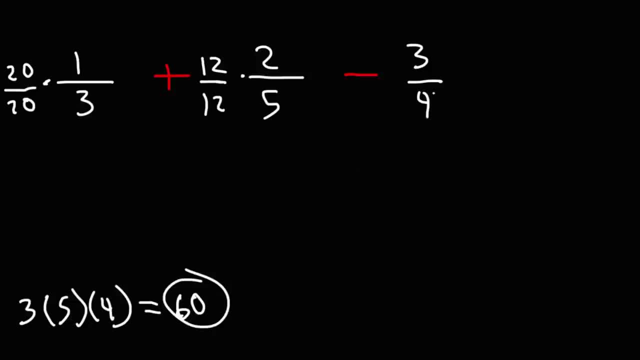 the top and the bottom by 12.. And 60 divided by 4 is 15.. So I'm going to multiply this fraction by 15 over 15.. So here I have 20 times 1, which is 20.. And then 20 times 3,, that's 60.. 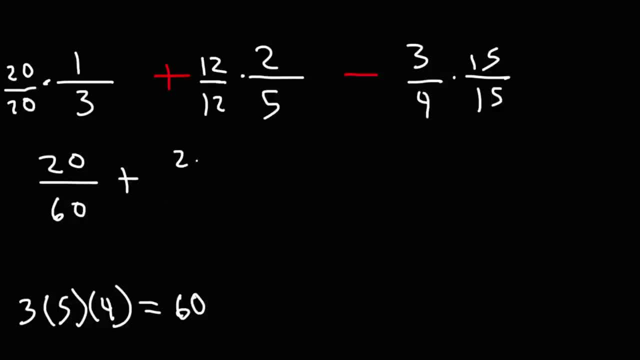 Next I have: 2 times 12 is 24.. And we know 12 times 5 is 60. And then 3 times 15 is 45.. 4 times 15 is 60. So now we can add 20 plus 24, that's 44.. 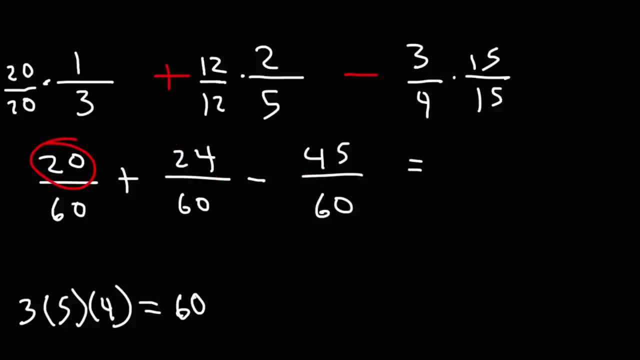 And then 44 minus 45 is negative 1.. So the final answer is going to be negative 1 over 60.. So that's what you can do if you need to add or subtract three fractions. Let's try another example. So let's say we have 2 over 3.. 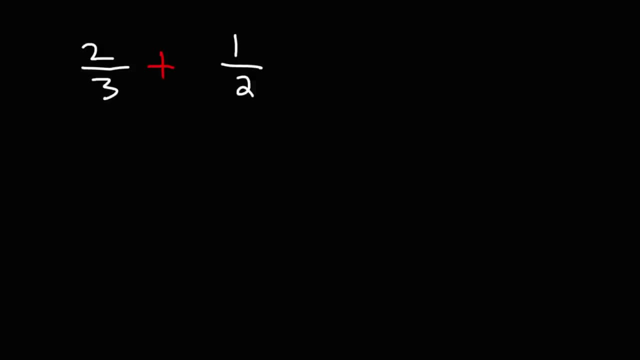 And then plus 1 over 2, minus 3 over 4.. So go ahead and combine those three fractions. So we need to get common denominators. If we multiply 3 by 2 and by 4, 3 times 2 is 6, 6 times 4 is 24.. 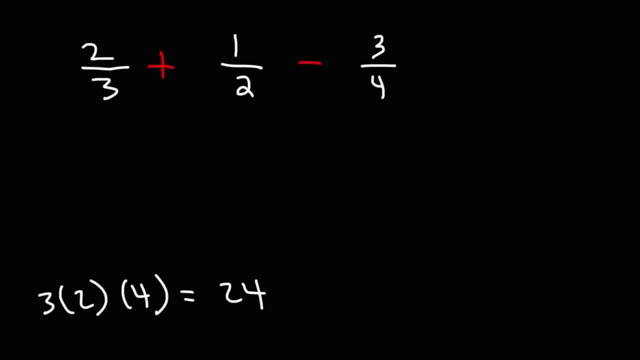 So 24 is a common multiple of these three numbers. It's not the lowest common multiple, but it is a multiple of those three numbers. The lowest common multiple, it turns out, is 12.. 12 is divisible by 3,, 2, and 4.. 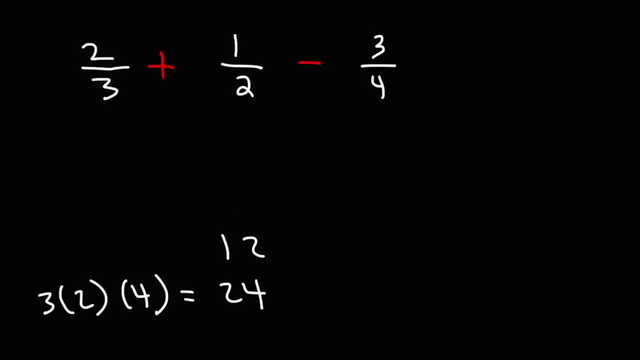 So let's get a denominator of 12 for each of these three fractions. 12 divided by 3 is 4.. So we're going to multiply this fraction by 4 over 4.. 12 divided by 2 is 6.. 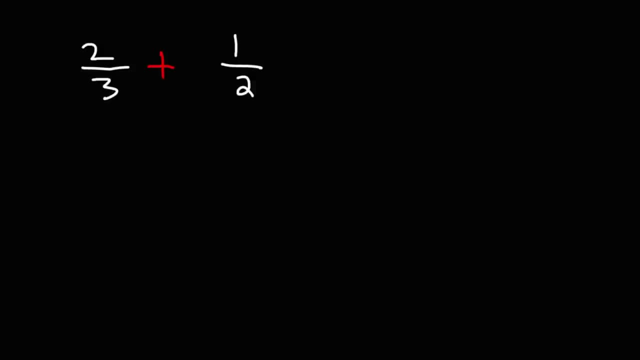 and then plus 1 over 2,, minus 3 over 4.. So go ahead and combine those three fractions, So we'll need to get common denominators. If we multiply 3, by 2 and by 4, 3 times 2 is 6, 6 times 4 is 24.. So 24 is a common multiple of. 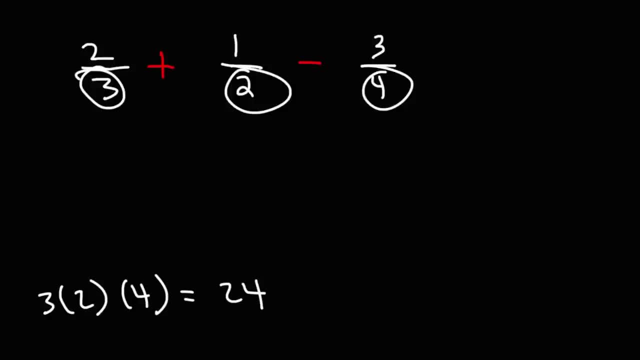 these three numbers. It's not the lowest common multiple, but it is a multiple of those three numbers. The lowest common multiple, it turns out, is 12.. 12 is divisible by 3,, 2, and 4.. So let's get a denominator. 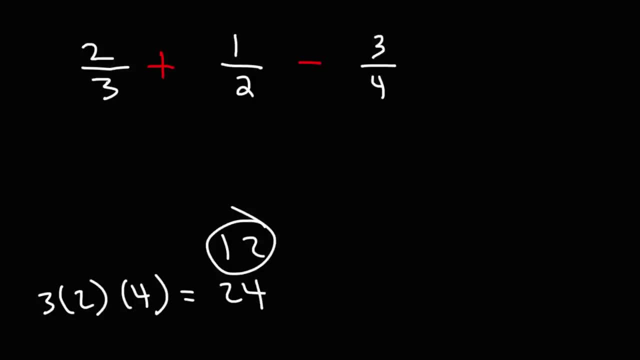 So let's get a denominator of 3,, 2, and 4.. So let's get a denominator of 3,, 2, and 4.. 12 for each of these three fractions. 12 divided by 3 is 4.. So we're going to multiply this. 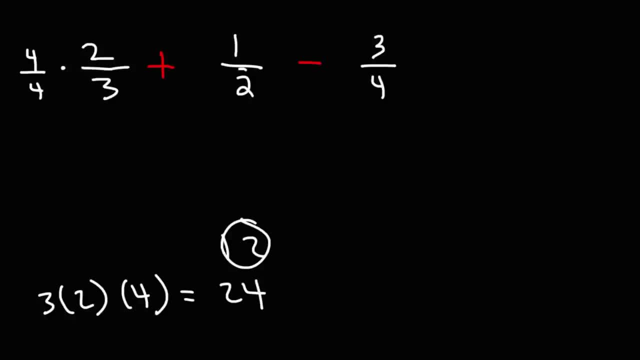 fraction by 4 over 4.. 12 divided by 2 is 6.. So we'll multiply this one by 6 over 6.. And 12 divided by 4 is 3.. So we'll multiply this one by 3 over 3.. So here we have 4 times 2, which is 8.. 4 times. 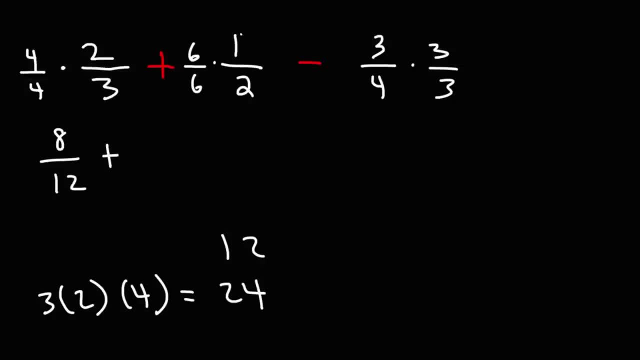 3 is 12.. Next we have 6 times 1,, which is 6.. 6 times 2 is 12.. And then 3 times 3 is 9.. And on the bottom, 4 and 3, we know it's 12.. 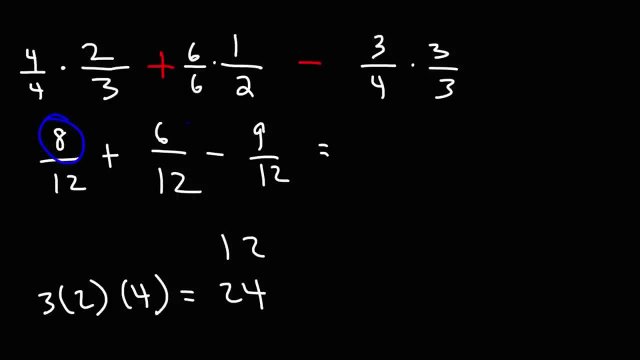 So now let's add the numerators of the fractions. 8 plus 6 is 14.. 14 minus 9 is 5.. So the final answer for this problem is 5 over 12.. So let's add the numerators of the fractions. 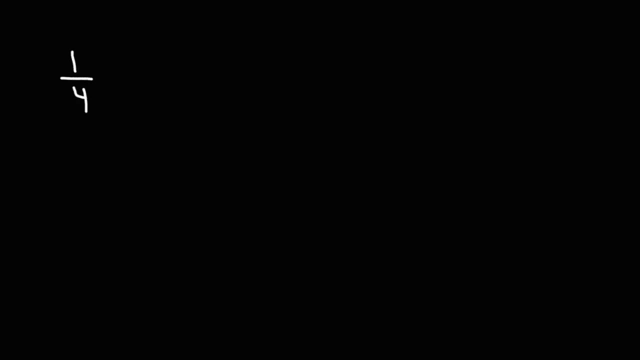 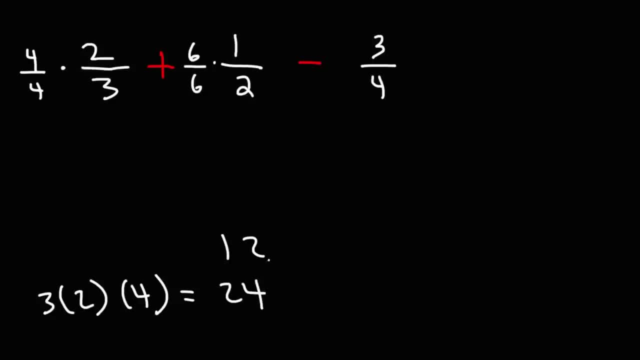 So we'll multiply this one by 6 over 6.. And 12 divided by 4 is 3.. So we'll multiply this one by 3 over 3.. So here we have 4 times 2, which is 8.. 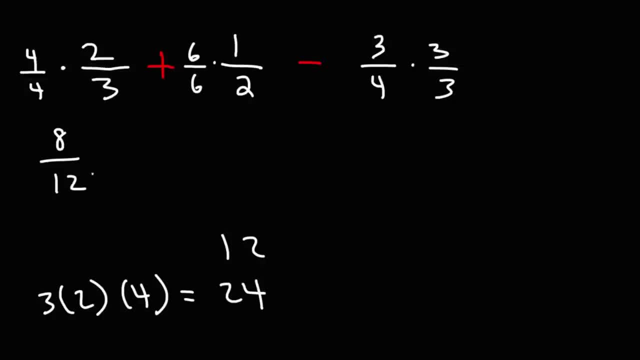 4 times 3 is 12.. Next we have 6 times 1,, which is 6.. 6 times 2 is 12.. And then 3 times 3 is 9.. And on the bottom, 4 and 3, we know it's 12.. 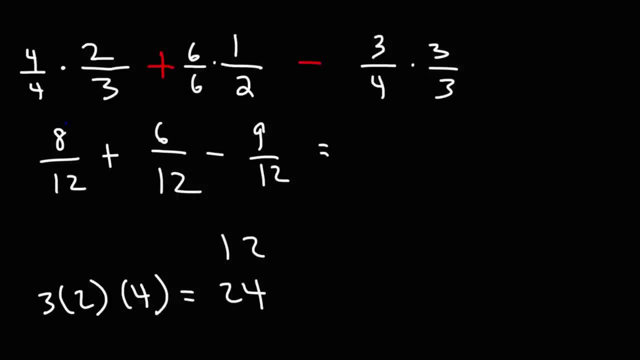 So now let's add the numerators of the fractions: 8 plus 6 is 14.. 14 minus 9 is 5.. So the final answer for this problem is 5 over 12.. Now let's try an example where we're. 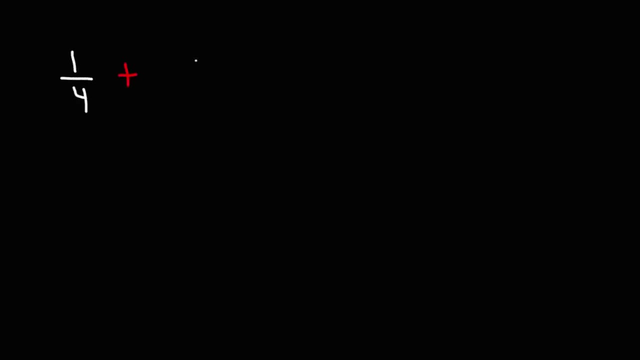 adding or subtracting a combination of 4 fractions. Go ahead and try that. What's 1 over 4 plus 2 over 5, minus 1 over 3 plus 5 over 6?? So what number goes into 4,, 5,, 3, and 6?? 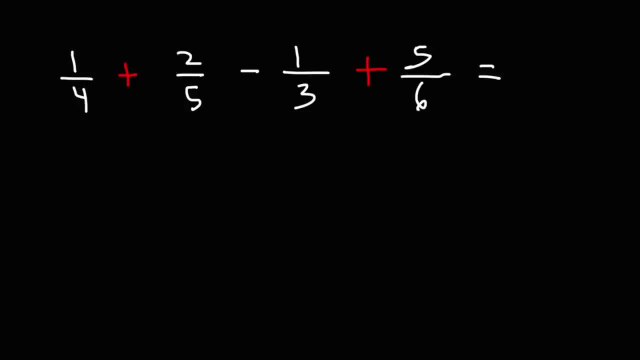 We need to find a common denominator. A quick and simple way is to multiply all of these numbers, But if we do, we're going to get something pretty big. I would go with 60.. 60 is divisible by 6,, 3,, 4, and 5.. 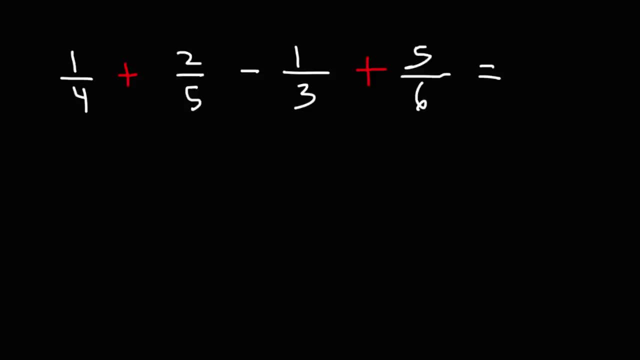 Now, if you're wondering how I got 60, well here's how you can do it: If we were to multiply 4 and 5,, that would be 20 times 3 is 60, times 6 is 360.. 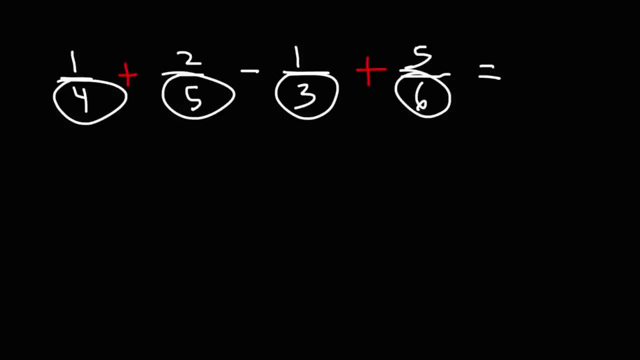 360 is a common multiple of all four of those numbers. What we need is a smaller number that contains the factors of 4, 5,, 3, and 6.. Factors of 4 are 2 and 2, 5,. you can write that as: 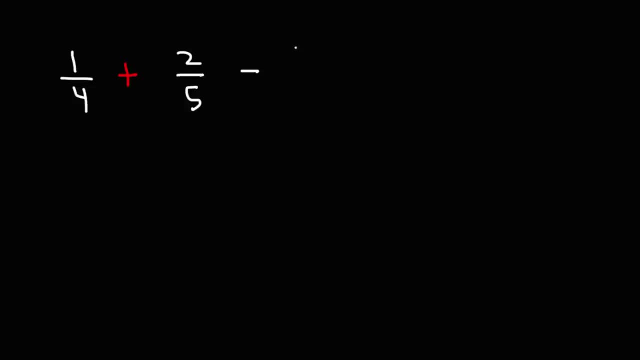 Let's try an example where we're adding or subtracting a combination of four fractions. Let's try an example where we're adding or subtracting a combination of four fractions. Let's try an example where we're adding or subtracting a combination of four fractions. 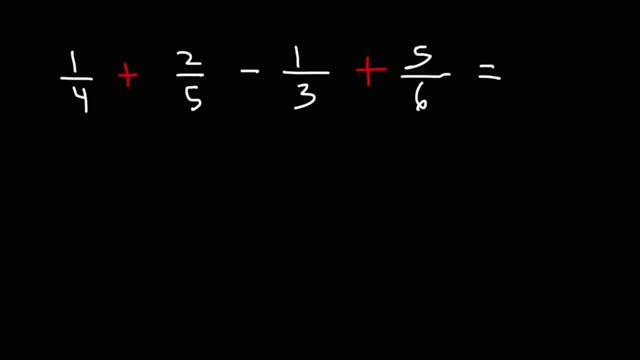 Go ahead and try that: What's 1 over 4 plus 2 over 5, minus 1 over 3 plus 5 over 6?? So what number goes into 4,, 5, 3, and 6?? 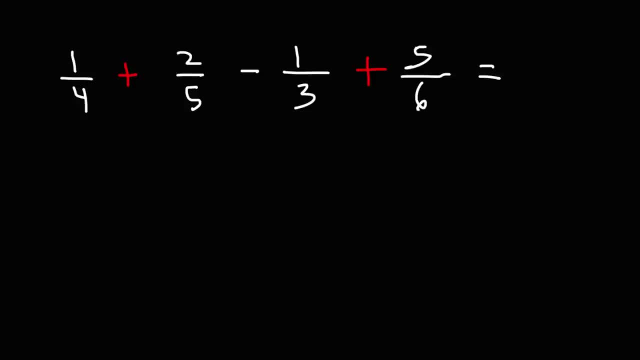 We need to find a common denominator. A quick and simple way is to multiply all of these numbers, But if we do, we're going to get something pretty big. I would go with 60.. 60 is divisible by 6,, 3,, 4, and 5.. 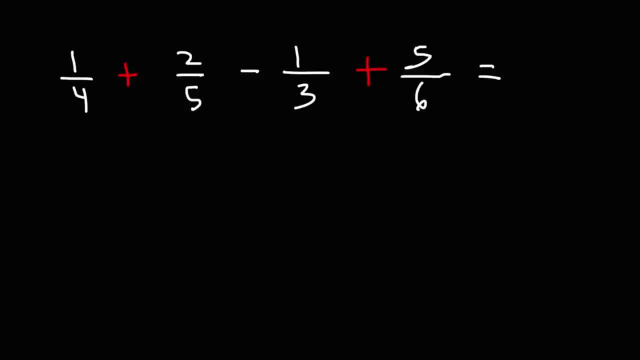 Now, if you're wondering how I got 60, well here's how you can do it: If we were to multiply 4 and 5, that would be 20 times 3 is 60 times 6 is 360.. 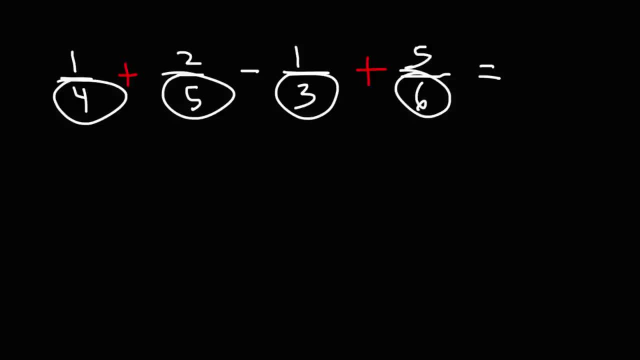 360 is a common multiple of all four of those numbers. What we need is a smaller number that contains the factors of 4,, 5,, 3, and 6.. Factors of 4 are 2 and 2.. 5, you can write that as 5 and 1,, but I'll just leave it as 5.. 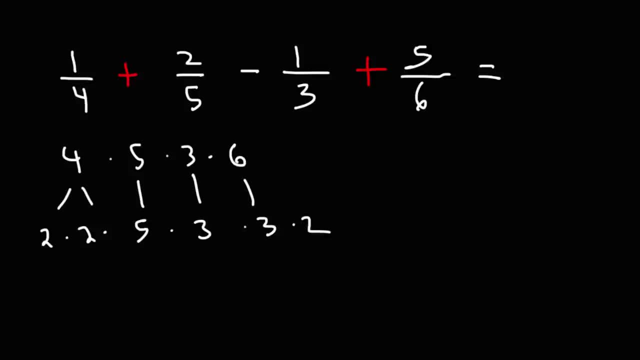 3,, I'm not going to break it up. 6, that's 3 and 2.. Now notice that we really don't need to use the 6 here, because we already have a 2 and a 3,, which will give us 6.. 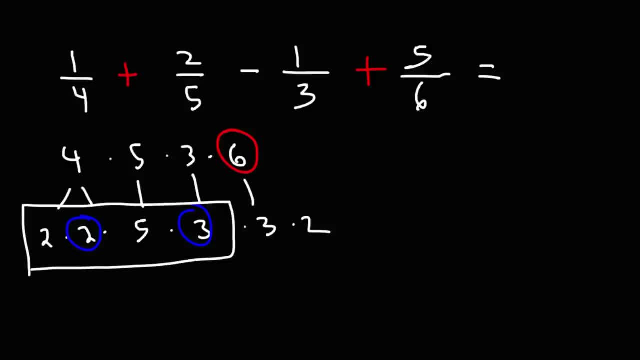 So if we multiply these four numbers, that result is going to be divisible by 4 because it has 2 times 2 in it. It's going to be divisible by 5 because it has a 5 in it. It's divisible by 3 because it has a 3 in it. 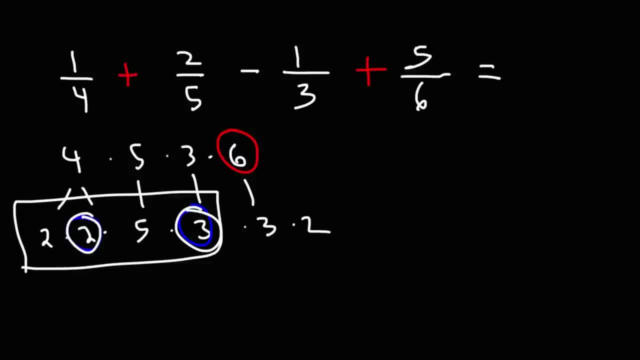 And it's divisible by 6 because it has 2 times 3, which is 6 in it. So we don't need to multiply by this extra number, because we already have a 6 in this number. 2 times 2 is 4, times 5 is 20, times 3 is 60. 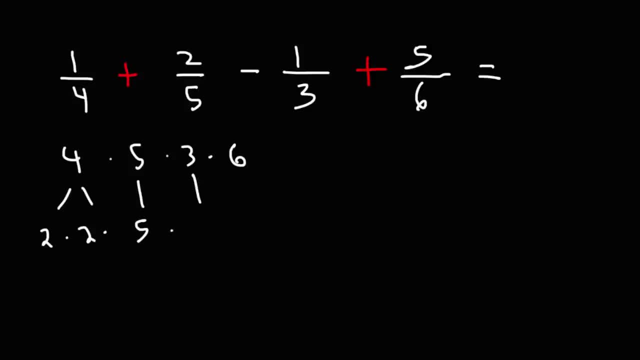 5 and 1,, but I'll just leave it as 5.. 3,- I'm not going to break it up. 6, that's 3 and 2.. Now notice that we really don't need to use the 6 here. 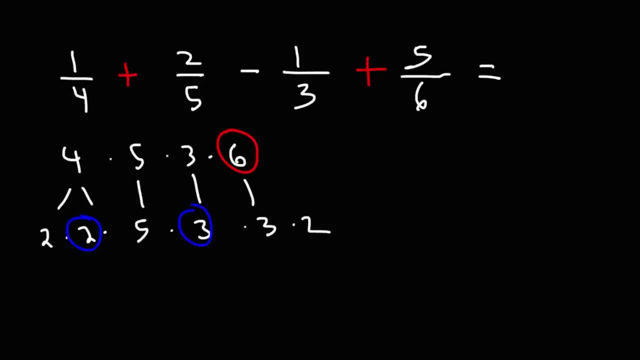 Because we already have a 2 and a 3, which will give us 6.. So if we multiply these four numbers, that result is going to be divisible by 4 because it has 2 times 2 in it. It's going to be divisible by 5 because it has a. 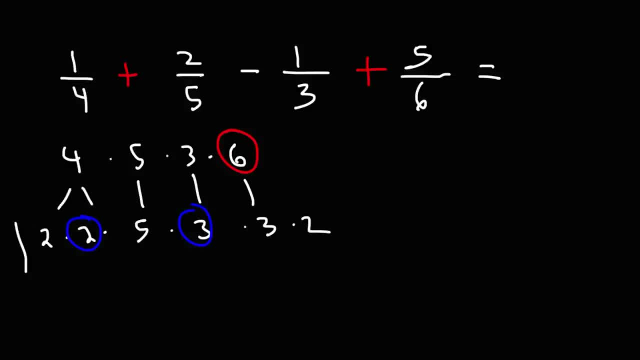 5 in it. It's divisible by 3 because it has a 3 in it And it's divisible by 6 because it has 2 times 3, which is 6 in it. So we don't need to multiply by this extra number, because. 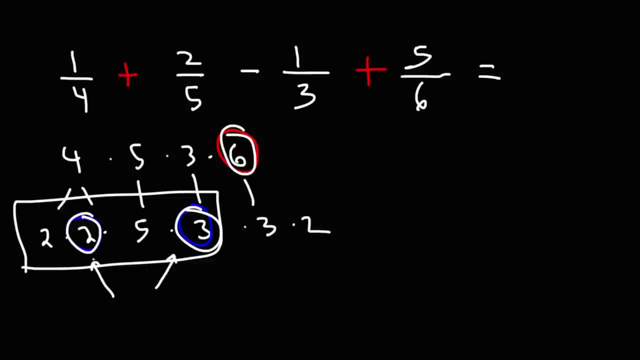 we already have a 6 in this number. 2 times 2 is 4, times 5 is 20, times 3 is 60. So that's why 60 is the least common multiple of 4, 5,. 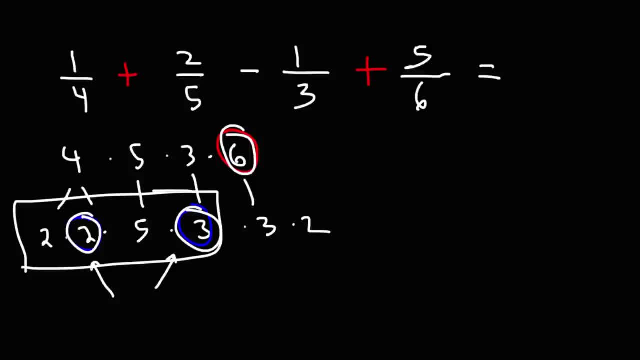 3, and 6.. It's because within 60, you have factors that will multiply to any one of these numbers. So that's how you can get 60 without writing out all the multiples of each number. So now that we know that 60 is, 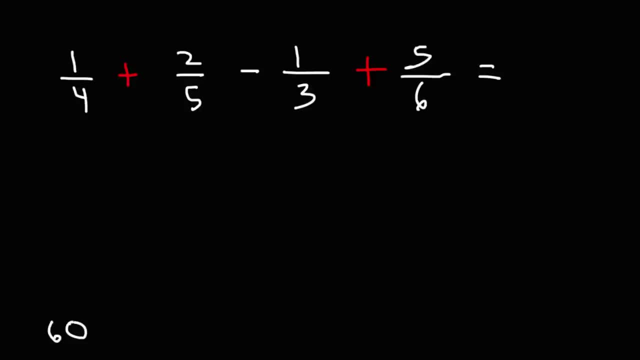 the common denominator that we're trying to get. let's go ahead and get it: 60 divided by 4 is 15.. So we're going to multiply this fraction by 15 over 15.. 60 divided by 5 is 12.. So we're going to. 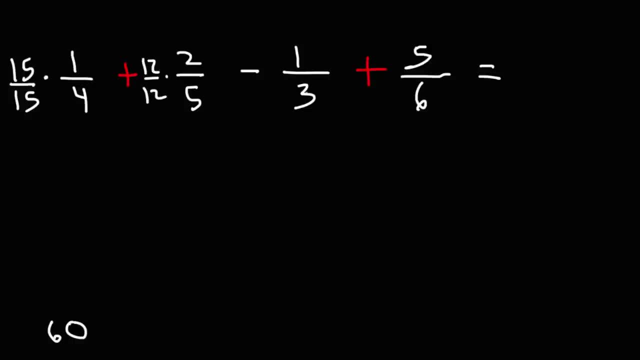 multiply this one by 12 over 12.. 60 divided by 3 is 20.. And 60 divided by 6 is 10.. So we'll multiply this one by 10 over 10.. So here we have 15 times 1,, which is 15.. 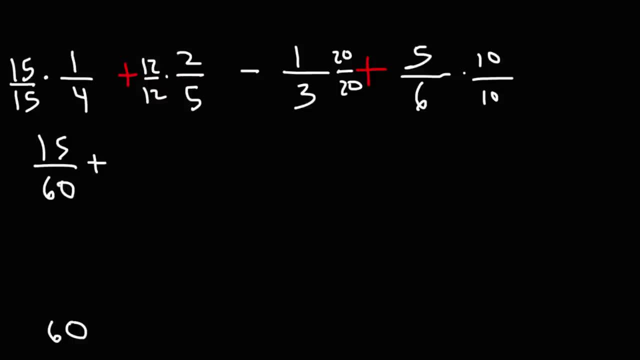 And then 12 times 2 is 24.. All of this, the denominators will be 60.. 1 times 20 is 20.. And then 5 times 10 is 50. So now what we need to do is add. 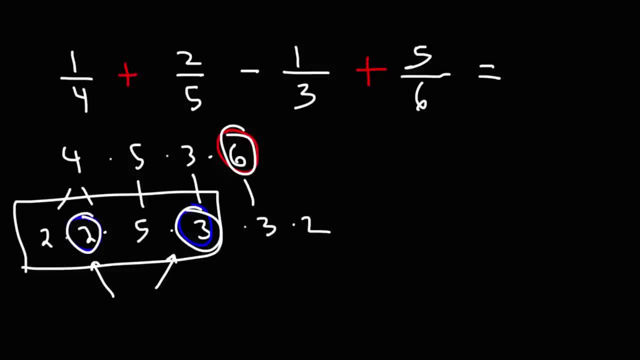 So that's why 60 is the least common multiple of 4,, 5,, 3, and 6.. It's because within 60, you have factors that will multiply to any one of these numbers. So that's how you can get 60. 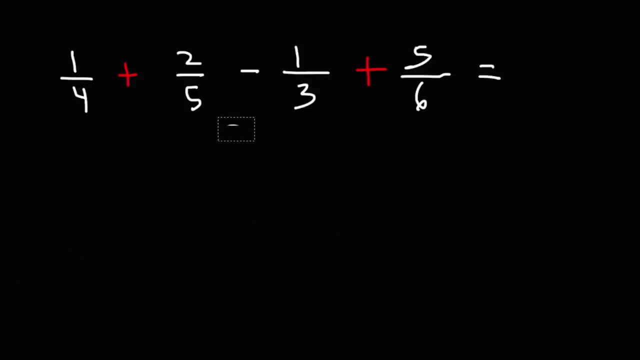 without writing out all the multiples of each number. So now that we know that 60 is the common denominator that we're trying to get, let's go ahead and get it: 60 divided by 4 is 15.. So we're going to multiply this fraction by 15 over 15.. 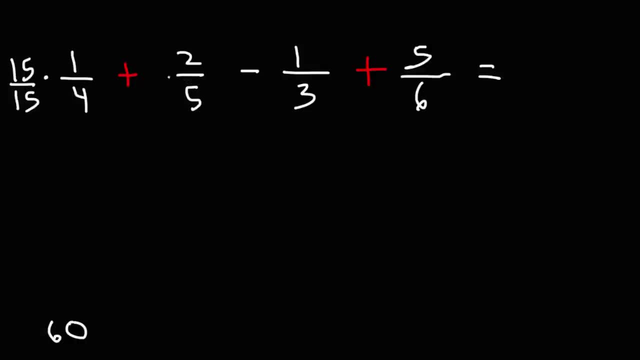 60 divided by 5 is 12.. So we're going to multiply this one by 12 over 12.. 60 divided by 3 is 20.. And 60 divided by 6 is 10.. So we'll multiply this one by 10 over 10.. 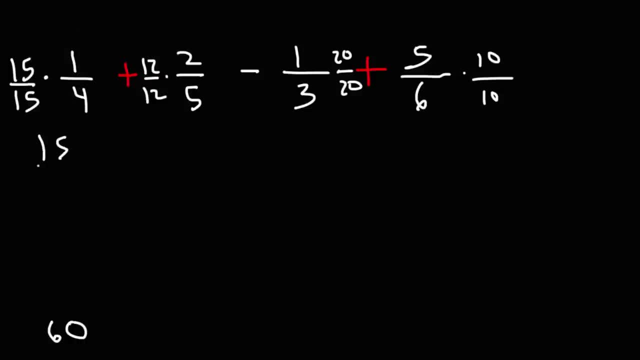 So here we have 15 times 1, which is 15.. And then 12 times 2 is 24.. All of the denominators, All of the denominators, will be 60.. 1 times 20 is 20.. 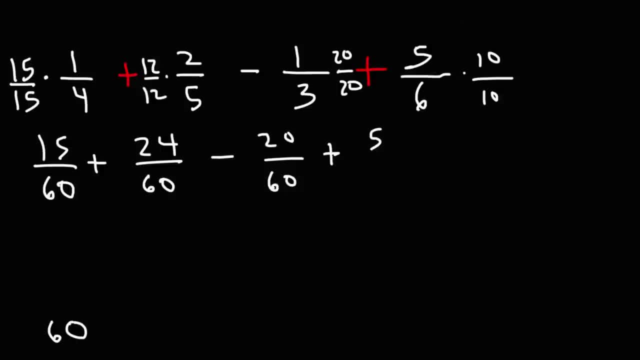 And then 5 times 10 is 50.. So now what we need to do is add. So let's add this one at a time: 15 plus 24,, that is 39.. Negative: 20 plus 50, or 50 minus 20,, that's positive: 30. 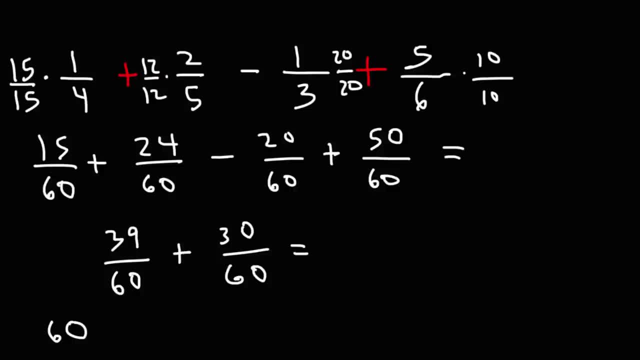 39 plus 30 is 69. So we get 69 over 60.. 69 is 23 times 3.. 60 is 20 times 3. So we can cancel the 3, and we'll be left with 23 over 20.. 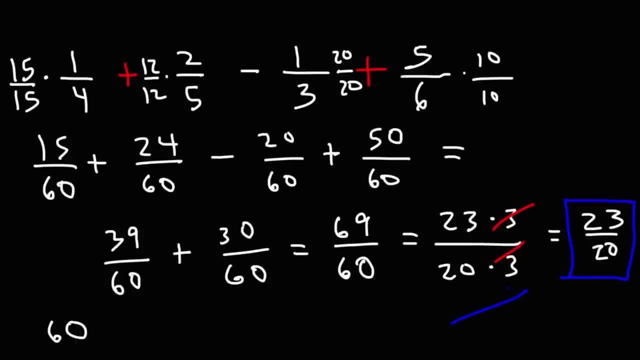 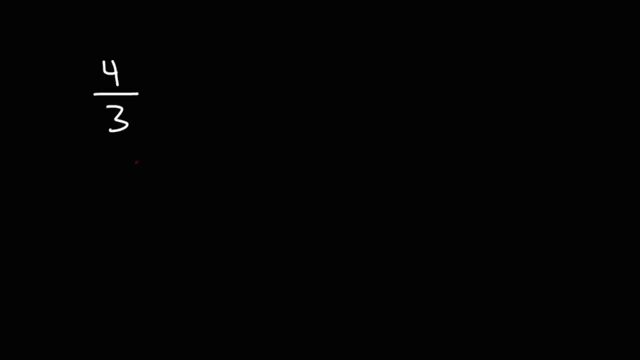 So this is going to be the sum of the four fractions. That's the final answer. Now let's move on to our next topic. Let's talk about how we can multiply two fractions. So what's 4 over 3 times 5 over 7?? 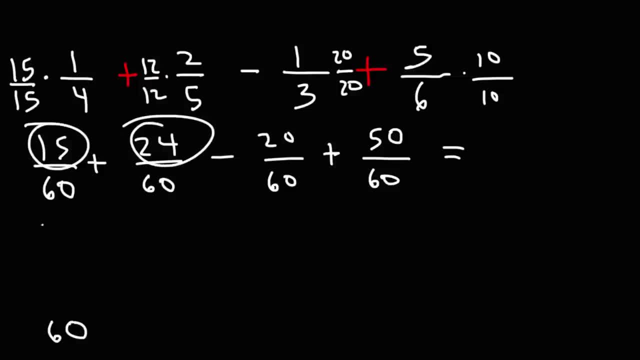 So let's add this one at a time: 15 plus 24,, that is 39.. Negative 20 plus 50, or 50 minus 20, is positive 30.. 39 plus 30 is 69.. So we get 69. 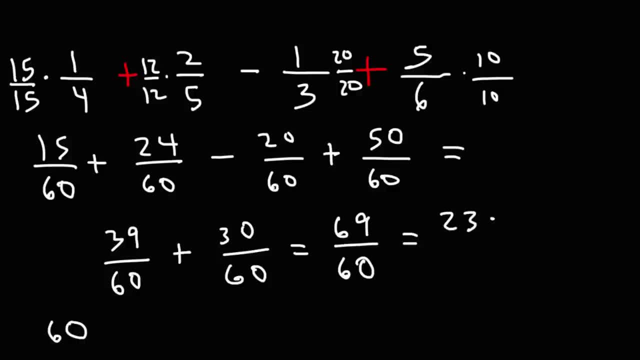 over 60.. 69 is 23 times 3.. 60 is 20 times 3.. So we can cancel the 3. And we'll be left with 23 over 20.. So this is going to be the sum of the 4 fractions. 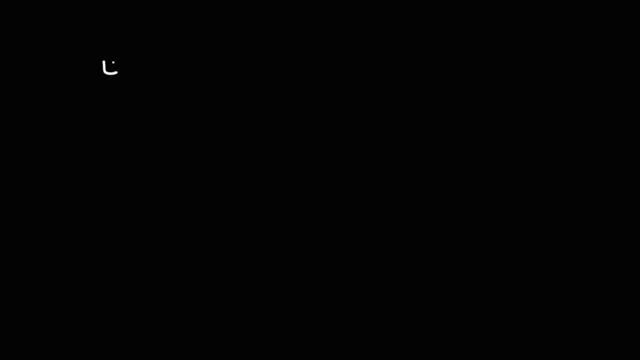 That's the final answer. Now let's move on to our next topic. Let's talk about how we can multiply 2 fractions. So what's 4 over 3 times 5 over 7?? If you see this dot or an x, it indicates: 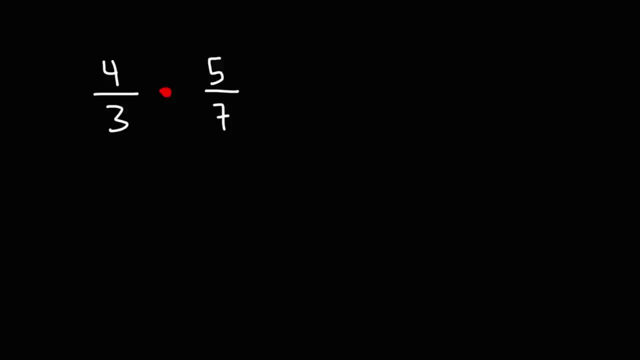 multiplication. In order to multiply 2 fractions, all you need to do is simply multiply across. 4 times 5 is 20.. 7 times 3 is 21.. So that's how we can multiply 2 fractions. So the final answer for this problem. 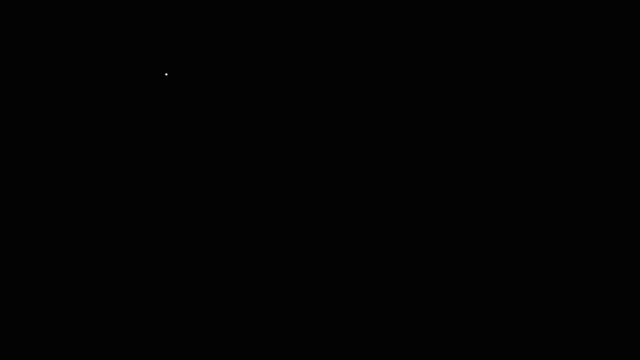 is 20 over 21.. Now let's try another example. Let's say we have 5 over 9, and we wish to multiply it by, let's say, 7 over 8.. Go ahead and try that. So this is going to be 5 times 7,. 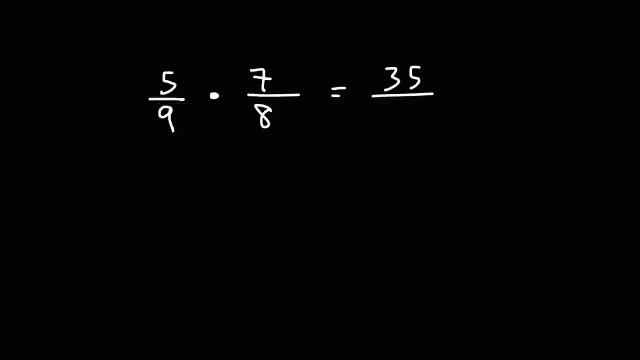 which is 35, divided by and 9 times 8 is 72. So our final answer is 35 over 72.. Try this 5 over 8 times. let's say 10 over 10 over 7.. Go ahead and multiply those 2.. 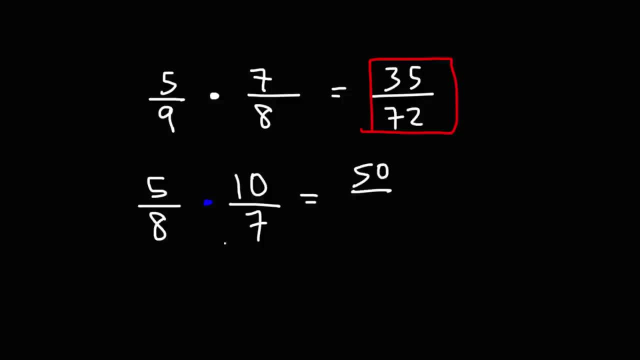 5 times 10 is 50.. 8 times 7 is 56.. Now we have 2 even numbers in this fraction, which means we can reduce it. 50 is 25 times 2. 56- well, we could say that's. 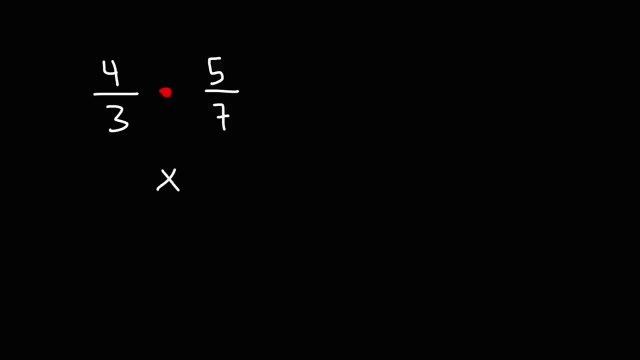 If you see this dot or an x, it indicates multiplication. In order to multiply two fractions, all you need to do is simply multiply across. 4 times 5 is 20.. 7 times 3 is 21.. So that's how we can multiply two fractions. 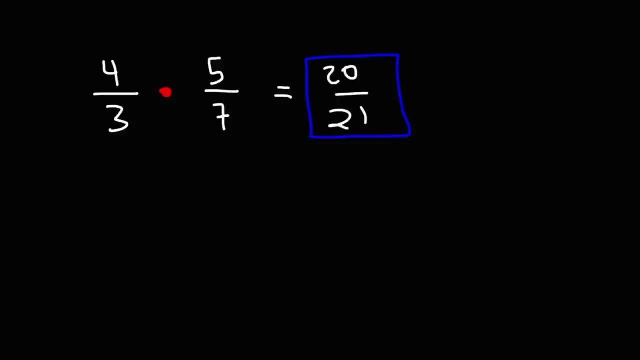 So the final answer for this problem is 20 over 21.. Now let's try another example. Let's say we have 5 over 9, and we wish to multiply it by, let's say, 7 over 8.. Go ahead and try that. 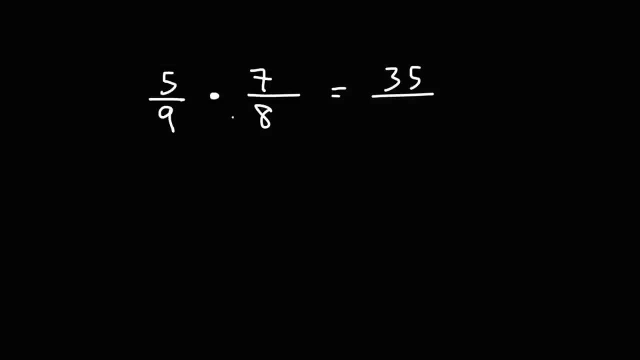 So this is going to be 5 times 7,, which is 35, divided by and 9 times 8 is 72.. So our final answer is 35.. So that's how we can multiply two fractions. Let's try this. 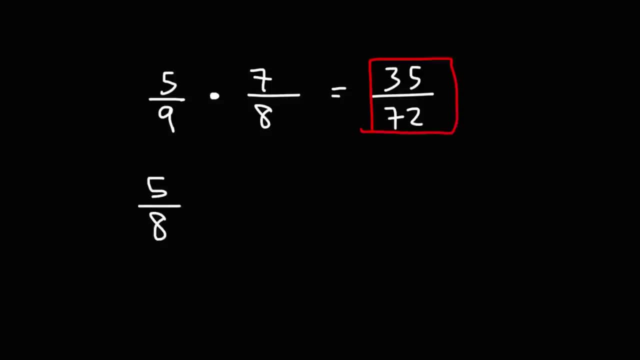 5 over 8 times. let's say 10 over 10 over 7.. Go ahead and multiply those two. 5 times 10 is 50.. 8 times 7 is 72.. So that's how we can multiply two fractions. 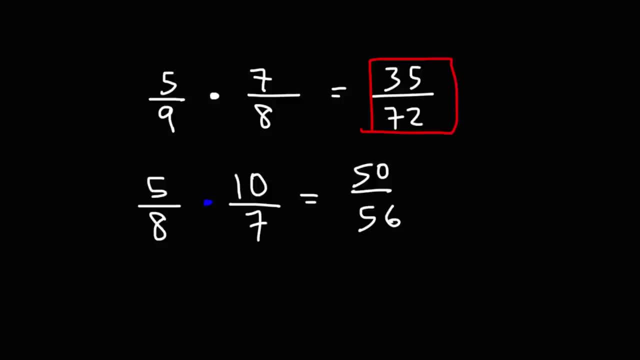 7 over 7 is 56.. Now we have two even numbers in this fraction, which means we can reduce it. 50 is 25 times 2.. 56,- well, we could say that's 28 times 2.. If we cancel a 2, we're left with 25 over 28 for our final answer. 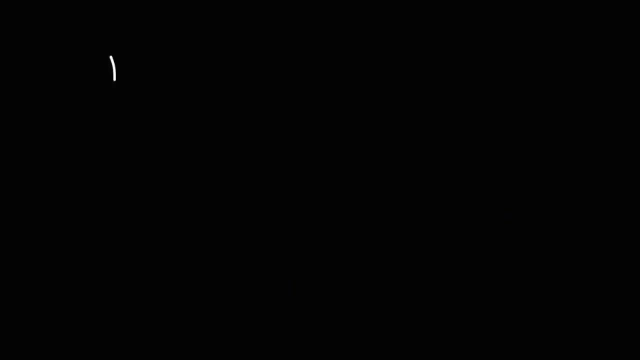 Now what about this one? 12 over 27 times 18 over 30. Go ahead and try that problem. Now. if we multiply across 12 times 18 is going to give us a big number. 27 times 30, that's another big number as well. 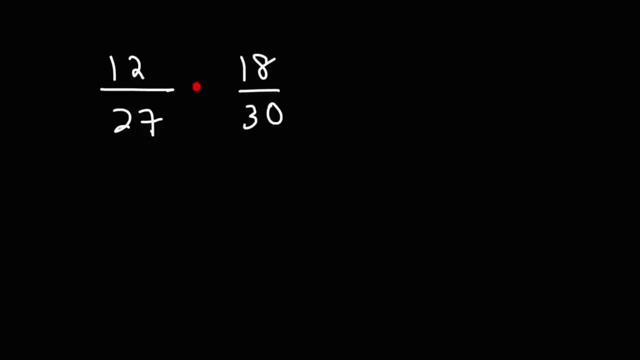 And then we'll have to reduce two big numbers. That's going to take a lot of work. Okay, Instead, it's better if we reduce these numbers now before we multiply and create an even bigger number: 27,. we can write that as 9 times 3.. 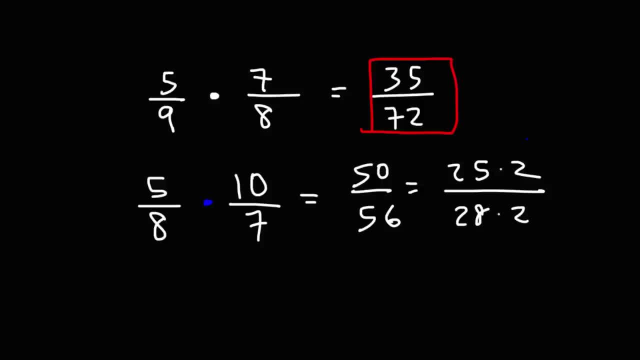 28 times 2.. If we cancel a 2, we're left with 25 over 28 for our final answer. Now what about this one? 12 over 27 times 18 over 30. Go ahead and try that problem. 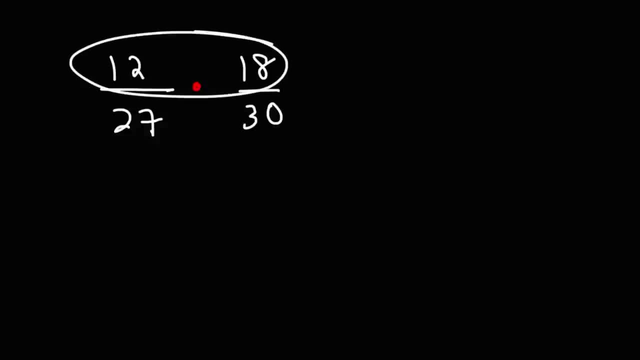 Now, if we multiply across 12 times 18 is going to give us a big number. 27 times 30, that's another big number as well, And then we'll have to reduce 2 big numbers. That's going to take a lot of work. 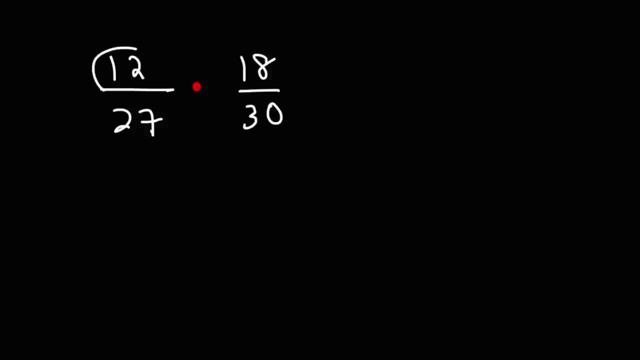 Instead, it's better if we reduce these numbers now before we multiply and create an even bigger number. 27: we can write that as 9 times 3.. 12: we can write that as 4 times 3.. 19 can be written as: 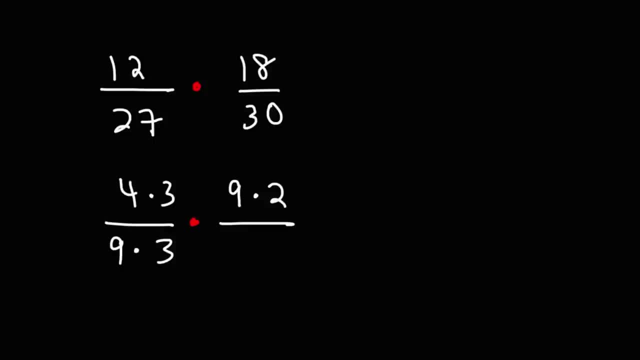 9 times 2.. So notice that we can cancel a 9 and we can cancel a 3.. 30- we can write that as 15 times 2.. So we can cancel a 2.. So all that's left is a 4 on top. 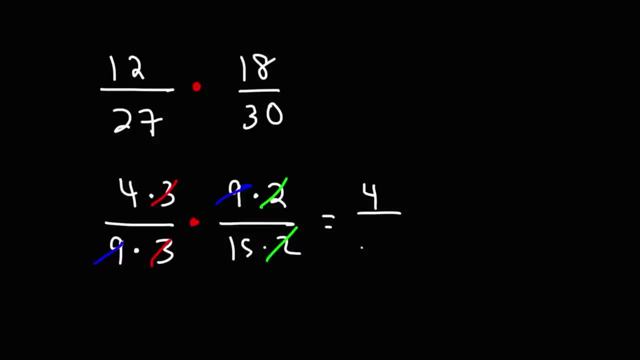 and a 15 on the bottom. So notice that in this problem we really didn't need to multiply by anything. All we need to do is break up these larger numbers into small numbers and cancel. So that's the answer: 4 over 15.. 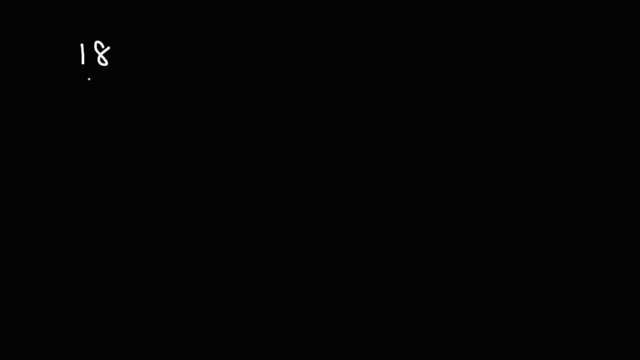 Let's work on another example. So let's say we have 18 divided by 45 times 40 over 42 times 35 over 24.. Go ahead and multiply those three fractions. So, once again, I recommend breaking down each fraction into smaller numbers. 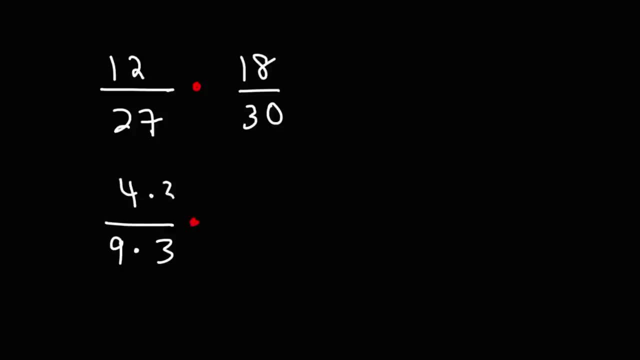 12, we can write that as 4 times 3.. 19 can be written as 9 times 2.. So notice that we can cancel a 9.. And we can cancel A 3.. 30,- we can write that as 15 times 2.. 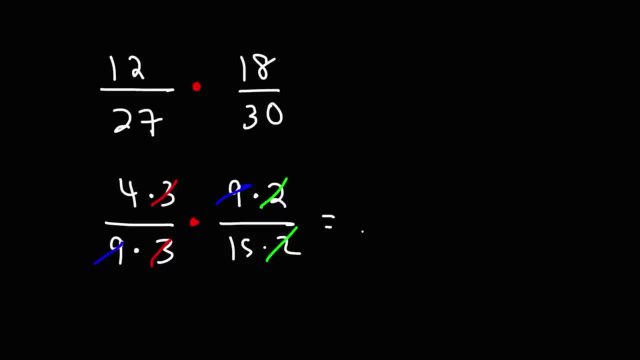 So we can cancel a 2.. So all that's left is a 4 on top and a 15 on the bottom. So notice that in this problem we really didn't need to multiply by anything. All we need to do is break up these larger numbers into smaller numbers and cancel. 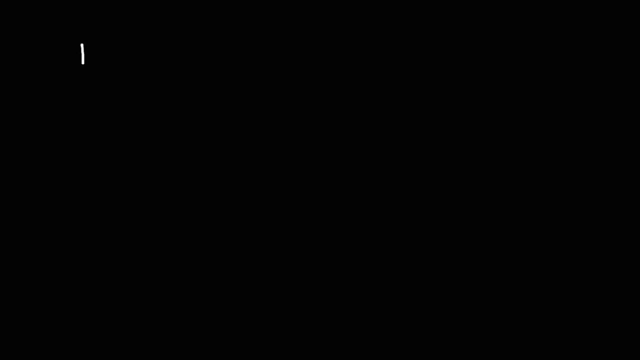 So that's the answer: 4 over 15.. Let's work on another example. So let's say we have 18 divided by 45 times 40 over 42 times 35 over 24.. Go ahead and multiply those three fractions. 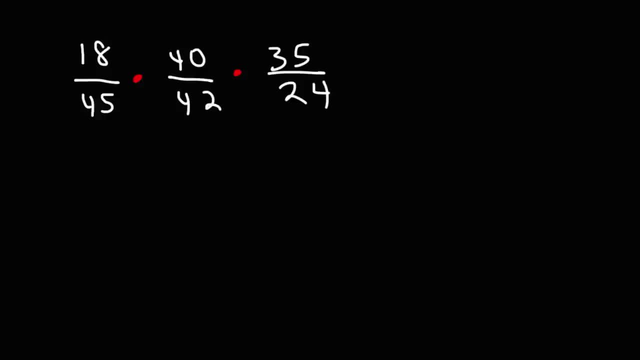 So, once again, I recommend breaking down each fraction into smaller numbers and cancel as much as you can before multiplying anything. So 45, we can write that as 9 times 5.. 18, we can write that as 9 times 2.. 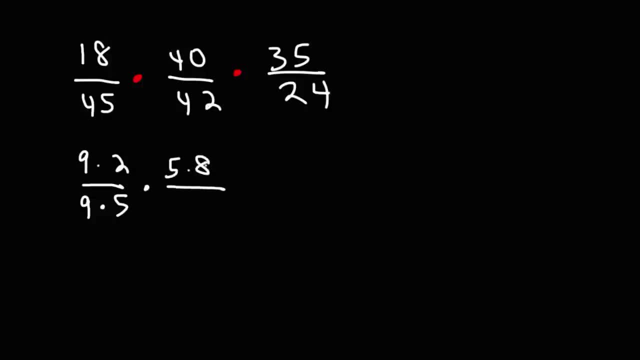 40, we can write 40 as 5 times 8. if we want to 42.. We can write that as 6 times 7.. 35 has a 7 in it. We can write that as 7 times 5.. 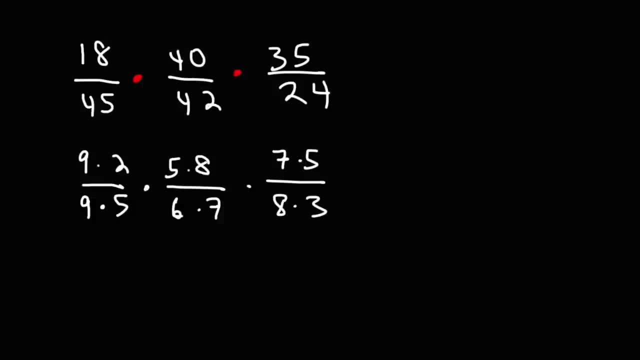 And 24 has an 8 in it, So we can write that as 8 times 3.. We can cancel an 8.. We can cancel a 7.. We can cancel a 5.. Let's put that in a different color. 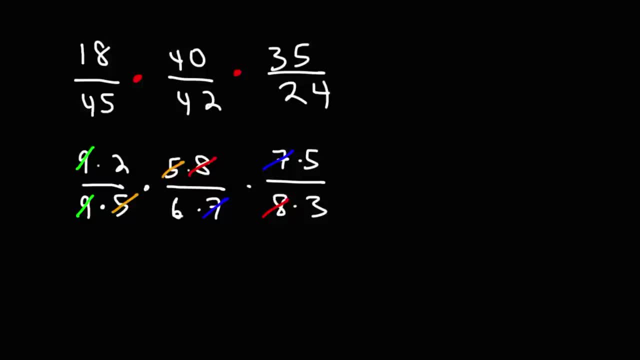 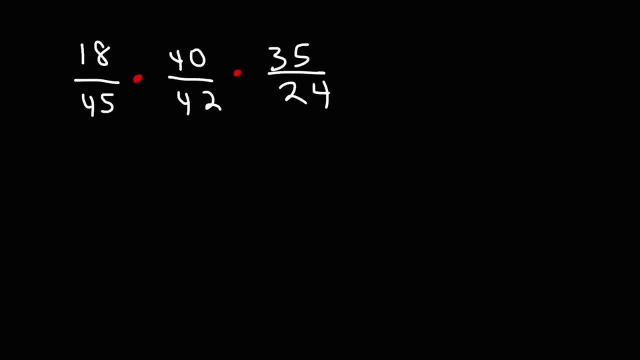 and cancel as much as you can before multiplying anything. So 45- we can write that as 9 times 5.. 18: we can write that as 9 times 2.. 40: we can write 40 as 5 times 8, if we want to. 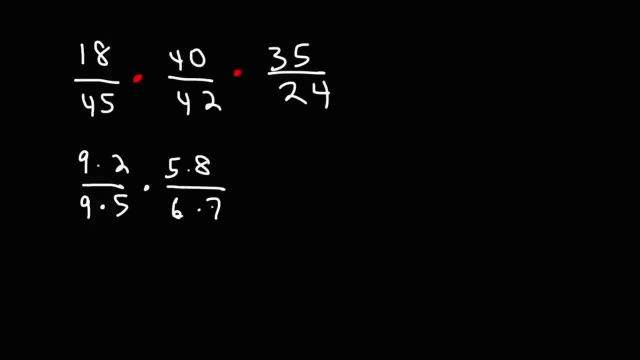 42, we can write that as 6 times 7.. 35 has a 7 in it. We can write that as 7 times 5.. And 24 has an 8 in it, So we can write that as 8 times 3.. We can cancel. 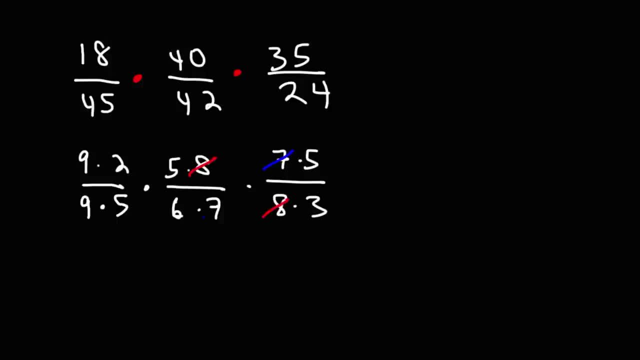 an 8.. We can cancel a 7.. We can cancel a 5.. Let's put that in a different color- And we can cancel a 9.. So right now we have 2 times 5, which is 10. And we have. 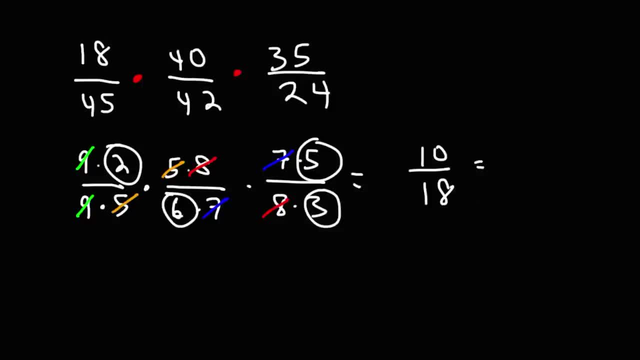 6 times 3, which is 18.. Now we can still reduce this further. 18: we can write that as 9 times 2.. 10: we can break that into 5 and 2.. So we can cancel the 2's. 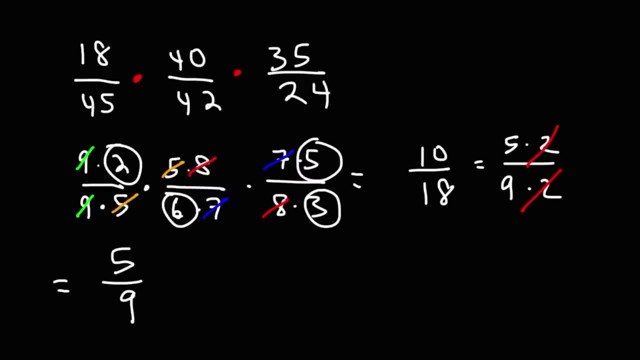 And thus we're left over with 5 over 9.. So that's the answer for this problem. Now let's talk about dividing two fractions. So let's say we have 15 over 40. And we wish to divide that by 35 over 56.. 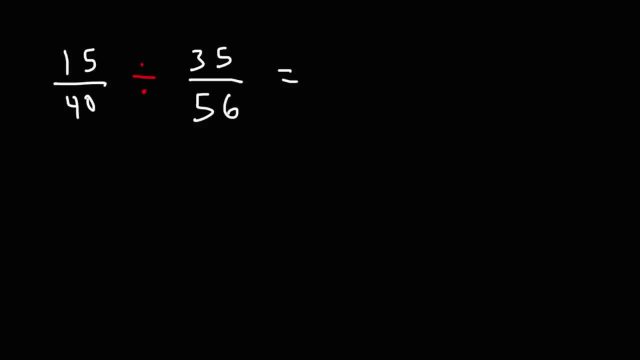 How can we do this? Perhaps you've heard of the expression keep, change flip. What it means is that you need to keep the first fraction, So we're going to keep it the same way. You need to change division to multiplication. 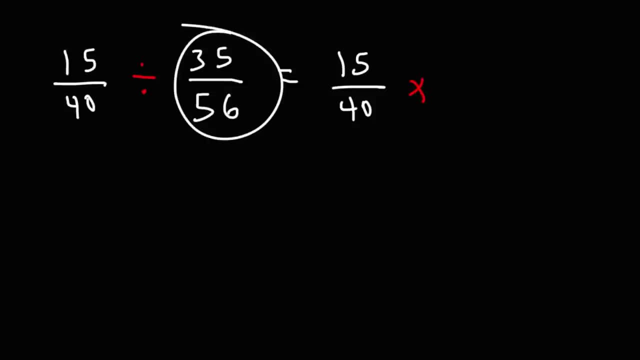 And then you need to flip the second fraction. So keep change and then flip this fraction. So now we converted a problem where we're dividing two fractions into one, where we're now multiplying two fractions. So let's break up these fractions into smaller numbers. 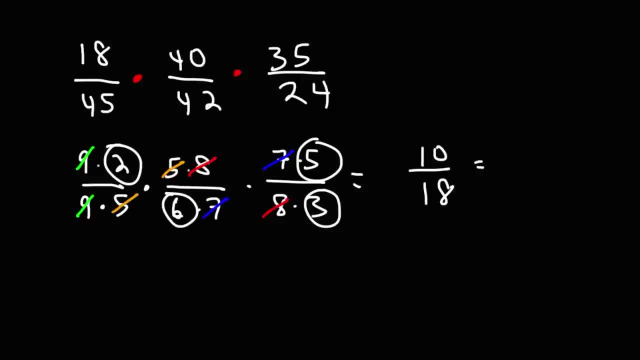 Now we can still reduce this further. 18, we can write that as 9 times 2.. 10, we can break that into 5 and 2. So we can cancel the 2's, and thus we're left over with 5 over 9.. 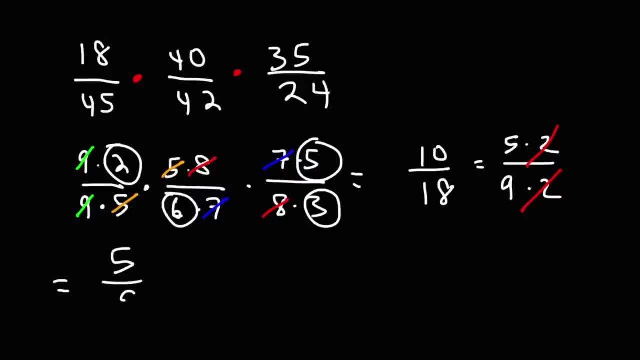 So that's the answer for this problem. Now let's talk about dividing. So let's look at this problem. So we can, if we want to struggled with dividing points, Yes, we can use mark tests for doing the multiplication algorithm. Yeah, and those b periods are: estoy, Michael, doesn't not delicious? 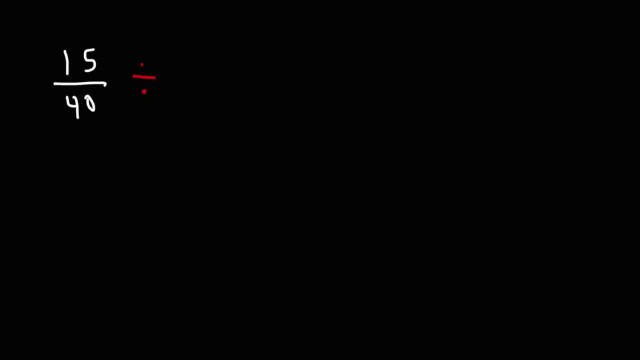 Not like me, Don't you? two fractions. So let's say we have 15 over 40, and we wish to divide that by 35 over 56. How can we do this? Perhaps you've heard of the expression keep change, flip What it means. 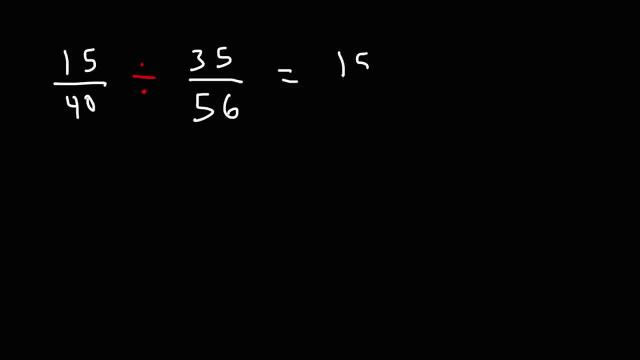 is that you need to keep the first fraction, So we're going to keep it. the same way, You need to change division to multiplication And then you need to flip the second fraction. So keep, change and then flip this fraction. So now we converted a problem where we're dividing two fractions into one, where we're 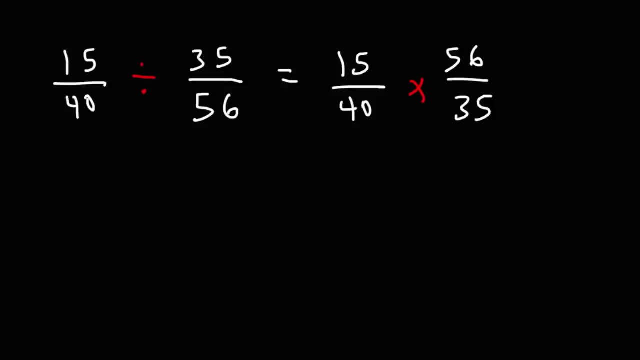 now multiplying two fractions. So let's break up these fractions into smaller numbers: 35, the only way we can break that up is in to seven and five: 56, we know that's seven times eight. 40 is eight times five. 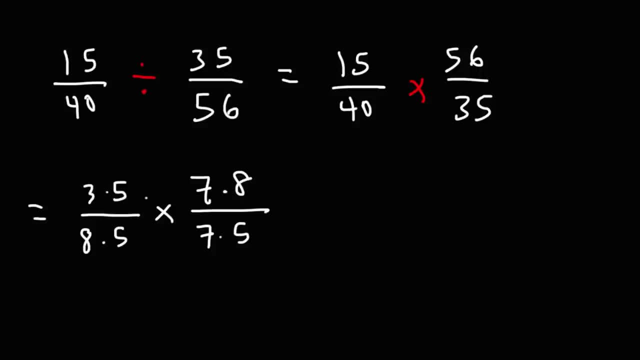 And 15 is five times three or three times five. So we can cross out an eight, We could cancel a seven And we can cancel a five. So we're left with three over five, And so that's it for this problem. 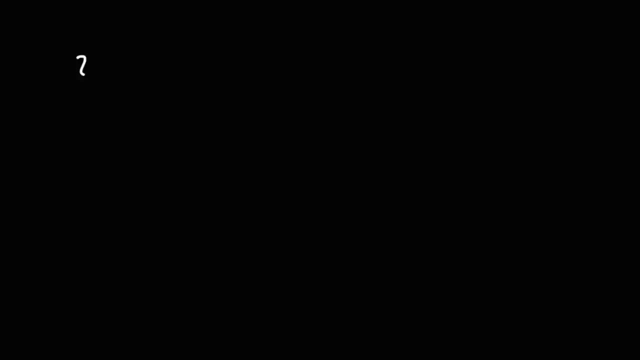 Now let's try another example. So let's say we have 28 over 24 divided by 35 over 32.. Go ahead and try that. So let's keep the first fraction the same, Let's change division to multiplication And then we're going to flip the second fraction. Keep, change, flip. 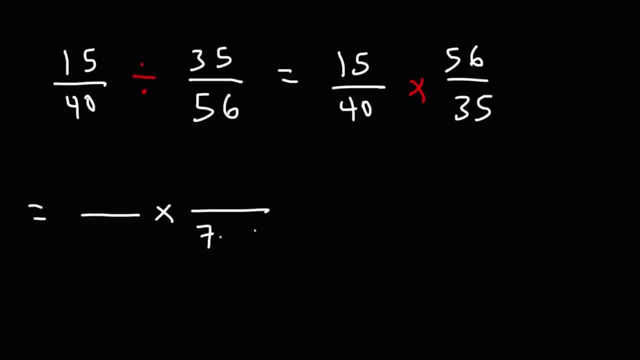 35, the only way we can break that up is into 7 and 5.. 56, we know that's 7 times 8.. 40 is 8 times 5.. And 15 is 5 times 3 or 3 times 5.. 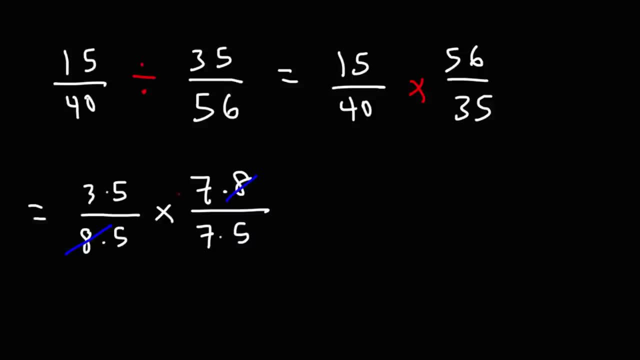 So we can cross out an 8.. We could cancel a 7. And we can cancel a 5.. So we're left with 3 over 5.. And so that's it for this problem. Now let's try another example. 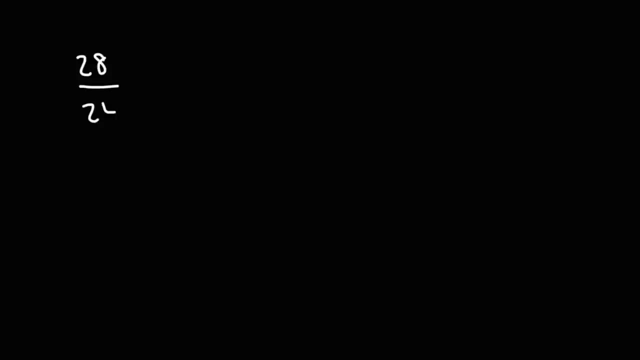 So let's say we have 28 over 24, divided by 35 over 32.. Go ahead and try that. So let's keep the first fraction the same, Let's change division to multiplication, And then we're going to flip the second. 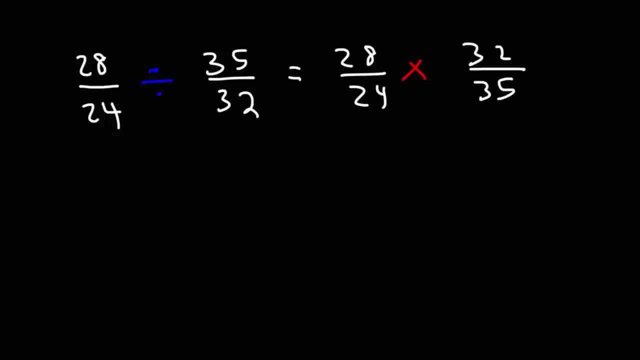 fraction. Keep change, flip. Now let's break up these fractions into small numbers. So 35,- that's the only option we have with that is 7 and 5.. 28 has a 7 in it, So we can write that as 7 times. 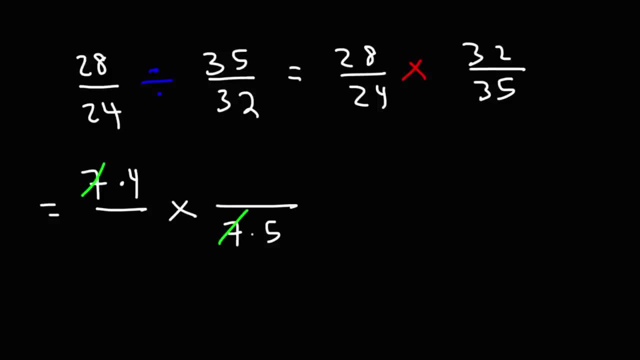 4. So the 7's will cancel, which is good. 24 has a 4 in it, So we can write that as 6 times 4.. Now 32,: we can write that as 8 times 4.. 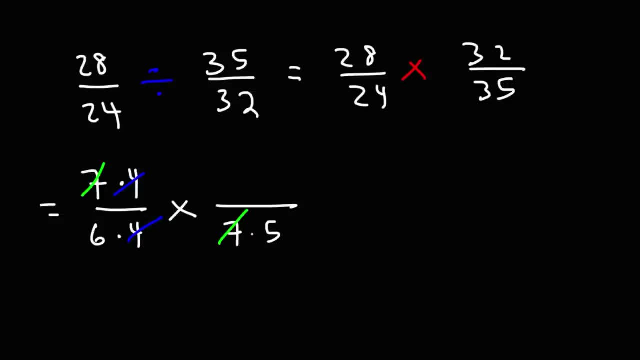 Or we can write that as 16 times 2.. For now let's leave it as 32.. On the bottom we have 6 and 5. So right now we have 32 over 30. 32 is 16 times 2.. 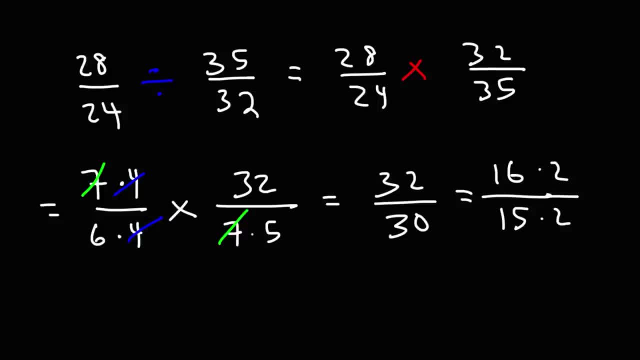 30 is 15 times 2.. So at least we can cancel the 2's, And so we're left with 16 over 15.. So that's the final answer, So that's what our original expression is equal to. Now what about this one? 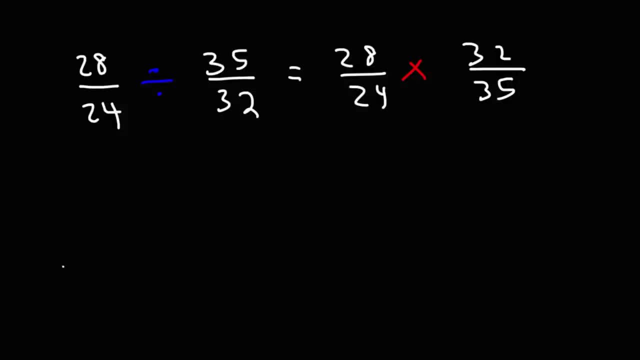 Now let's break up these fractions into small numbers. So 35,- that's the only option we have- of that is seven, and five, 28 has a seven in it, So we can write that as seven And then times four, So the sevens will cancel, which is good. 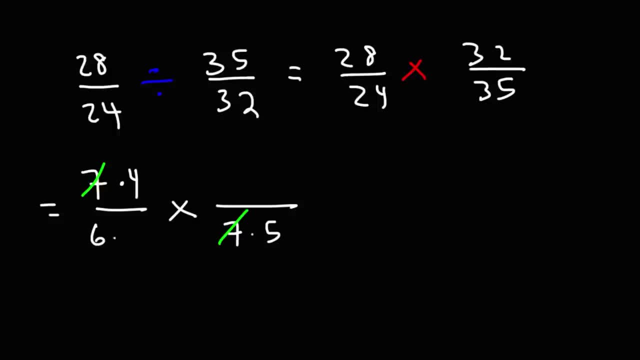 24 has a four in it, So we can write that as six times four, Now 32,. we can write that as eight times four, Or we can write that as 16 times two. For now let's leave it as 32.. On the bottom we have six and five. 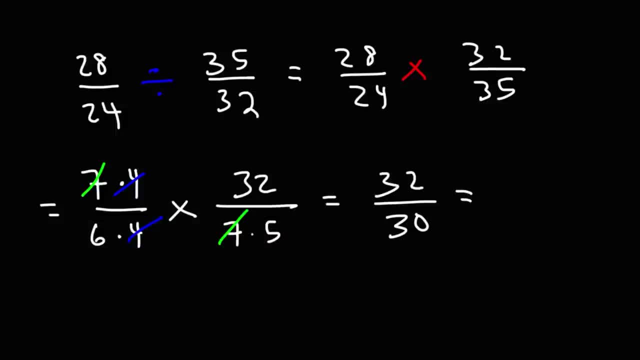 So right now we have 32.. 32 is 16 times two, 30 is 15 times two. So at least we can cancel the twos, And so we're left with 16 over 15.. So that's the final answer. 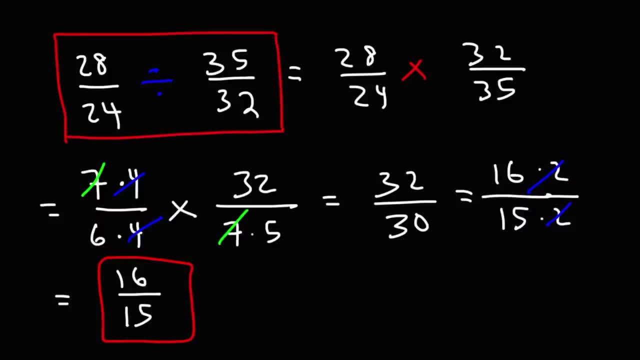 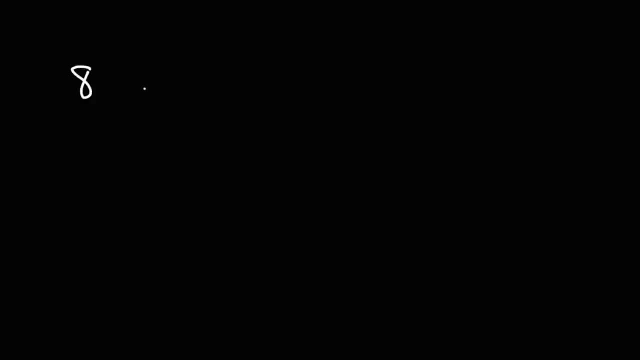 So that's what our original expression is equal to. Now what about this one? Let's say if we have a whole number And we wish to divide it by a fraction. So what is eight divided by three over four? How can we divide a whole number by a fraction? 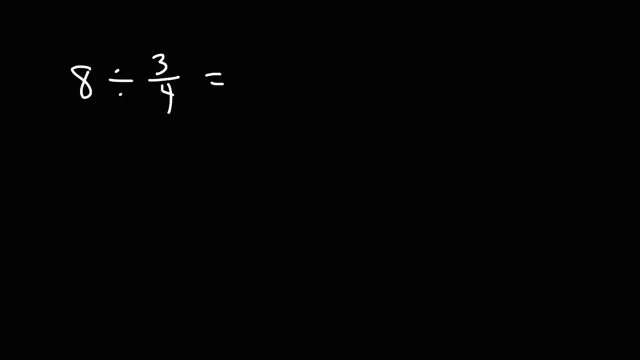 What we can do is we can turn the whole number into a fraction. Eight is the same as eight over one, So what we really have is eight over one divided by three over four, And now we can evaluate this the way we've been doing it before using keep change flip. 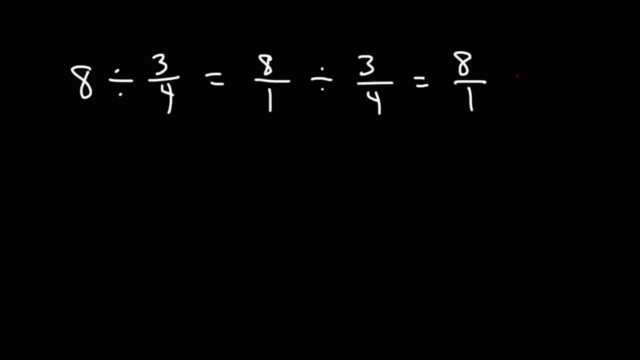 So let's keep the first, Let's keep the second fraction the same, Let's change division to multiplication, And then we're going to flip the second fraction, So now we can multiply across. So we have eight times four, which is 32.. 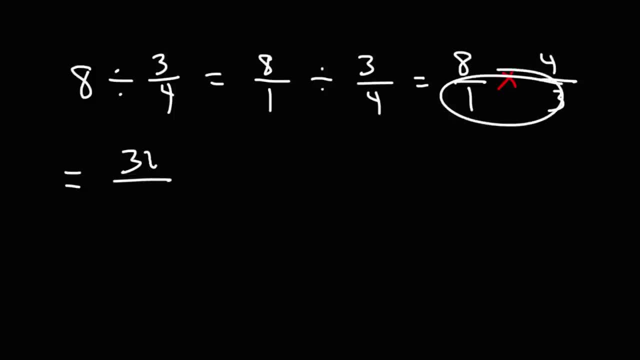 And on the bottom, one times three, which is three. So that's going to be the answer: It's 32 over three. Now, what about taking a fraction, let's say five over seven, And dividing it by three, And dividing it by a whole number? 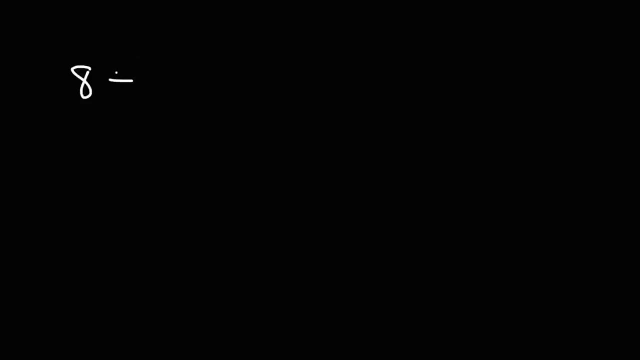 Let's say, if we have a whole number and we wish to divide it by a fraction. So what is 8 divided by 3 over 4?? How can we divide a whole number by a fraction? What we can do is we can turn the whole. 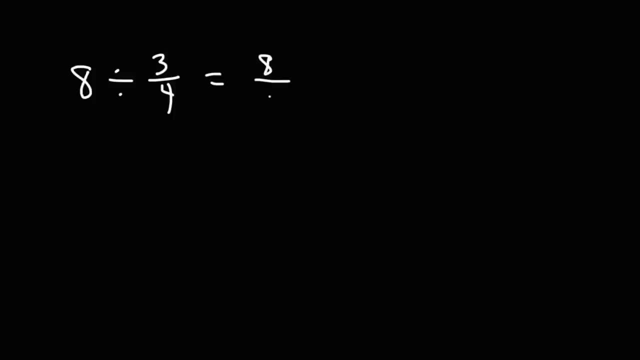 number into a fraction. 8 is the same as 8 over 1.. So what we really have is 8 over 1 divided by 3 over 4.. And now we can evaluate this the way we've been doing it before. 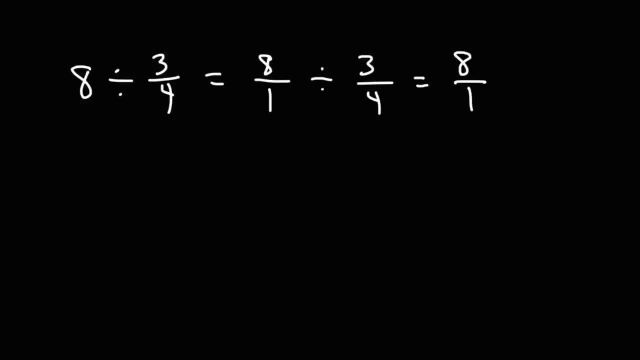 Using keep, change, flip. So let's keep the first fraction the same, Let's change division to multiplication, And then we're going to flip the second fraction, So now we can multiply across. So we have 8 times 4, which is 32.. 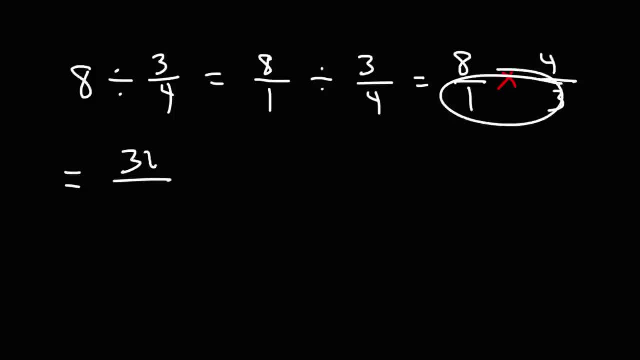 And on the bottom, 1 times 3, which is 3.. So that's going to be the answer: It's 32 over 3.. Now what about taking a fraction, let's say 5 over 7, and dividing it by a whole number? 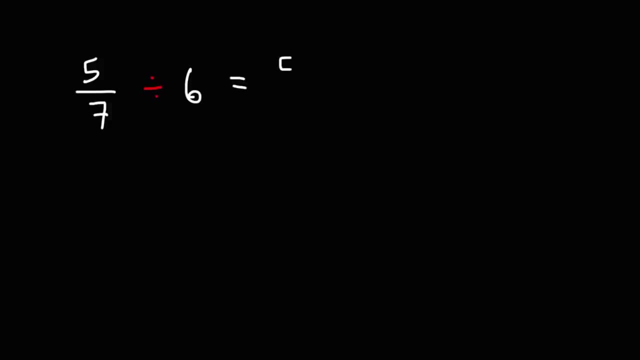 What's 5 over 7 divided by 6?? So we can rewrite 6 as a fraction, We can say it's 6 over 1.. And then using: keep, change flip. we'll keep the first fraction the same, We'll change. 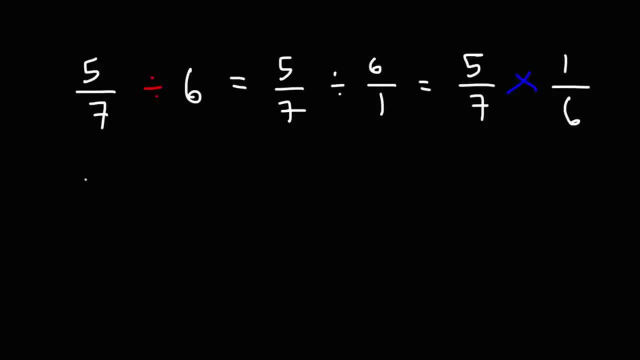 division to multiplication, And then we'll flip the second fraction, So it becomes 5 times 1, which is 5.. And 7 times 6, which is 42. So the answer is going to be 5 over 42.. Now what would you do if you saw? 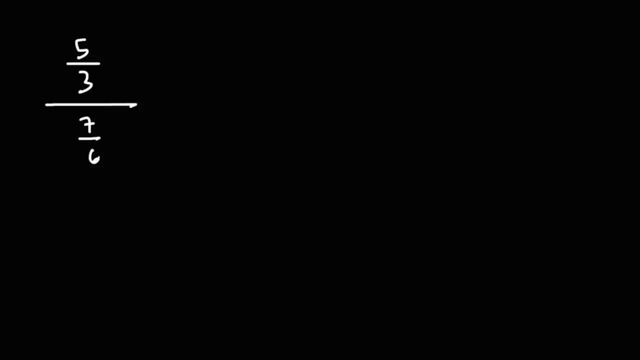 a fraction that looked like this: A complex fraction: 5 over 3, divided by 7 over 6.. How can we solve this one? What this really means is we're taking the first fraction, 5 over 3.. And then this: 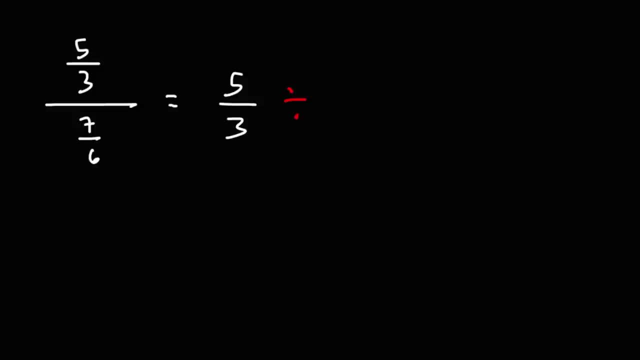 fraction here means division. We're dividing it by the second fraction, 7 over 6.. So it's another way to write this expression. So using keep change flip, we'll keep the first fraction the same, We'll change division to multiplication. 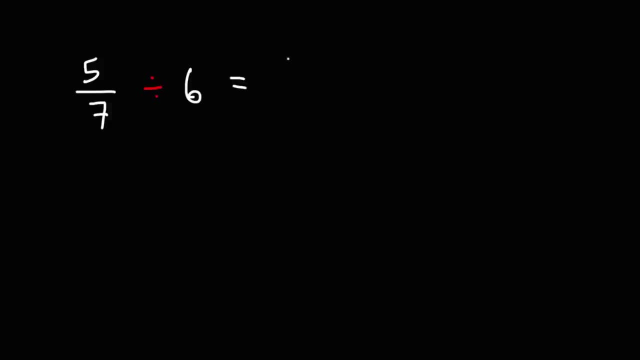 What's five over seven divided by six. So we can rewrite six as a fraction. We can say it's six over one And then using: keep, change, flip. we'll keep the first fraction the same, We'll change division to multiplication And then we'll flip the second fraction. 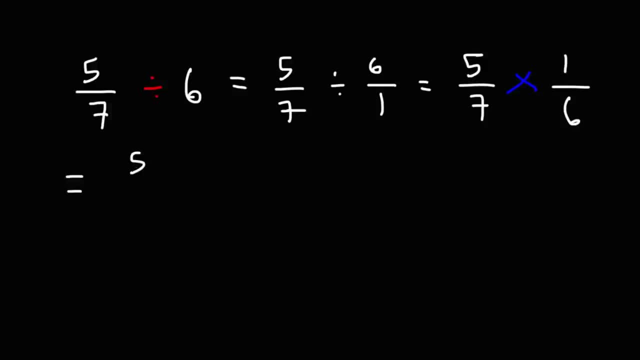 So it becomes five times one, which is five, And seven times six, which is 42.. So the answer is going to be five over 42.. Now what would you do if you saw a fraction that looked like this, A complex fraction? 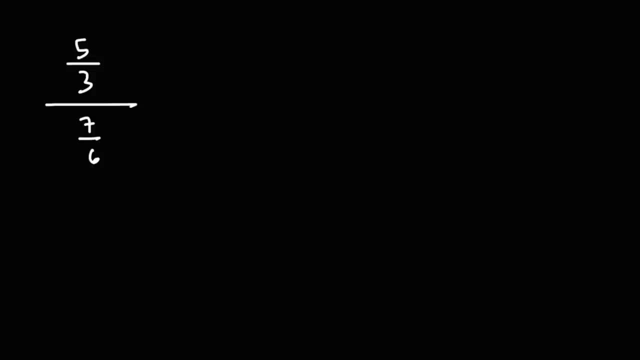 Five over three, divided by seven over six. How can we solve this one? What this really means is we're taking the first fraction, Five over three, And then this fraction here means division. We're dividing it by the second fraction, seven over six. 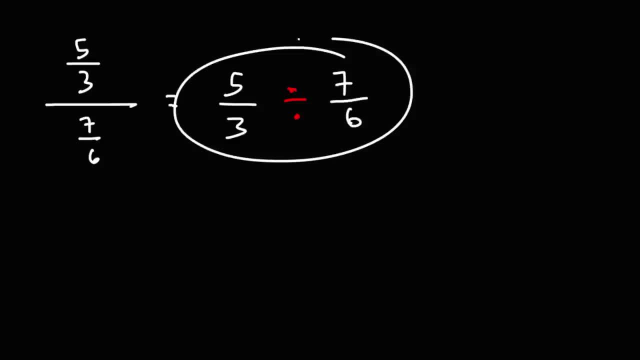 So it's another way to write this expression. So using: keep, change, flip. we'll keep the first fraction the same, We'll change division to multiplication And then we're going to flip the second fraction. So five and three. We can't really break that into small numbers. 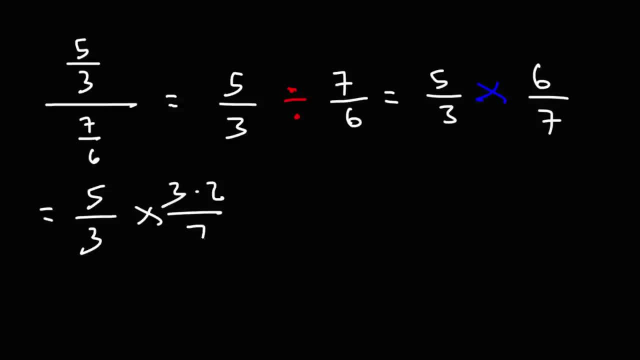 But six. We can break up six into three times two, So we can cancel the three, And then we'll be left with five times two, which is ten, And we only have a seven on the bottom. So this is the final answer. 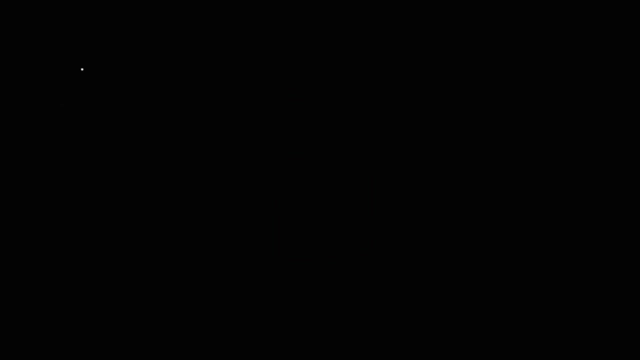 It's ten over seven. Now let's talk about how we can convert an improper fraction into a mixed number. An improper fraction is a fraction where the numerator is greater in value than the denominator. So seventeen over five is an improper fraction. How can we convert this into a mixed number? 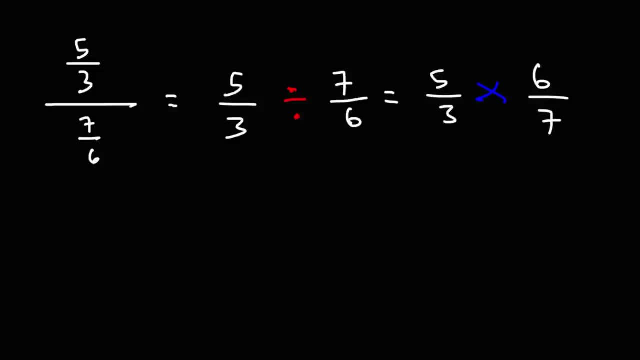 And then we're going to flip the second fraction, So 5 and 3. we can't really break that into small numbers, But 6. we can break up 6 into 3 times 2. So we can cancel with 3.. 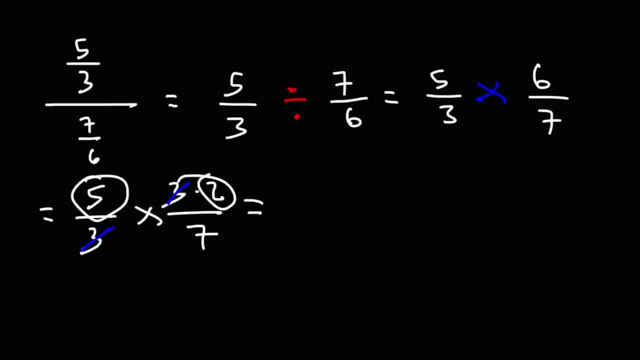 And then we'll be left with 5 times 2, which is 10.. And we only have a 7 on the bottom. So this is the final answer: It's 10 over 7.. Now let's talk about how we can convert an improper. 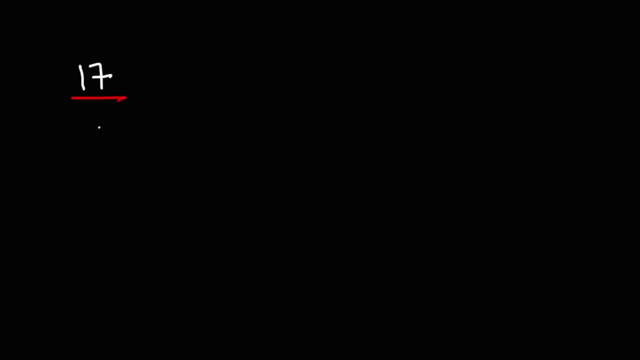 fraction into a mixed number. An improper fraction is a fraction where the numerator is greater in value than the denominator. So 17 over 5 is an improper fraction. How can we convert this into a mixed number? So here's how you can do it mentally. 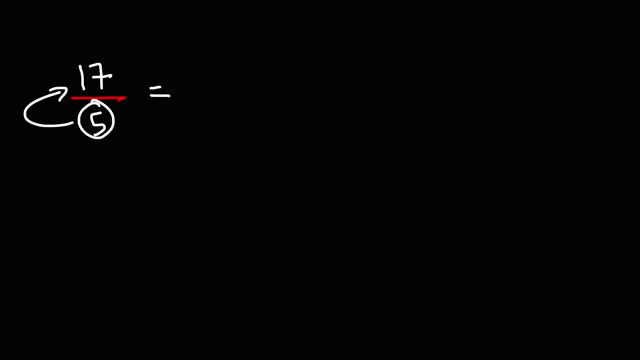 How many times does 5 go into 17?? 5 goes into 17 three times. The denominator is not going to change. 5 times 3 is 15.. And 17 minus 15 is 2.. So the remainder is 2.. 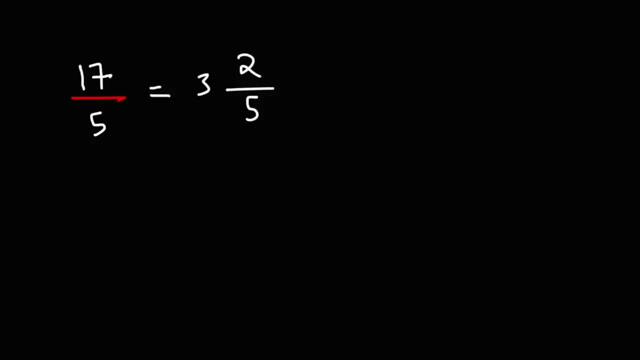 Thus, 17 over 5 is 3 and 2 fifths as a mixed number. Let's try another example: 29 over 7.. How many times does 7 go into 29? 7 goes into 29 four times. 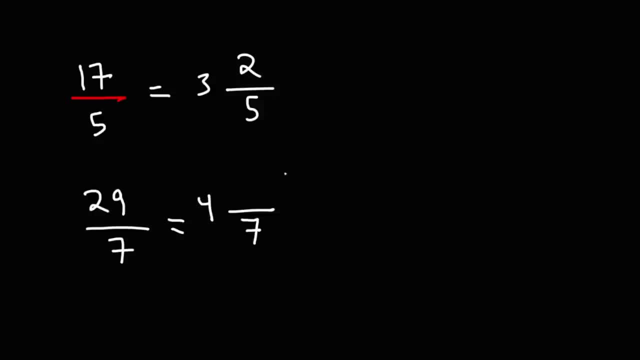 4 times 7 is 28.. 29 minus 28 is 1.. So the answer is 4 and 1, seventh as a mixed number. So that's how you can do it mentally For those of you who want to show your work. 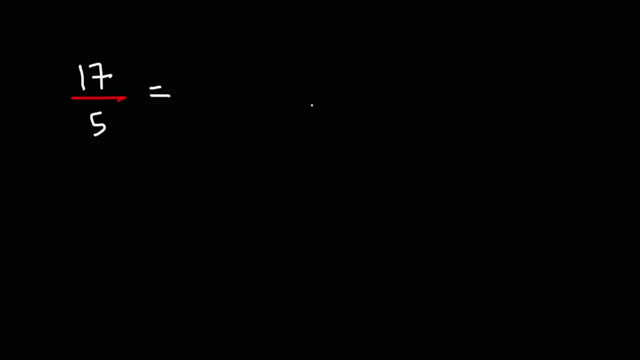 here's what you can do: 17 over 5. we can break that into 15 over 5 and 2 over 5.. The reason why I chose 15 is because 5 goes into 15 evenly. 15 over 5 is 3. 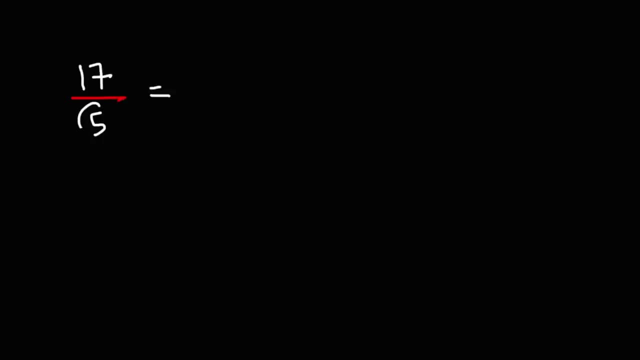 So here's how you can do it mentally: How many times does five go into seventeen? Five goes into seventeen three times. The denominator is not going to change. Five times three is fifteen, And seventeen minus fifteen is two, So the remainder is two. 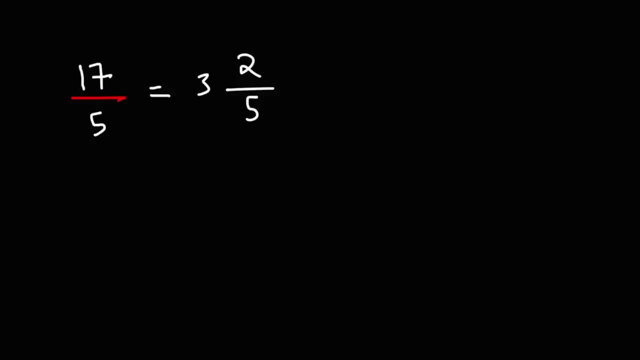 Thus, seventeen over five is three and two-fifths as a mixed number. Let's try another example: Twenty-nine over seven. How many times does seven go into twenty-nine? Seven goes into twenty-nine four times. Four times seven is twenty-eight. 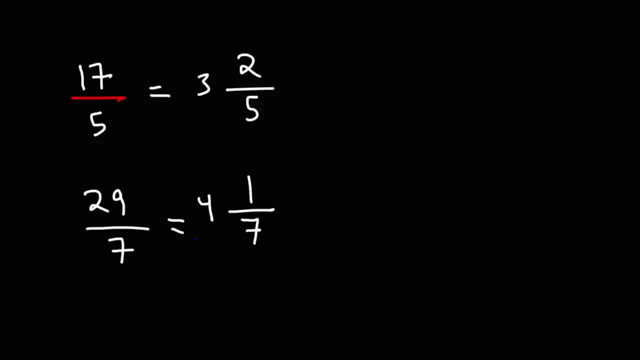 Twenty-nine minus twenty-eight is one, So the answer is four and one-seventh as a mixed number. So that's how you can do it mentally. For those of you who want to show your work, here's what you can do: Seventeen over five. we can break that into fifteen over five and two over five. 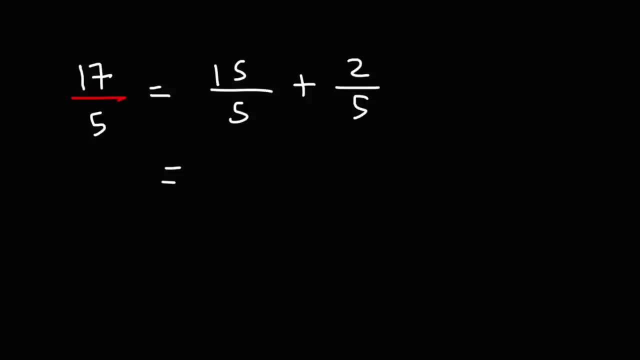 The reason why I chose fifteen is because five goes into fifteen evenly. Fifteen over five is three, And then we have three plus two over five, which is three and two-fifths as a mixed number. So that's a quick way to show your work. 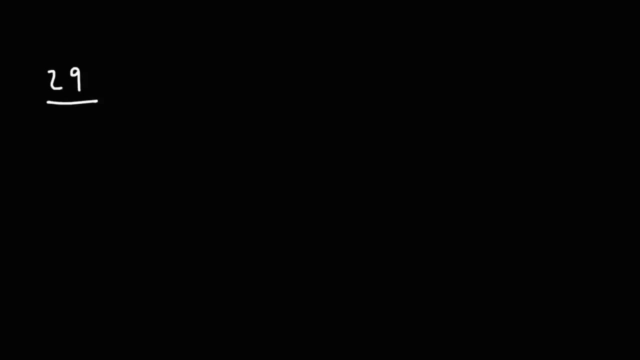 For the other one, where we had twenty-nine over seven, we can write that as twenty-eight over seven plus one over seven, Twenty-nine is twenty-eight plus one. Twenty-eight divided by seven is four. So we get four plus one over seven, which is four and one-sevenths. 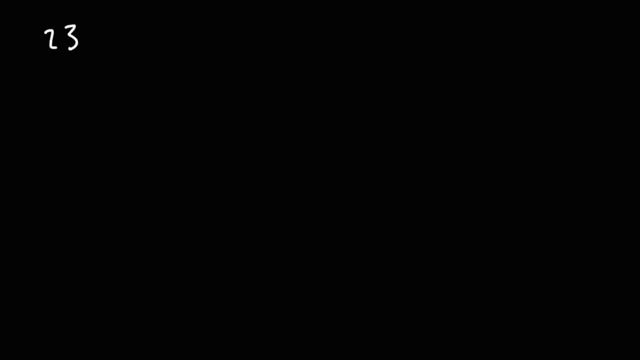 Go ahead and try these examples. Convert these fractions into mixed numbers: Twenty-three over five, Try fourteen over nine And also twenty-eight over six. So for the first one I would break up twenty-three into twenty and three Five goes into twenty. 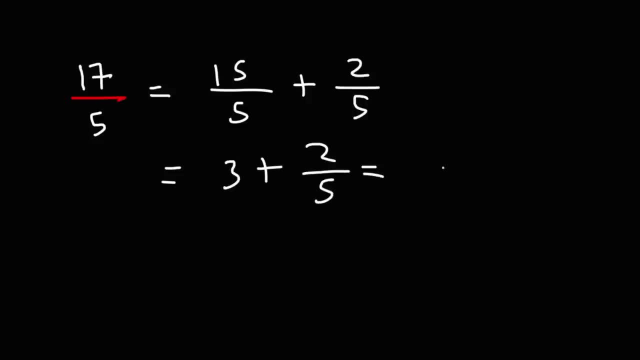 and then we have 3 plus 2 over 5, which is 3 and 2 fifths as a mixed number. So that's a quick way to show your work. For the other one, where we had 29 over 7, we can write: 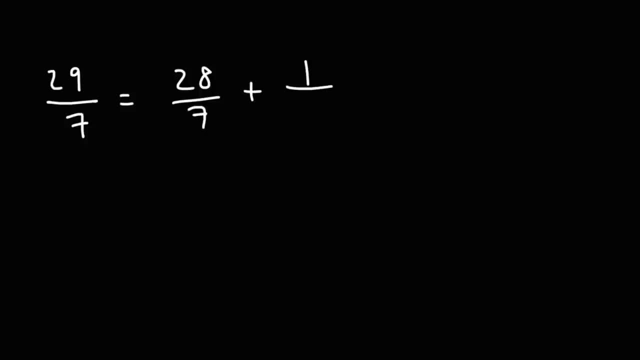 that, as 28 over 7 plus 1 over 7.. 29 is 28 plus 1.. 28 divided by 7 is 4.. So we get 4 plus 1 over 7, which is 4 plus 1. sevenths, 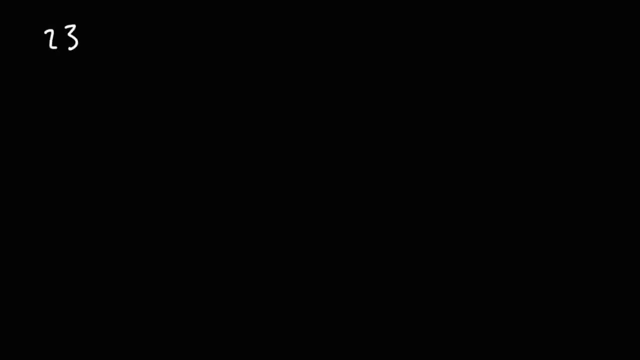 Go ahead and try these examples. Convert these fractions into mixed numbers: 23 over 5, Try 14 over 9 and also 28 over 6. So for the first one, I would break up 23 into 20 and 3.. 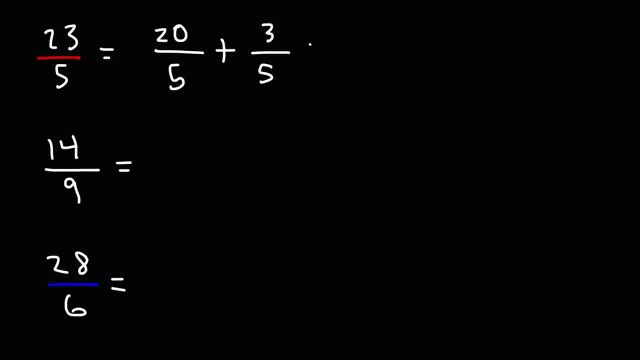 5 goes into 20.. 20 divided by 5 is 4.. So we get 4 plus 3 over 5.. So we can write that as 4 and 3. fifths, 14 over 9. we can write that as 9 over 9. 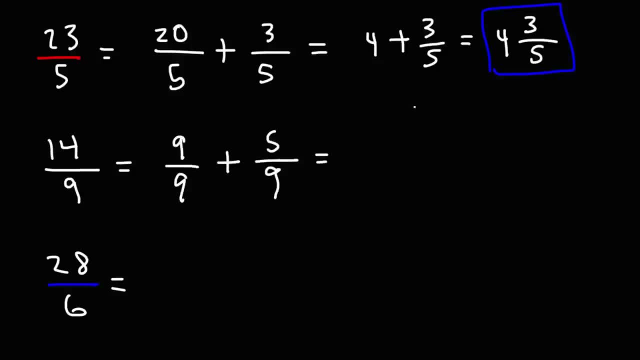 plus 5 over 9.. 9 over 9 is 1., And so this becomes 1 and 5 ninths. Now how can we break up 28?? What I would do is I would choose the highest multiple of 6. 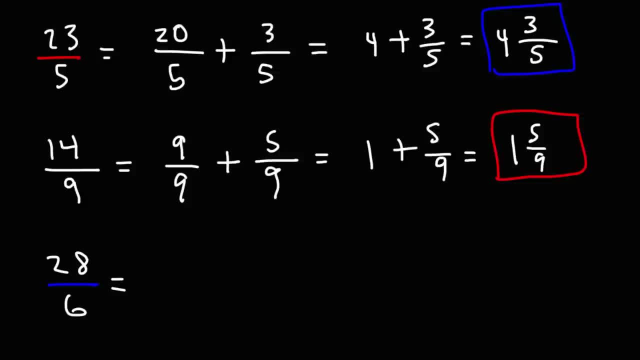 just under 28.. Multiples of 6 are 6,, 12,, 18, and 24.. 30 is too high, So we have 24, and then 28 minus 24 is 4.. So I would break up 28 as 4.. 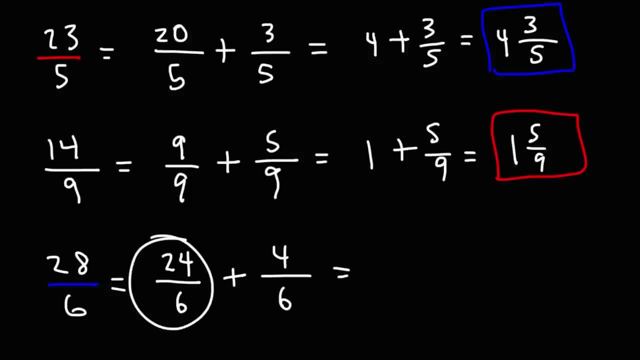 8 into 24 plus 4.. 24 divided by 6 is 4. And 4 over 6. we could simplify that fraction: 4 is 2 times 2.. 6 is 3 times 2.. So we can cancel. 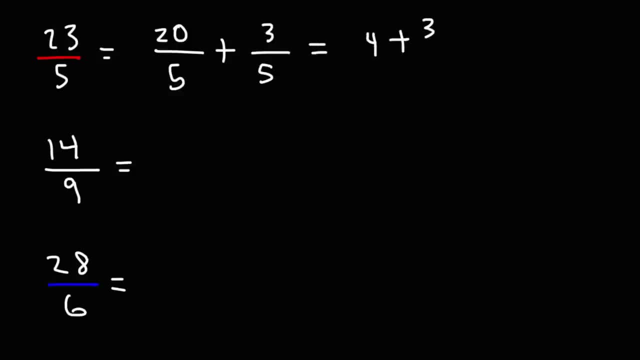 Twenty divided by five is four, So we get four plus three over five, So we can write that as four and three-fifths, Fourteen over nine. We can write that as nine over nine plus five over nine. Nine over nine is one. 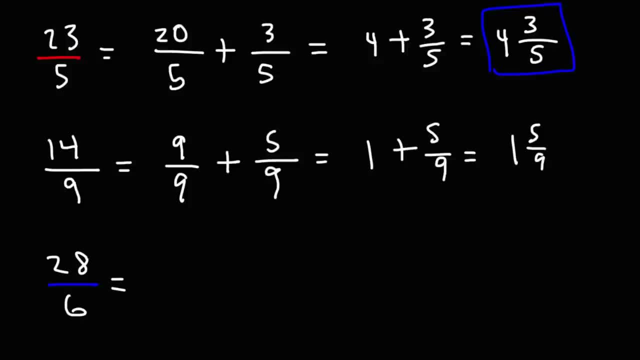 And so this becomes one and five-nines. Now how can we break up twenty-eight? What I would do is I would choose the highest multiple of six. just under twenty-eight Multiples of six are six, twelve, eighteen and twenty-four. 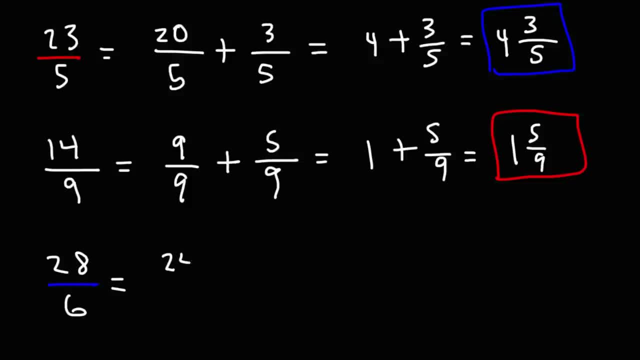 Thirty is too high, So we have twenty-four. And then twenty-eight minus twenty-four is four, So I would break up twenty-eight into twenty-four plus four. Twenty-four divided by six is four, And four over six. we could simplify that fraction. 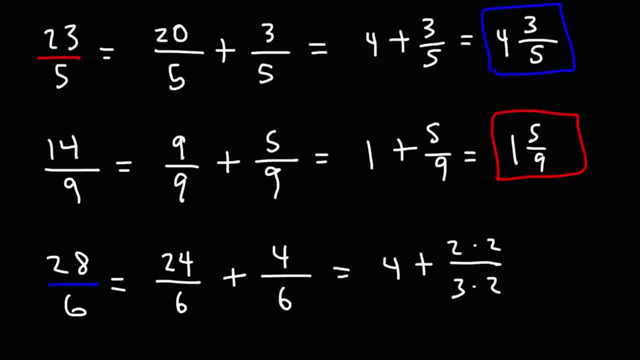 Four is two times two, Six is three times two, So we can cancel a two, And so we're left with four plus two over three. Thus, the final answer is four and two-thirds. So now you know how to convert an improper fraction into a mixed number. 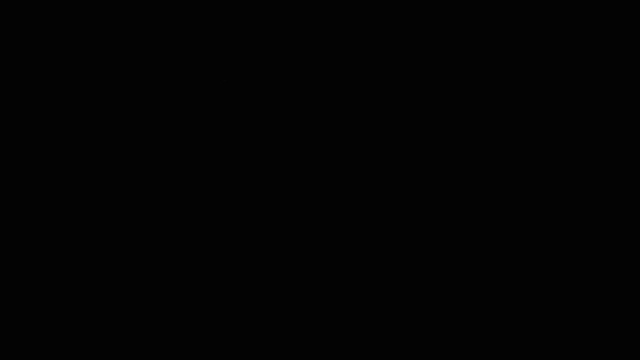 Now what about going the other way? What if we had a mixed number? How can we convert the mixed number into an improper fraction? So first rewrite the denominator, Next multiply these two numbers. Three times three is nine, And then add the numerator. 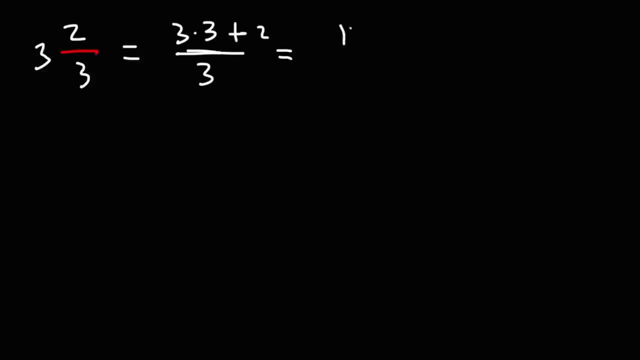 So we got three times three is nine plus two is eleven. The answer is going to be eleven over three. Try this one: Convert five and one-fourths into an improper fraction, So it's going to be five times four, which is twenty plus one. 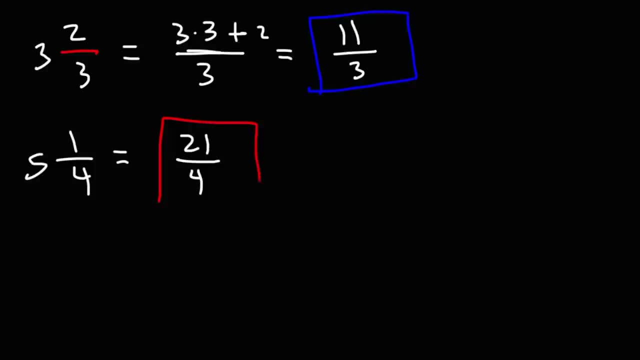 So that's going to be twenty-one over four. Try these two, Seven and three-eighths, And then two and four-fifths. So first let's write the eight, And then it's seven times eight, which is fifty-six plus three. 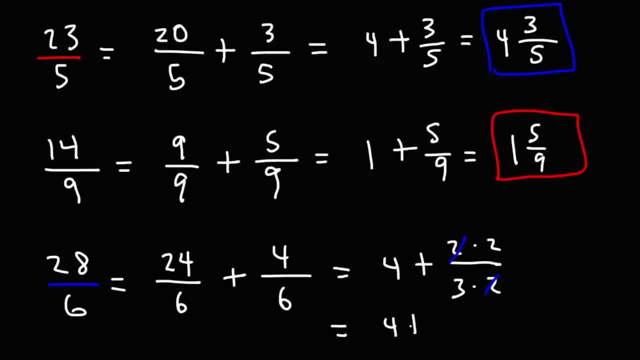 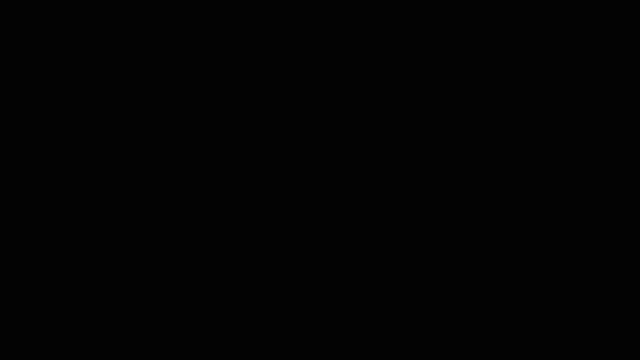 a 2.. And so we're left with 4 plus 2 over 3.. Thus, the final answer is 4 and 2 thirds. So now you know how to convert an improper fraction into a mixed number. Now what about going the other way? 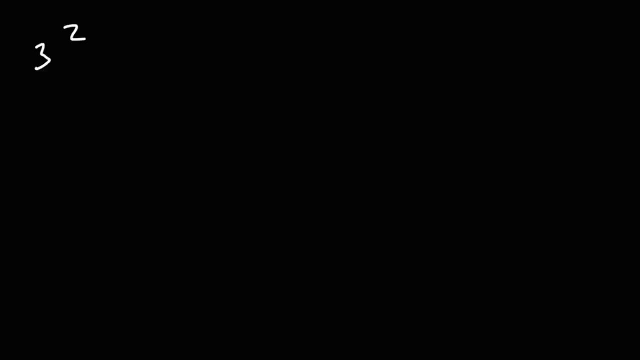 What if we had a mixed number? How can we convert the mixed number into an improper fraction? So first rewrite the denominator, Next multiply these two numbers. 3 times 3 is 9 and then add the numerator. So we got 3 times 3 is. 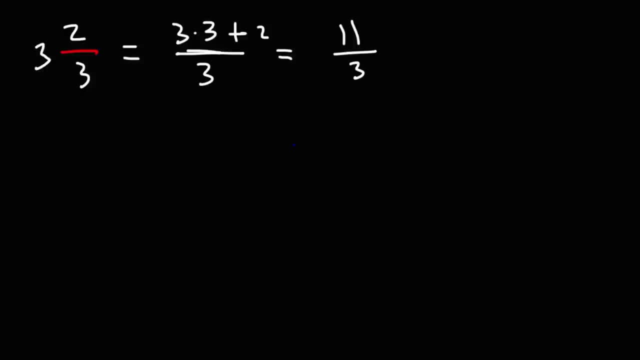 9 plus 2 is 11.. The answer is going to be 11 over 3.. Try this one. Convert 5 and 1 fourths into an improper fraction. So it's going to be 5 times 4, which is 20 plus 1.. 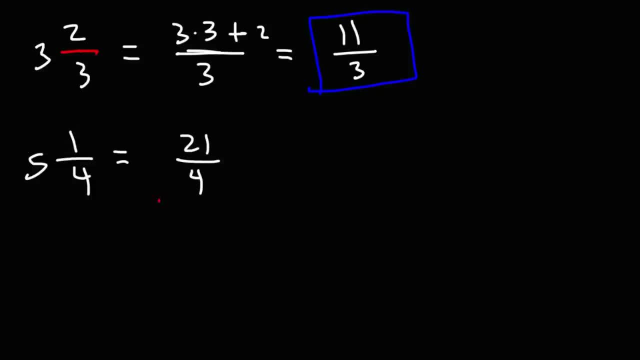 So that's going to be 21 over 4.. Try these two, 7 and 3 eighths, and then 2 and 4 fifths. So first let's write the 8 and then it's 7 times 8. 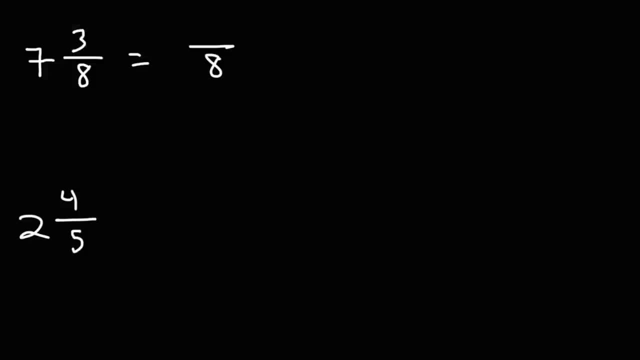 which is 56 plus 3, and that's going to be 59.. For the next one, let's rewrite the 5.. 2 times 5 is 10 plus 4, that's 14.. That's going to be 14 over 5.. 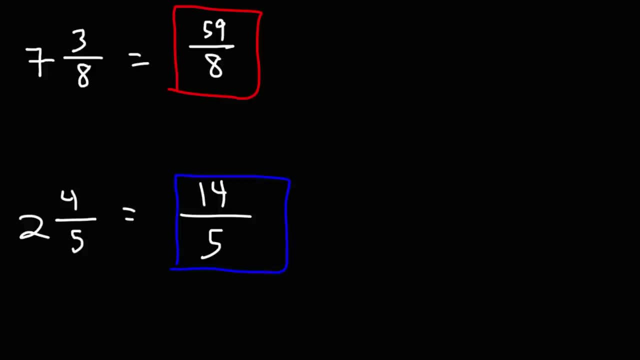 So that's how you can convert a mixed number back into an improper fraction. Now, how can we add two mixed numbers? So let's say, if we have 3 and 1 fourth plus 5 and 2 thirds, How can we add these two? 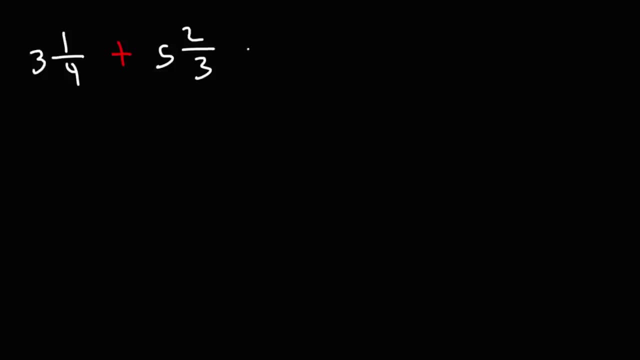 mixed numbers. Well, first let's rewrite it: 3 and 1. fourth, we know it's 3 plus 1 over 4.. 5 and 2 thirds is 5 plus 2 over 3.. So we can add 3 and 5 together and we're going to. 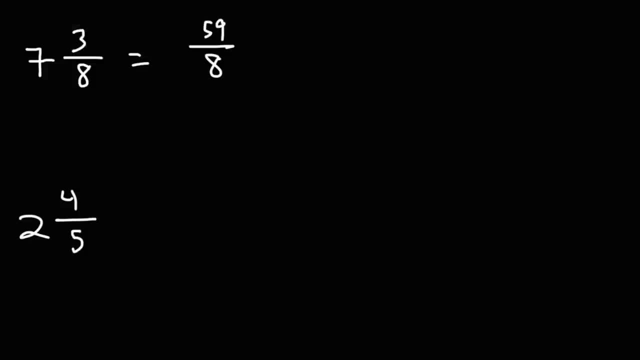 And that's going to be fifty-nine. For the next one, let's rewrite the five. Two times five is ten plus four, That's fourteen. So it's going to be fourteen over five. So that's how you can convert a mixed number back into an improper fraction. 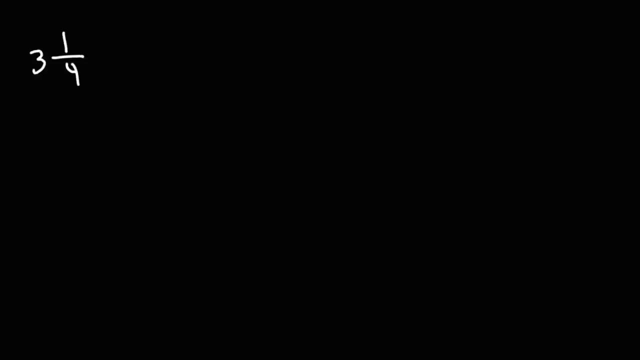 Now, how can we add two mixed numbers? So let's say, if we have three and one-fourth plus five and two-thirds, How can we add these two mixed numbers? Well, first let's rewrite it: Three and one-fourth. we know it's three plus one over four. 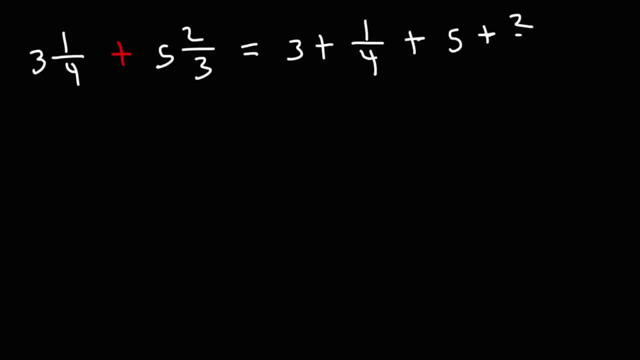 Five and two-thirds is five plus two over three, So we can add three and five together and we're going to get eight, And then we have eight plus one over four, plus two over three. Now what we need to do is we need to add those two fractions together. 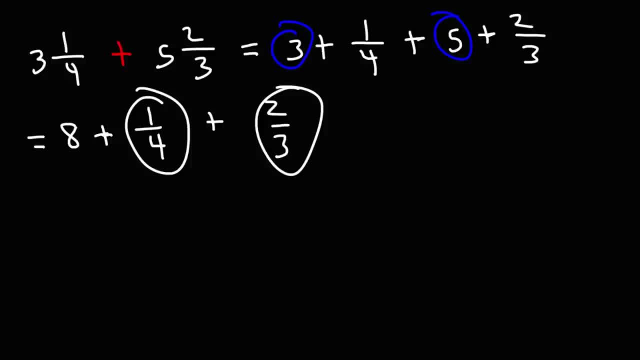 And in order to do that we have to get common denominators. So we're going to multiply this one by three over three and this fraction by the other denominator, four over four. So we have eight, and then plus One times three is three. 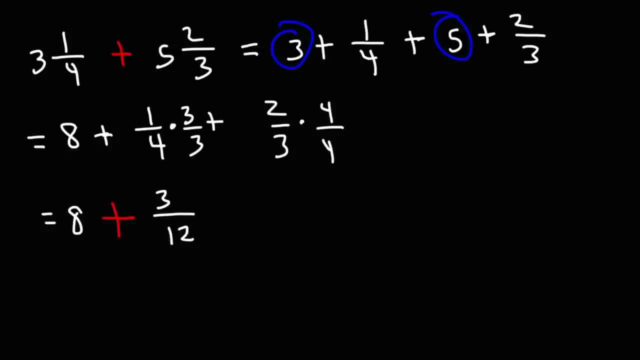 Four times three is twelve, And here we have two times four, which is eight over three times four, which is twelve. Three over twelve plus eight over twelve is eleven over twelve. So thus we have eight plus eleven over twelve. Thus we can write the final answer as eight and eleven twelves. 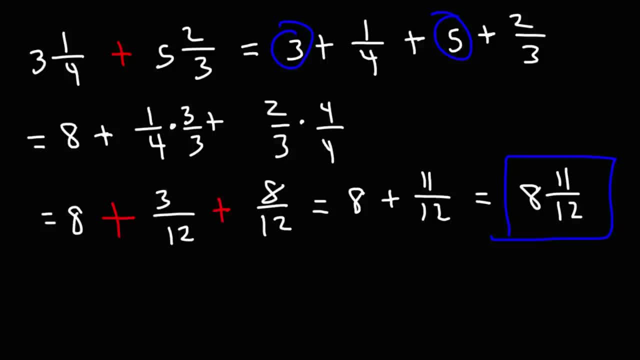 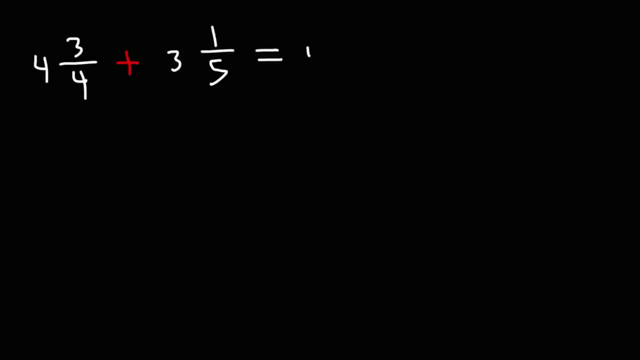 So that's how we can add two mixed numbers together. Try this: one, Four and three-fourths plus three and one-fifths. Feel free to pause the video. Go ahead and add those two mixed numbers together. So first let's rewrite the problem. 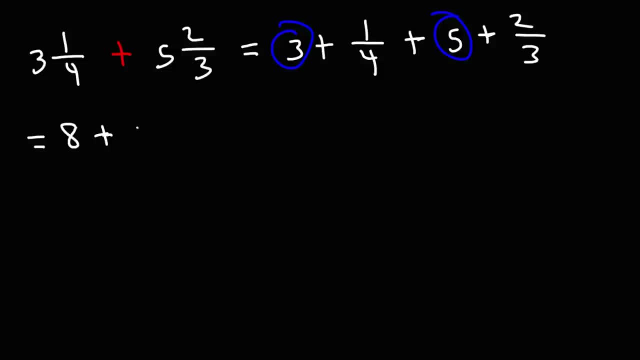 get 8.. And then we have 8 plus 1 over 4 plus 2 over 3.. Now what we need to do is we need to add those two fractions together, And in order to do that, we have to get common. 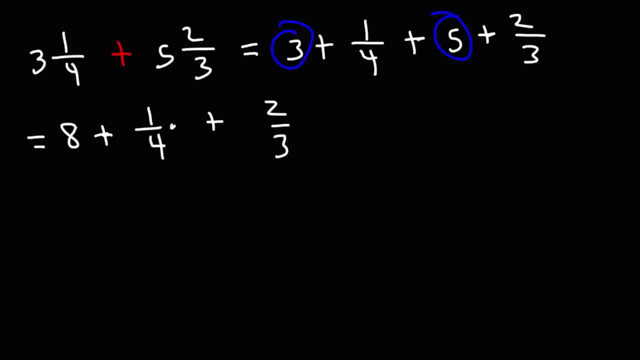 denominators. So we're going to multiply this one by 3 over 3 and this fraction by the other denominator, 4 over 4.. So we have 8, and then plus 1 times 3 is 3, 4 times 3. 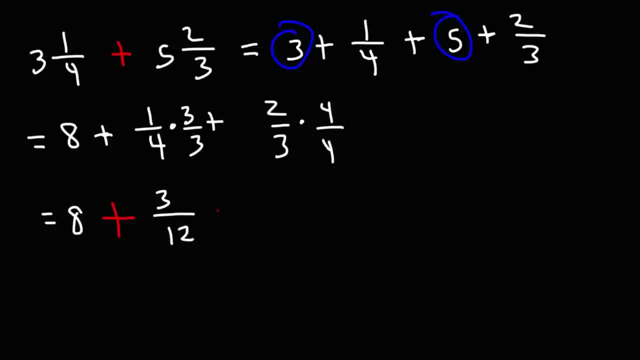 is 12.. And here we have 2 times 4, which is 8 over 3 times 4, which is 12.. 3 over 12 plus 8 over 12 is 11 over 12.. So thus we have 8 plus 11. 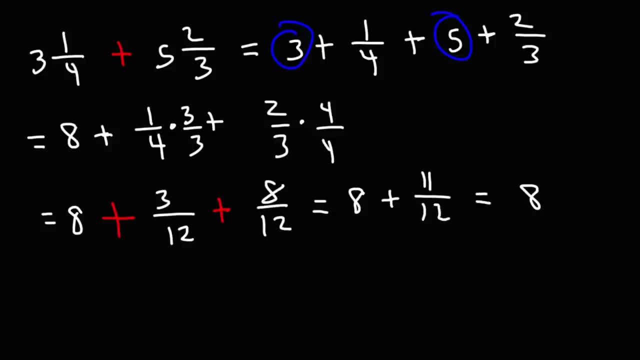 over 12.. Thus we can write the final answer as 8 and 11 twelfths. So that's how we can add two mixed numbers together. Try this: one, 4 and 3 fourths plus 3 and one fifths. 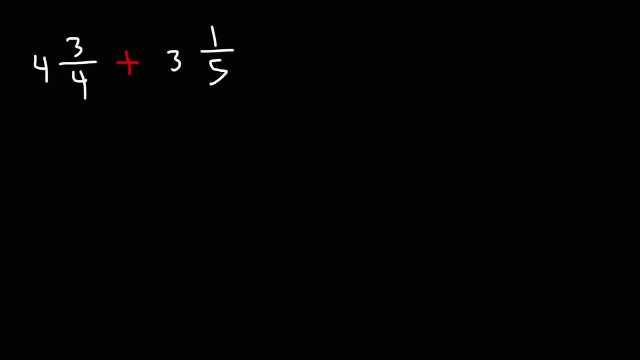 Feel free to pause the video. Go ahead and add those two mixed numbers together. So first let's rewrite the problem. 4 and 3. fourths is 4 plus 3 over 4.. 3 and one. fifths is 3. 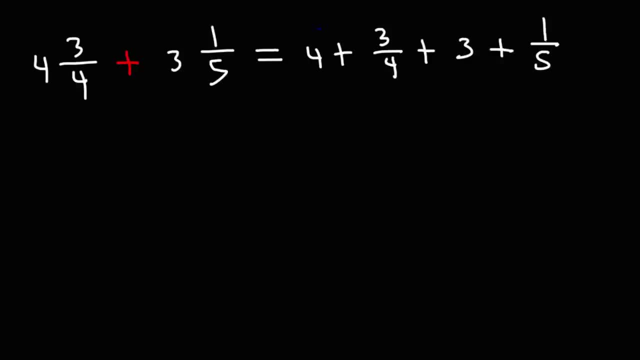 plus 1 over 5.. So now let's combine the whole numbers: 4 plus 3 is 7.. And then we have 3 over 4.. And then plus 1 over 5.. So 3 fourths. let's multiply by using. 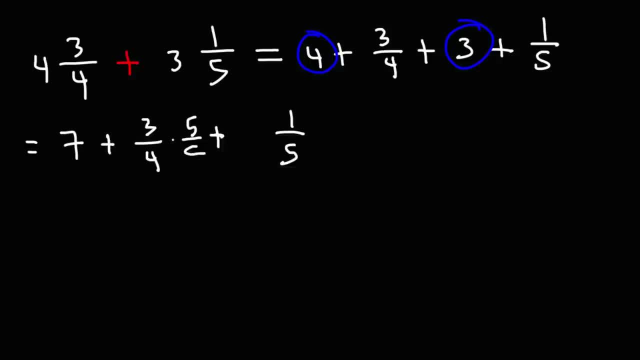 the 5.. So we're going to multiply 3 fourths by 5 over 5.. And we're going to multiply 1 over 5 by the other denominator, 4.. So times 4 over 4.. So this is going to be 7 plus. 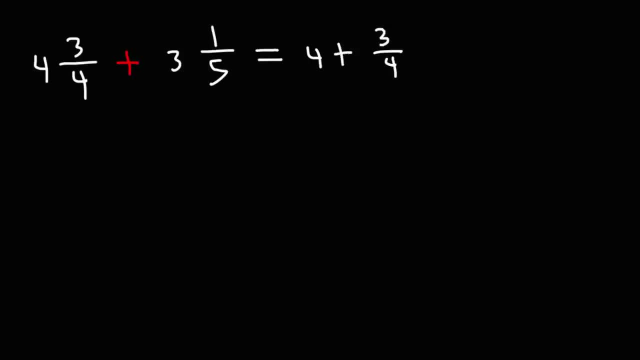 Four and three-fourths is four plus three over four. Three and one-fifths is three plus one over five. So now let's combine the whole numbers. Four plus three is seven, And then we have plus three over four, And then plus one over five. 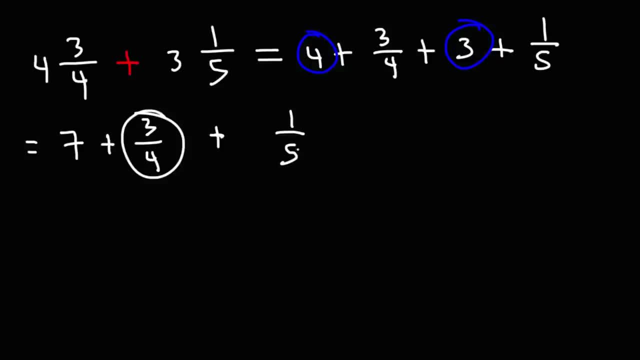 So three-fourths. let's multiply by using the five. So we're going to multiply three-fourths by five over five, And we're going to multiply one over fifth by the other denominator, four. So times four over four. So this is going to be seven plus three times five is fifteen. 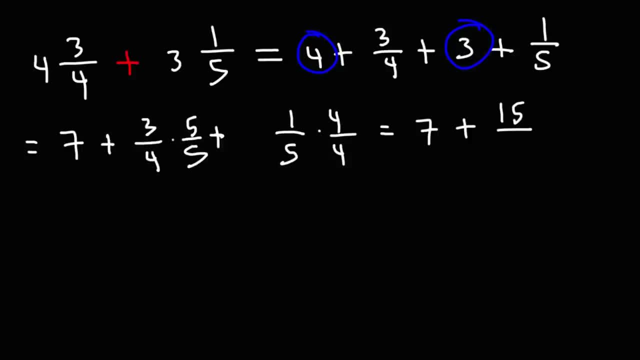 Four times five is twenty, And then this is four over twenty. So now we can add these two fractions, Fifteen over twenty plus four over twenty, That's going to be nineteen over twenty. So the final answer is seven, nineteen-twenties. 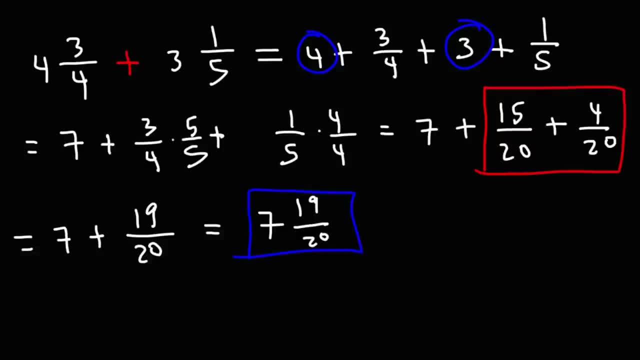 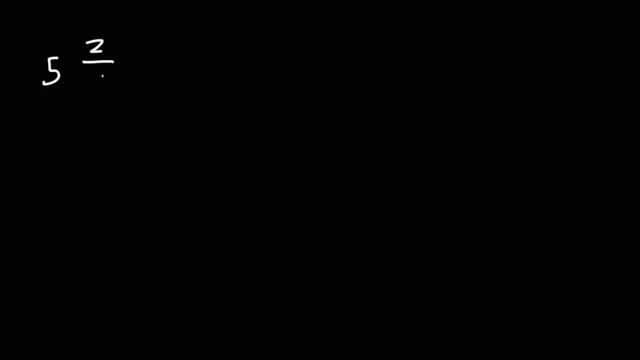 I mean seven and nineteen over twenty. Now let's work on an example where we need to subtract two mixed numbers, So five and two-sevenths minus three and three-fourths. Go ahead and try that example So we can rewrite this as five plus two over seven. 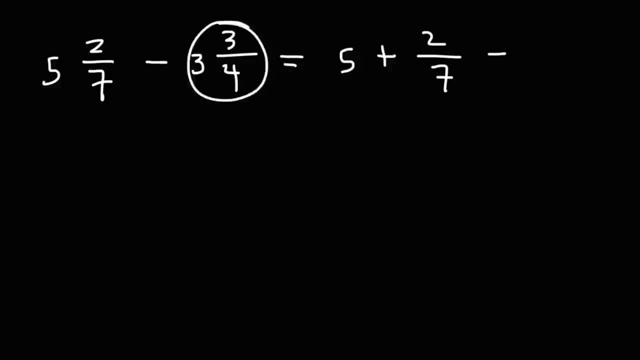 And then minus This is three and three-fourths. But we need to distribute the negative sign to both the three and the three-fourths. So here we have five minus three. Five minus three is two, And then we're left with positive two over seven. 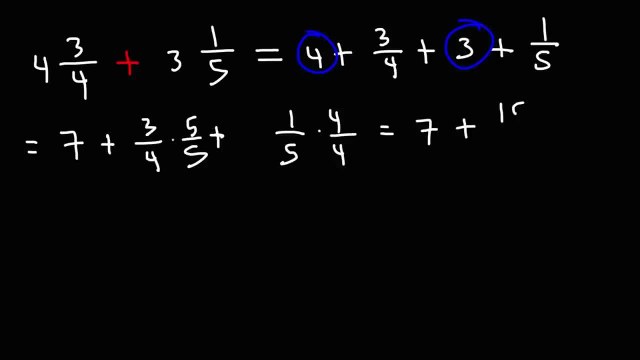 3 times 5 is 15.. 4 times 5 is 12.. And then this is 4 over 20.. And then this is 4 over 20.. So now we can add these two fractions: 15 over 20. 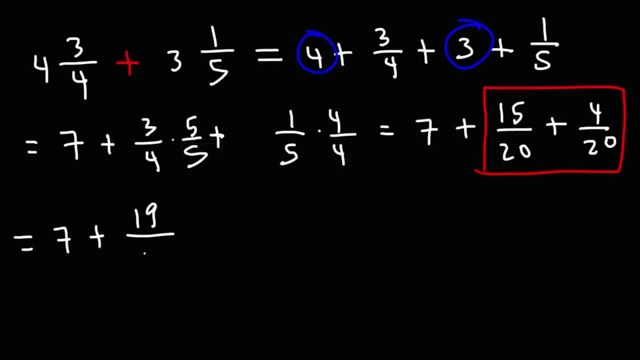 plus 4 over 20.. That's going to be 19 over 20.. So the final answer is 7, 19- 20s. I mean 7 and 19 over 20.. Now let's work on an example where we need to subtract two mixed 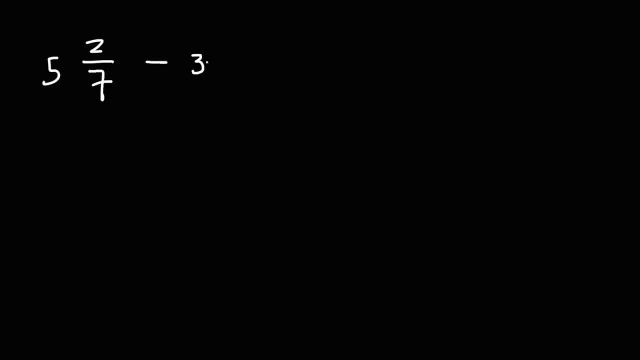 numbers. So 5 and 2 sevenths, minus 3 and 3 fourths. Go ahead and try that example, So we can rewrite this as 5 plus 2 over 7. And then minus this is 3 and 3 fourths. 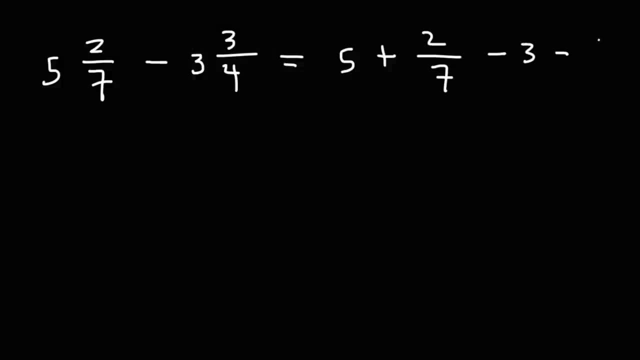 But we need to distribute the negative sign to both the 3 and the 3 fourths. So here we have 5 minus 3.. 5 minus 3 is 2.. And then we're left with positive 2 over 7.. 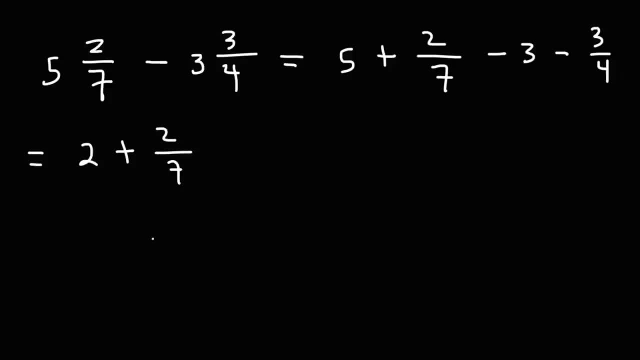 And then negative 3 fourths. So now let's combine these two fractions. We're going to multiply this fraction by 4 over 4.. And we're going to multiply this fraction by 7 over 7 to get common denominators. 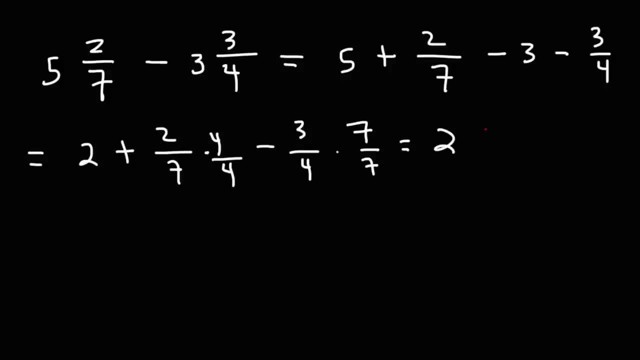 So it's going to be 2.. And then it's plus: this is: 2 times 4 is 8.. 7 times 4 is 28.. So it's 8 over 28.. And then minus 3 times 7 is. 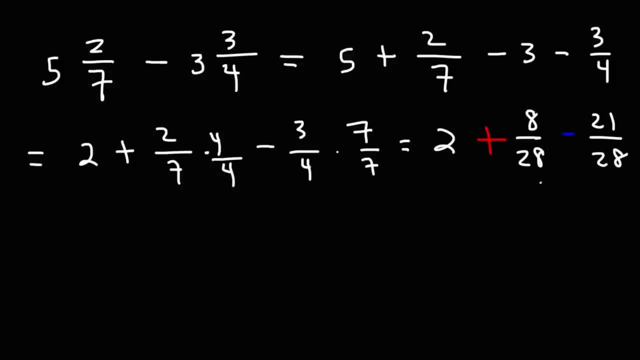 21. And that's going to be over 28 as well. 8 minus 21. That's negative 13.. So we got 2 minus 13 over 28.. So what can we do here? What we're going to do is we're going to borrow a 1. 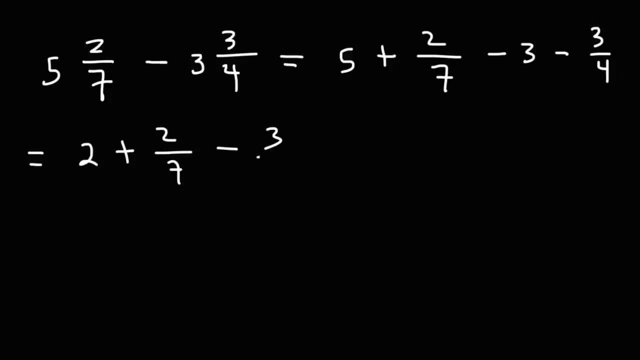 And then negative three-fourths. So now let's combine these two fractions. We're going to multiply this fraction by four over four, And we're going to multiply this fraction by seven over seven To get common denominators. So it's going to be two. 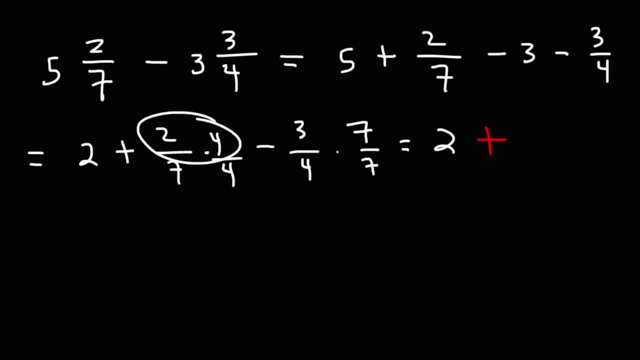 And then it's plus This is two times four is eight. Seven times four is twenty-eight. So it's eight over twenty-eight, And then minus Three times seven is twenty-one, And that's going to be over twenty-eight as well. 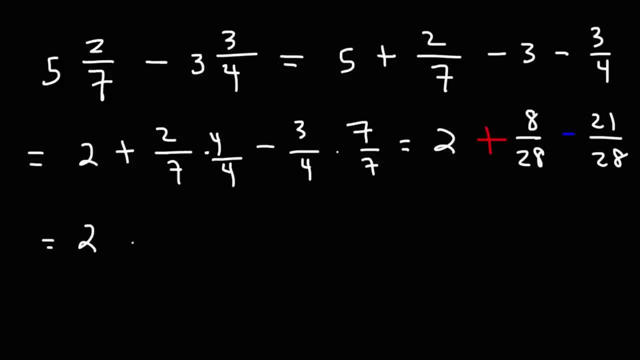 Eight minus twenty-one, That's negative thirteen. So we got two minus thirteen over twenty-eight. So what can we do here? What we're going to do is we're going to borrow a one from the two, So I'm going to write two as one plus one. 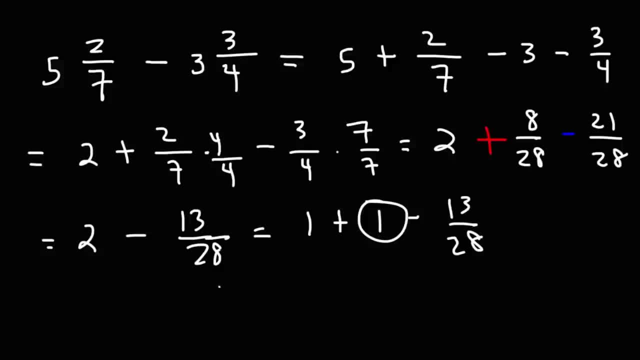 This one. I'm going to convert it into twenty-eight over twenty-eight. A number divided by itself is one, So we have one plus, And then we're going to change this. So basically, what I'm doing is I'm multiplying this one. 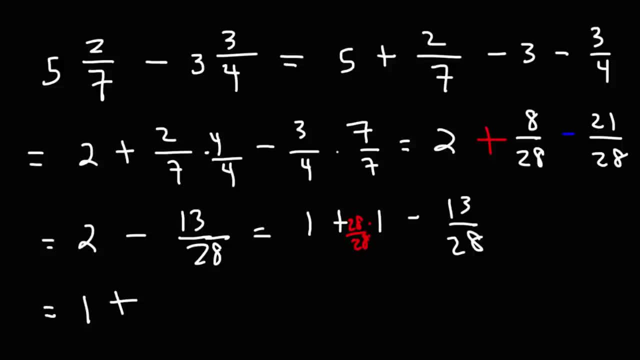 By twenty-eight over twenty-eight, So it becomes twenty-eight over twenty-eight, But it still has the same value as one. So now we can combine these two fractions. Twenty-eight minus thirteen is fifteen, So the final answer is going to be one. 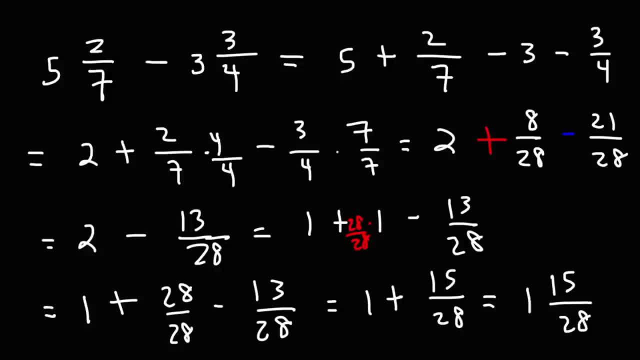 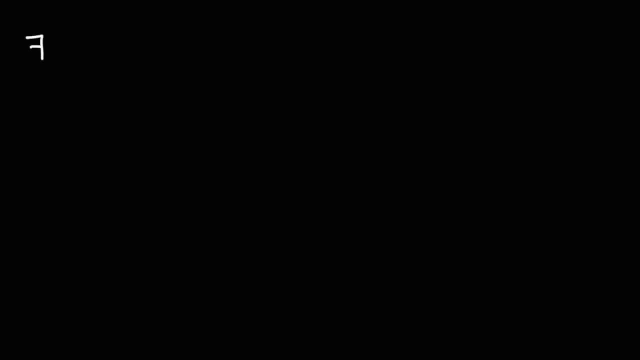 And fifteen over twenty-eight. So that's how we can subtract two mixed numbers. Let's try another example. So let's say, if we have seven and one-eighths, We wish to subtract that by three and four-fifths. Go ahead and try that. 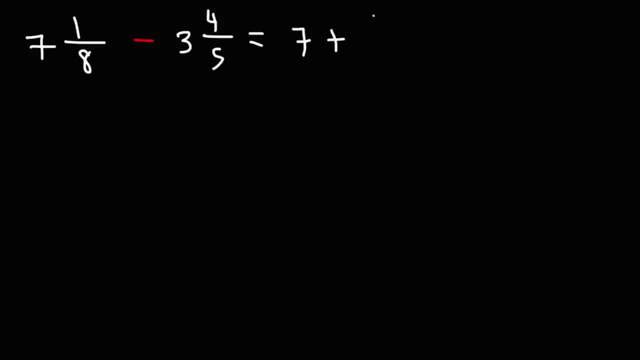 So let's begin by rewriting the problem. This is seven plus one over eight, And then it's minus three, And then minus four over five. Don't forget to distribute the negative to the three And the four over five as well. So now let's combine the whole number. 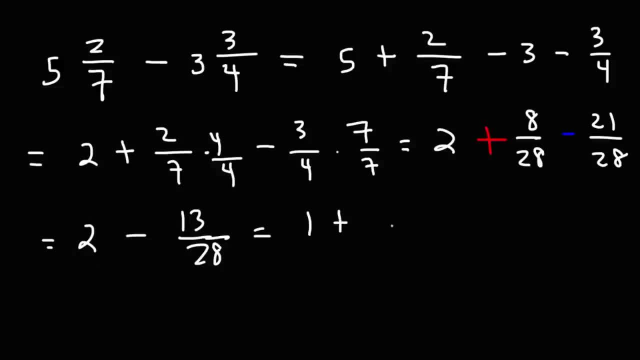 from the 2.. So I'm going to write 2 as 1 plus 1.. This one, I'm going to convert it into 28 over 28.. A number divided by itself is 1.. So we have 1 plus. 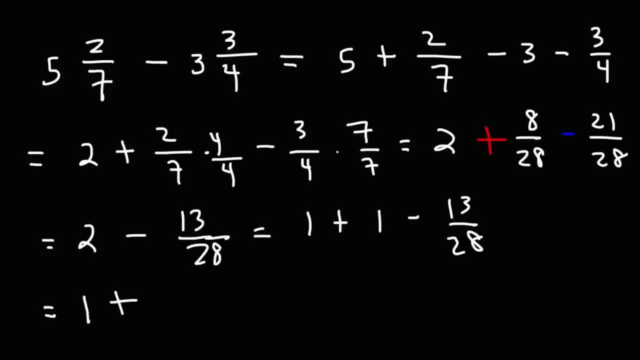 and then we're going to change this. So basically, what I'm doing is I'm multiplying this one by 28 over 28. So it becomes 28 over 28. But it still has the same value as 1.. So now we can combine these two. 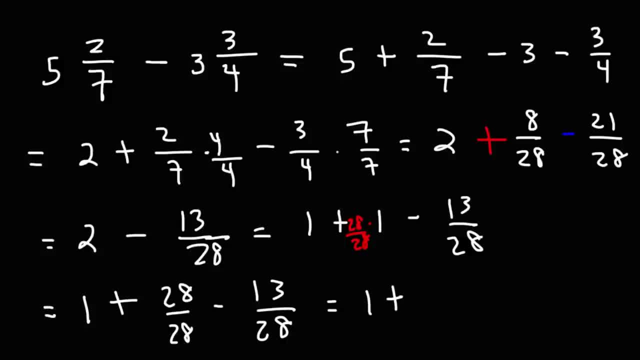 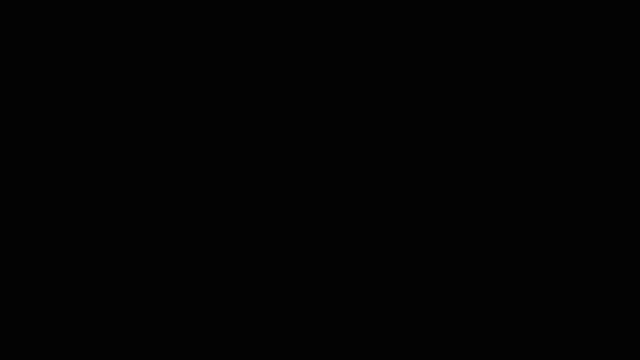 fractions, 28 minus 13 is 15.. So the final answer is going to be 1 and 15 over 28.. So that's how we can subtract two mixed numbers. Let's try another example. So let's say: if we have 7, 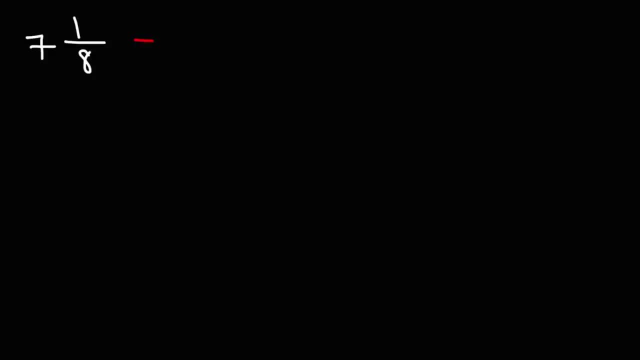 and 1 eighths. we wish to subtract that by 3 and 4 fifths. Go ahead and try that. So let's begin by rewriting the problem. This is 7 plus 1 over 8, and then it's minus 3. 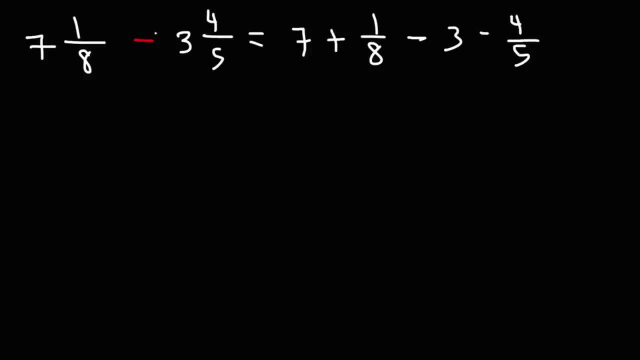 and then minus 4 over 5.. Don't forget to distribute the negative to the 3 and the 4 over 5 as well. So now let's combine the whole numbers, 7 plus negative 3, and that's going to be. 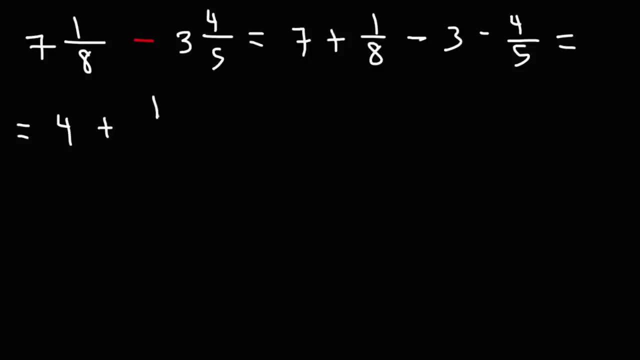 positive 4.. And then we're left with 1 over 8, minus 4 over 5.. So let's get common denominators. Let's multiply this fraction by 5 over 5.. And let's multiply 4 over 5. 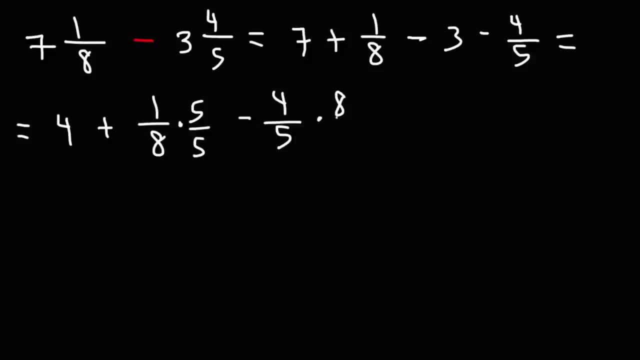 by 8 over 8. This will give us a common denominator of 40. So this is 5, and then 8 times 5 is 40. And then it's going to be minus 4 times 8 is 32, and that will be over 40 as well. 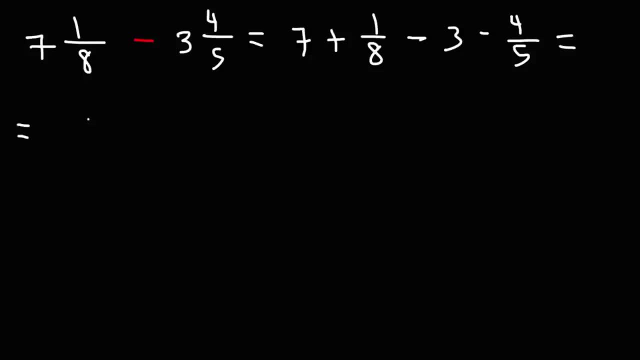 Seven plus negative three, And that's going to be positive four. And then we're left with one over eight Minus four over five. So let's get common denominators. Let's multiply this fraction by five over five, And let's multiply four over five by eight over eight. 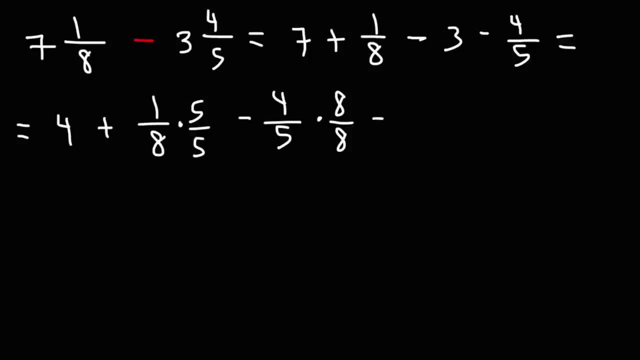 This will give us a common denominator of forty. So this is five, And then eight times five is forty, And then it's going to be minus Four times eight is thirty-two, And that will be over forty as well. Five minus thirty-two. 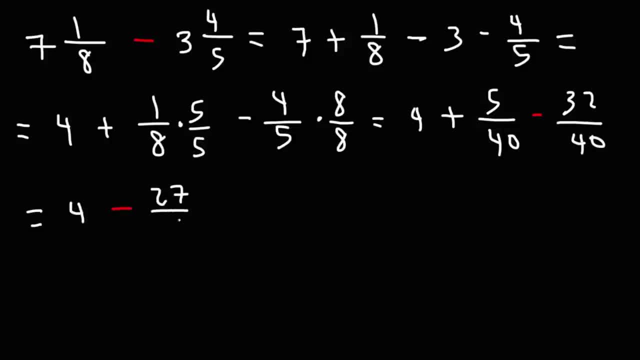 That's going to be negative twenty-seven. So we need to borrow a one from the four. So four, we're going to write that as three plus one. Now, this one, you can write it as one over one, And we're going to multiply it by forty over forty. 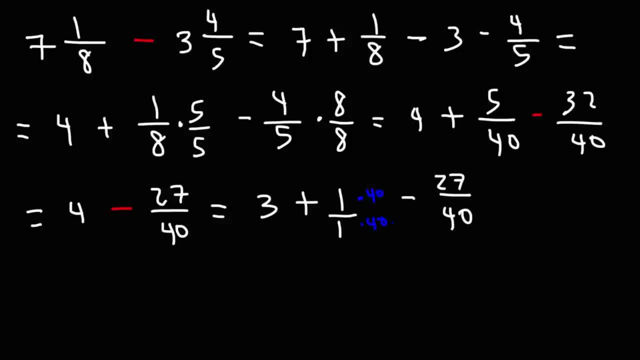 To get common denominators. So what we have now is three plus forty over forty. This right here is equal to four, by the way, And then minus twenty-seven over forty. So forty minus twenty-seven is thirteen. We're going to get three plus thirteen over forty. 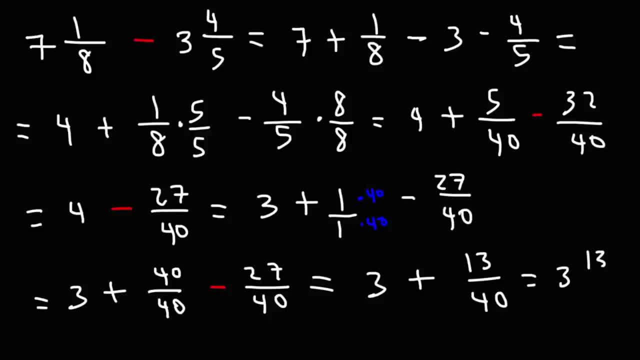 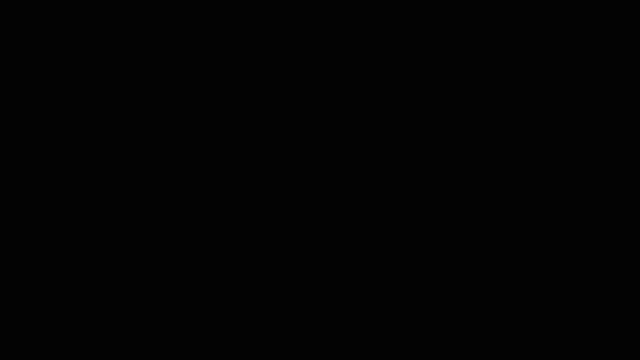 Which means our final answer is three And thirteen over forty. So now you know how to subtract two mixed numbers And how to leave your final answer as a mixed number as well. Now let's talk about how to multiply two mixed numbers. So let's say, if we have seven and one fourths. 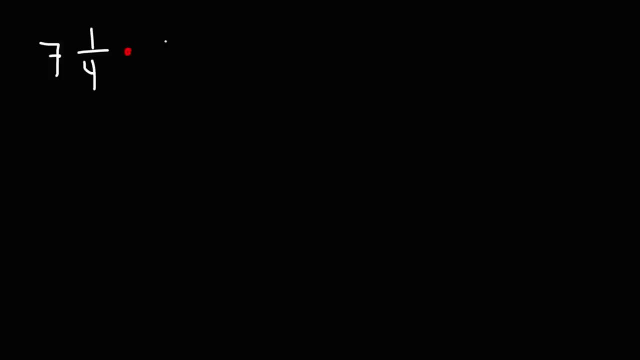 And we want to multiply that by three and two fifths. How can we do this? What I recommend doing is converting each mixed number into an improper fraction. So for the first one, it's going to be seven times four, which is twenty-eight. 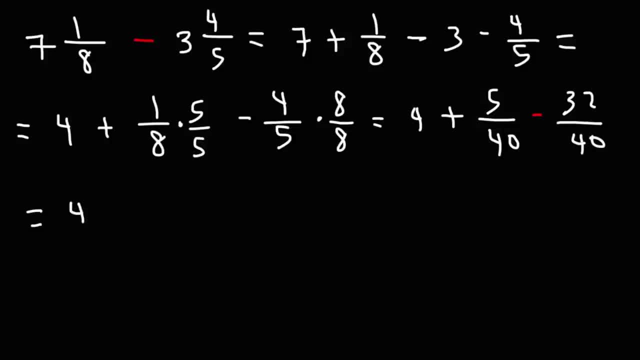 5 minus 32.. That's going to be negative 27.. So we need to borrow a 1 from the 4.. So 4, we're going to write that as 3 plus 1.. Now this 1, you can. 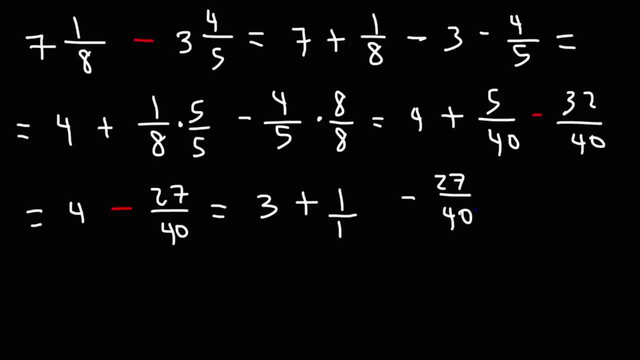 write it as 1 over 1.. And we're going to multiply it by 40 over 40 to get common denominators. So what we have now is 3 plus 40 over 40. This, right here, is equal to 4, by the way. 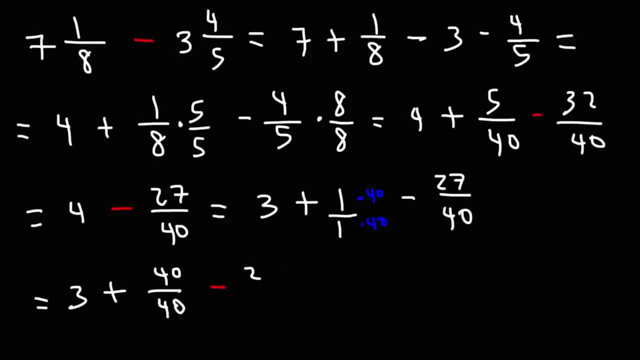 And then minus 27 over 40. So 40 minus 27 is 13.. We're going to get 3 plus 13 over 40. Which means our final answer is 3 and 13 over 40. So now you know how to subtract. 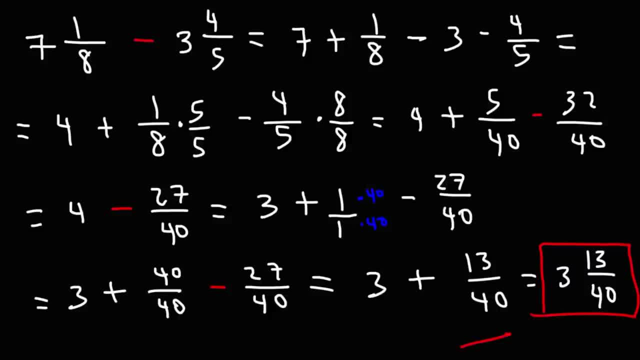 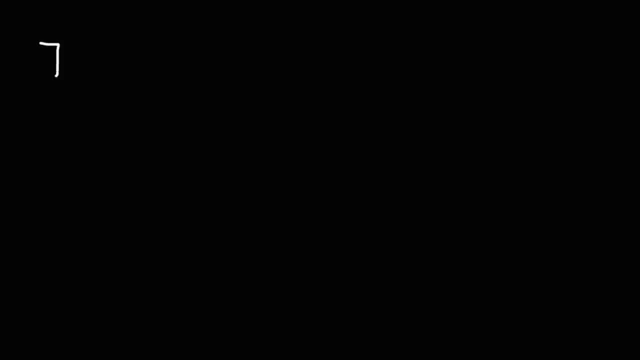 two mixed numbers And how to leave your final answer as a mixed number as well. Now let's talk about how to multiply two mixed numbers. So let's say, if we have 7 and 1 fourths and we want to multiply that by, 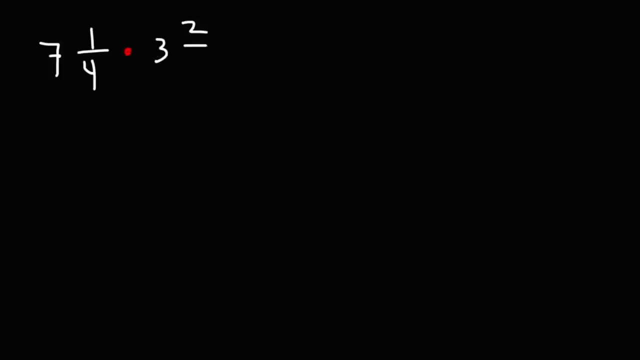 3 and 2. fifths, How can we do this? What I recommend doing is converting each mixed number into an improper fraction. So for the first one, it's going to be 7 times 4, which is 28 plus 1.. So that's. 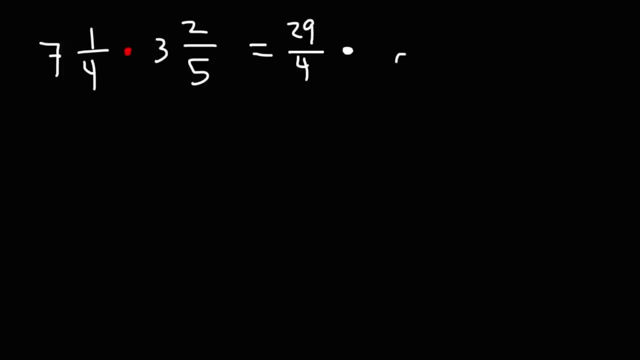 29 over 4.. For the next one, we're going to keep the denominator the same, And then we're going to multiply these two numbers 3 times. 5 is 15 plus 2. So that gives us 17.. And then 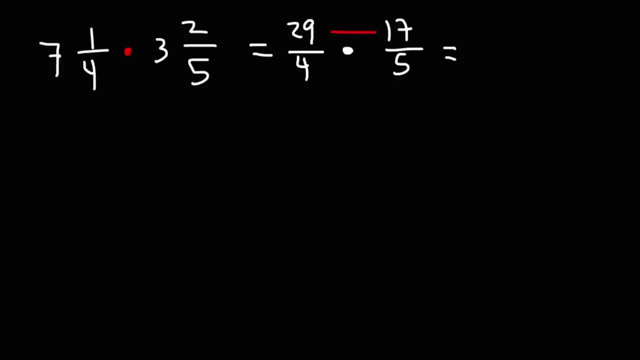 all we need to do is just multiply across 29 times 17, that's 493.. And then 4 times 5 is 20.. And so this is our answer: It's 493 over 20.. And that's how we can. 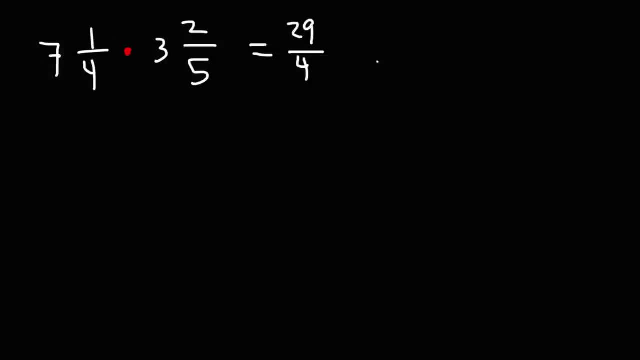 Plus one, So that's twenty-nine over four. For the next one we're going to keep the denominator the same, And then we're going to multiply these two numbers. Three times five is fifteen Plus two, So that gives us seventeen. 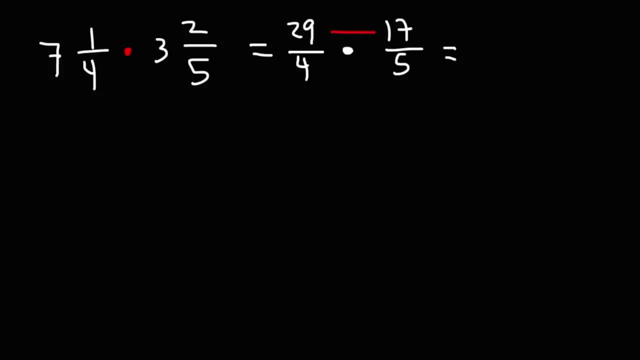 And then all we need to do is just multiply across Twenty-nine times seventeen, That's four hundred and ninety-three, And then four times five is twenty, And so this is our answer: It's four hundred and ninety-three over twenty, And that's how we can multiply two mixed numbers. 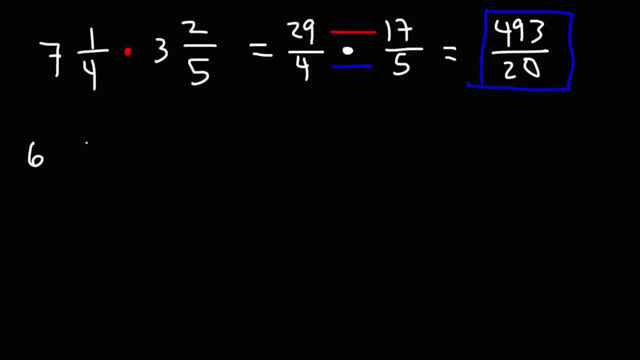 Now let's try another example. So let's multiply six and four, fifths By seven and two-thirds. Go ahead and try that. So let's convert the first mixed number into an improper fraction. Let's begin by rewriting the denominator, And then it's going to be six times five, which is thirty. 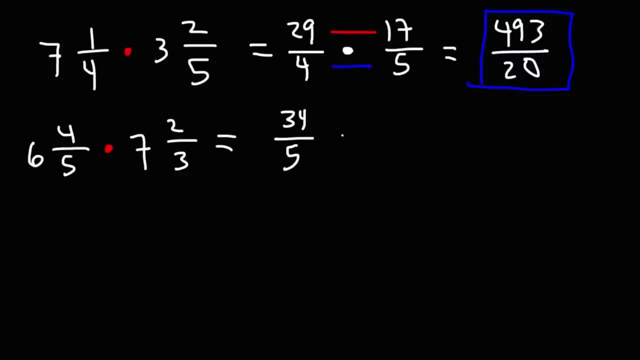 Plus four, That's going to give us thirty-four. And then times. Let's write the denominator of the other fraction. This is going to be seven times three, which is twenty-one Plus two, That's twenty-three. And now let's multiply across. 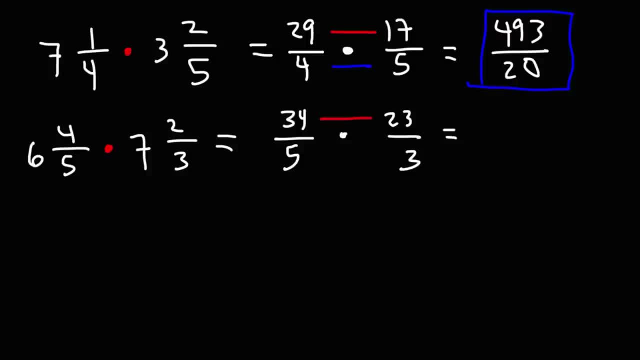 Thirty-four times twenty-three- I'm using the calculator for that- That's going to be seven hundred and eighty-two, And then five times three, that's fifteen. So the answer is seven hundred eighty-two over fifteen. By the way, for those of you who want to review long multiplication, 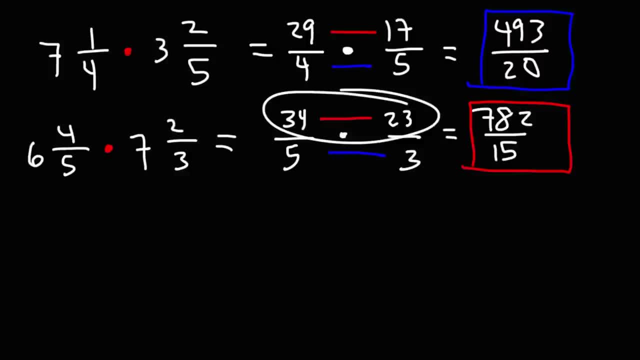 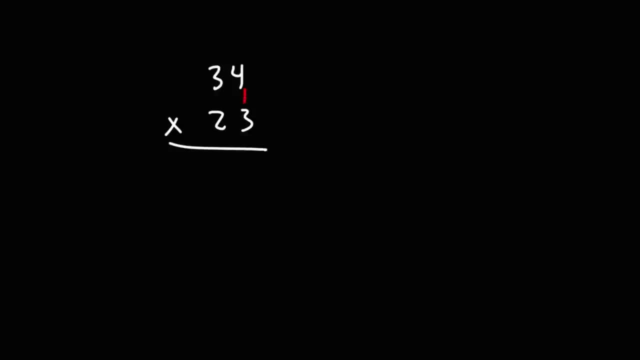 here's what you can do if you don't have a calculator And you want to multiply those two numbers. So first we have four times three, which is twelve, Write the two, carry over the one, And then three times three is nine. 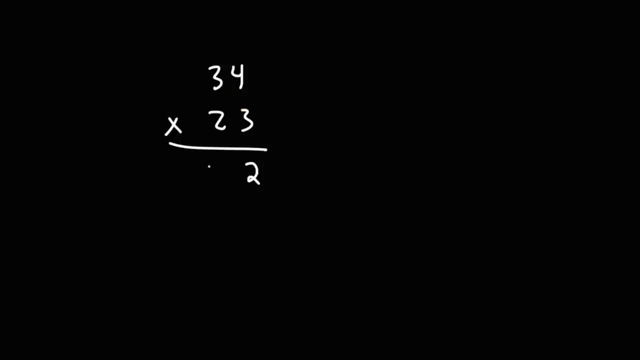 Plus one is ten, So we can write ten here. Next: put a zero Two times four is eight, And then two times three is six, And then you can add: Two plus zero is two, Zero plus eight is eight. One plus six is seven. 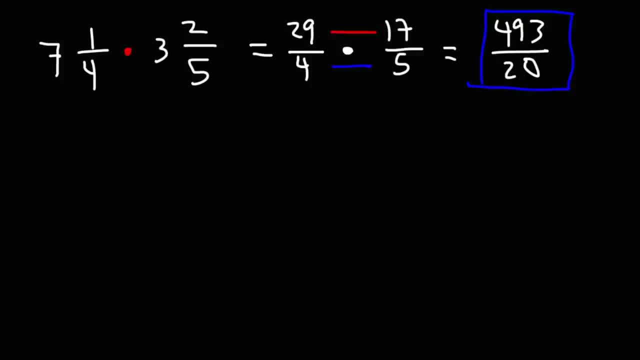 multiply two mixed numbers. Now let's try another example. So let's multiply 6 and 4 fifths by 7 and 2 thirds. Go ahead and try that. So let's convert the first mixed number into an improper fraction. Let's begin by rewriting the denominator. 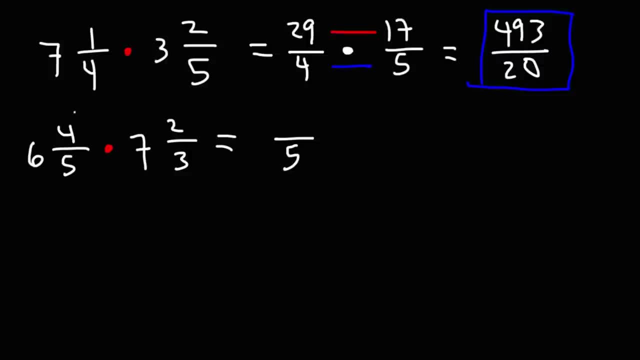 And then it's going to be 6 times 5, which is 30 plus 4.. That's going to give us 34.. And then times- let's write the denominator of the other fraction. This is going to be 7 times 3, which is. 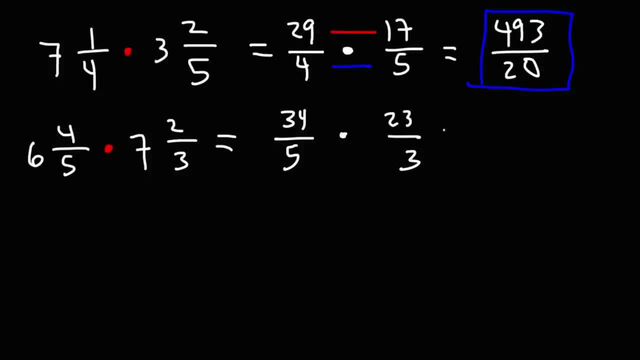 21 plus 2, that's 23.. And now let's multiply across 34 times 23.. I'm using the calculator for that. That's going to be 782.. And then 5 times 3, that's 15.. 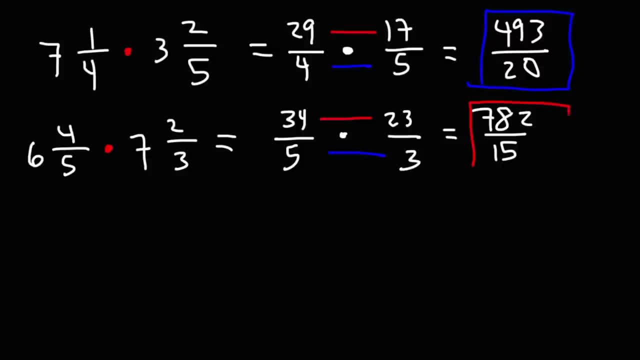 So the answer is 782 over 15.. By the way, for those of you who want to review long multiplication, here's what you can do if you don't have a calculator And you want to multiply those two numbers. So first we have 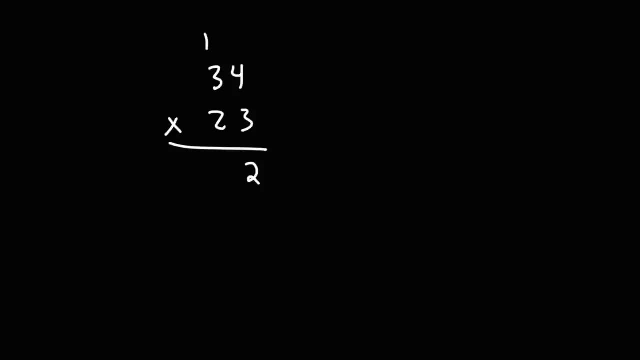 4 times 3, which is 12.. Write the 2, carry over the 1. And then 3 times 3 is 9 plus 1 is 10.. So we can write 10 here. Next put a 0.. 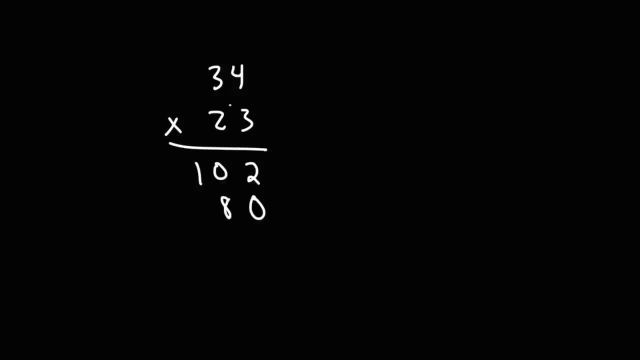 2 times 4 is 8.. And then 2 times 3 is 6.. And then you can add: 2 plus 0 is 2.. 0 plus 8 is 8.. 1 plus 6 is 7.. 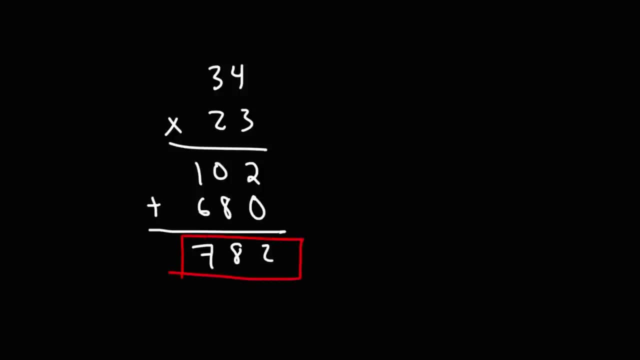 So that's a quick review of how you can perform long multiplication. Now let's talk about how we can divide two mixed numbers. So let's say we have 5 and 2 sevenths And we wish to divide that by 3 and 1- fourth. 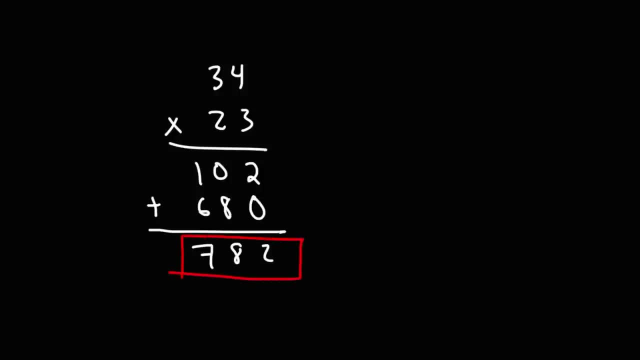 So that's a quick review of how you can perform long multiplication. Now let's talk about how we can divide two mixed numbers. So let's say we have five and two sevenths And we wish to divide that by three and one fourth. 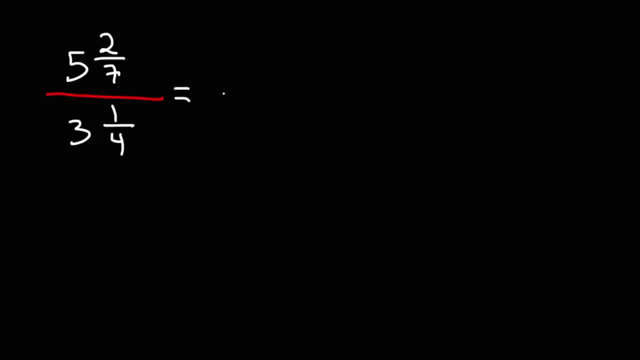 What I recommend doing is converting each mixed number into an improper fraction. So let's write the denominator first, And then we have five times seven, which is thirty-five plus two. So this is thirty-seven over seven. For the next one, let's begin by writing the denominator four. 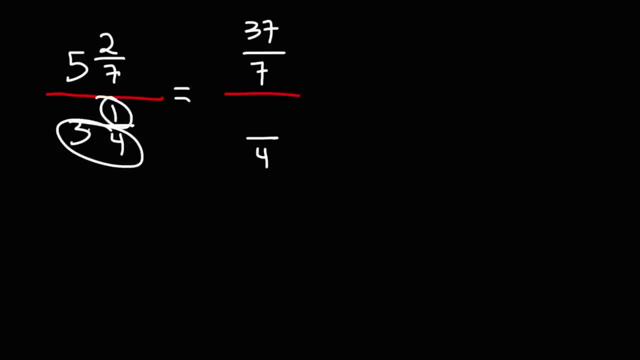 And then it's four times three, which is twelve plus one, That's thirteen. So we're dividing these two improper fractions So we can rewrite it as thirty-seven over seven divided by thirteen over four. Now, using keep change flip, we're going to keep the first fraction the same. 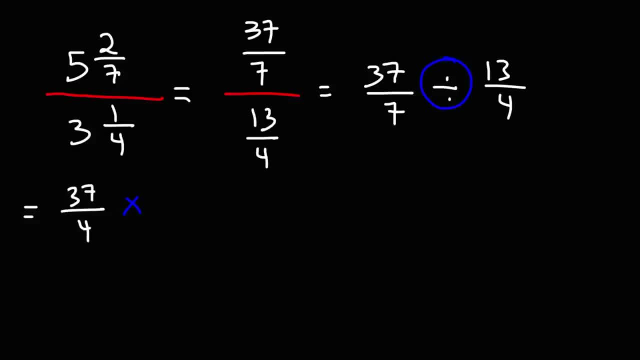 We're going to change division to multiplication And then we're going to flip the second fraction, So this is going to be four over thirteen. For some reason I wrote four here. This should be a seven. I don't know why I put a four. 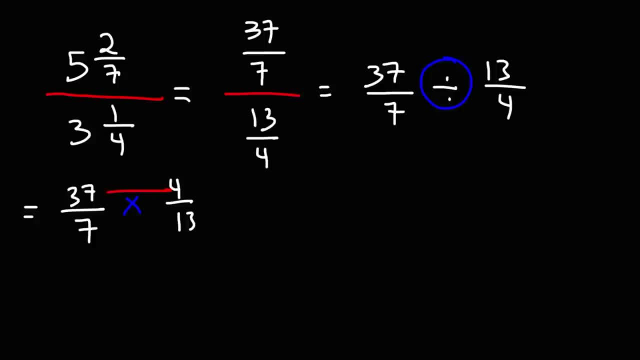 But now what we can do is we can multiply across. So thirty-seven times four is a hundred and forty-eight, And then seven times thirteen is ninety-one, So the answer is one hundred forty-eight over ninety-one. Let's try another example. 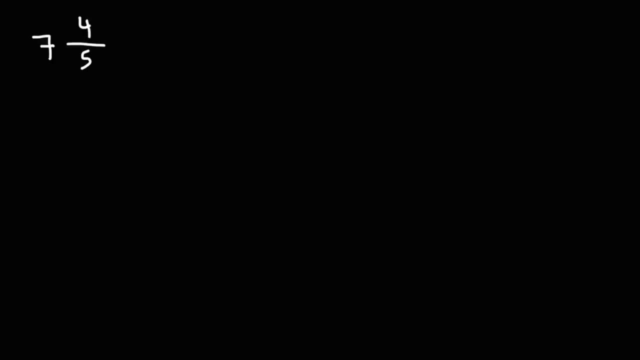 Let's divide seven and four fifths by three and two sevenths. So feel free to try that. So let's begin by converting each mixed number into an improper fraction. So five times seven is thirty-five. plus four, That's going to be thirty-nine. 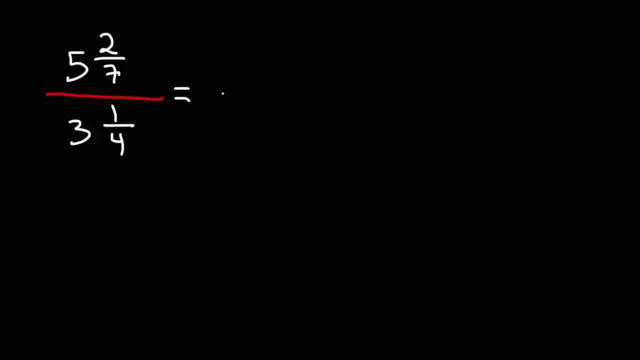 What I recommend doing is converting each mixed number into an improper fraction. So let's write the denominator first, And then we have 5 times 7, which is 35 plus 2. So this is 37 over 7.. For the next one, let's begin by writing: 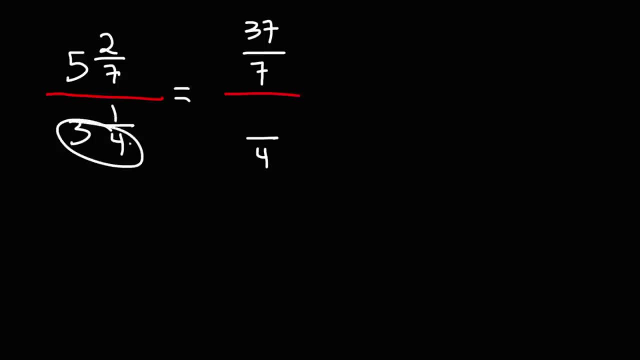 the denominator 4.. And then it's 4 times 3, which is 12 plus 1. That's 13.. So we're dividing these two improper fractions So we can rewrite it as 37 over 7, divided by 13 over 4.. 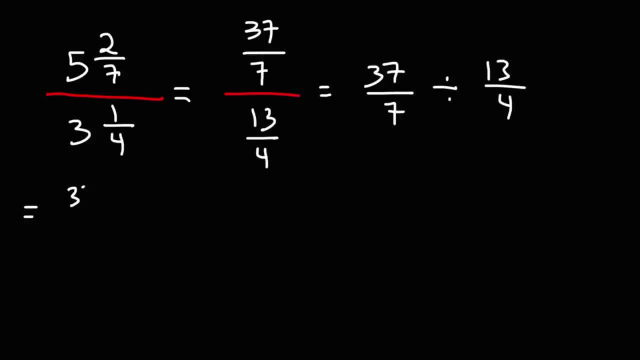 Now using keep, change, flip. we're going to keep the first fraction the same, We're going to change division to multiplication And then we're going to flip the second fraction. So this is going to be 4 over 13.. For some reason, 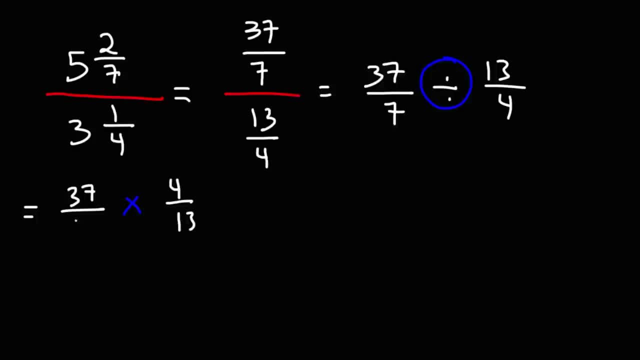 I wrote 4 here. This should be a 7.. I don't know why I put a 4.. But now what we can do is we can multiply across. So 37 times 4 is 148.. And then 7 times 13. 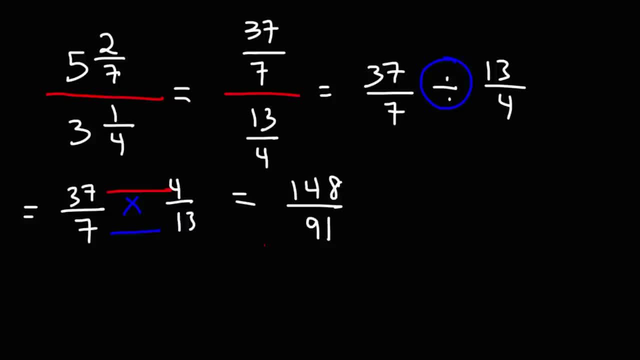 is 91. So the answer is 148 over 91.. Let's try another example. Let's divide 7 and 4 fifths by 3 and 2 sevenths. So feel free to try that. So let's begin by converting each. 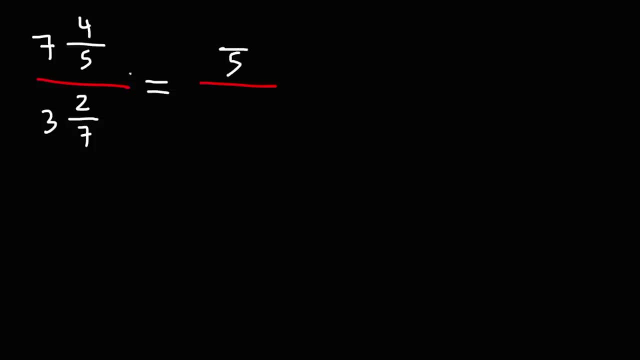 mixed number into an improper fraction. So 5 times 7 is 35 plus 4.. That's going to be 39.. 3 times 7 is 21 plus 2. That's 23.. So what we have now is 39 over 5. 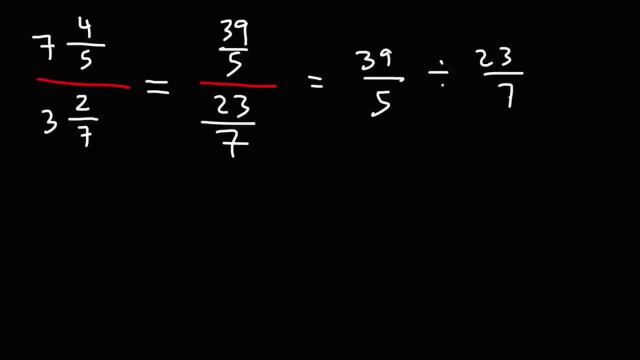 divided by 23 over 7.. Using keep, change, flip. we're going to keep the first fraction the same And, just like before, we're going to change division to multiplication, And then we're going to flip the second fraction. So now let's multiply. 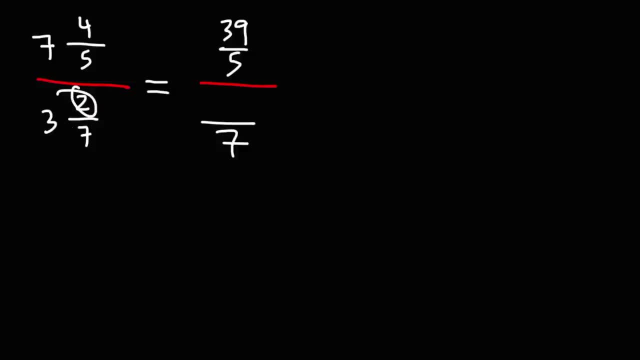 Three times seven is twenty-one plus two, That's twenty-three. So what we have now is thirty-nine over five, Divided by twenty-three over seven. Using keep change flip. we're going to keep the first fraction the same And, just like before, we're going to change division to multiplication. 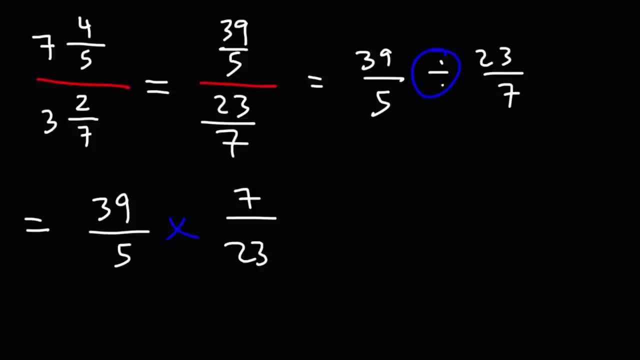 And then we're going to flip the second fraction. So now let's multiply across. So we have thirty-nine times seven, which is two hundred and seventy-three, Five times twenty-three. Five times twenty is a hundred. Three times five is fifteen. 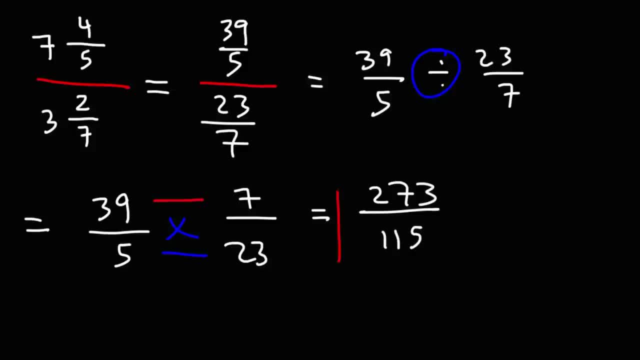 So this is one fifteen. So now you know how to divide two mixed numbers. But you know what? Since the original problem was a mixed number, let's convert this improper fraction back into a mixed number. One fifteen goes into two hundred seventy-three, two times. 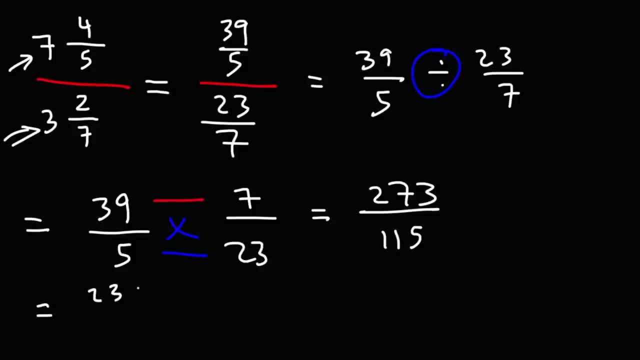 One fifteen times two is two hundred thirty. If we subtract two seventy-three by two thirty, that's going to be forty-three. So these are the two numbers that I want to break up two seventy-three into Two thirty plus forty-three. Now we know that two thirty divided by one fifteen is two. 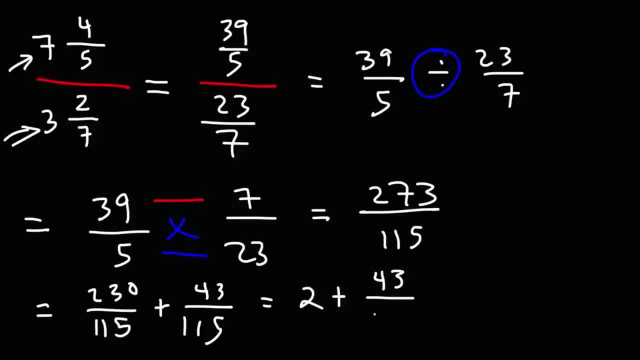 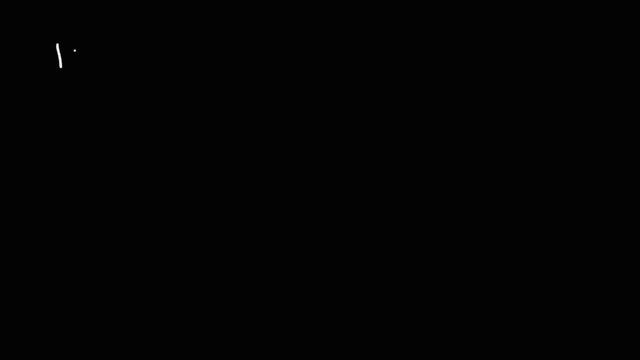 So we get two plus forty-three over one fifteen, And so our final answer as a mixed number is two forty-three over one fifteen. Now, going back to the previous problem, where we had our answer as one forty-eight over ninety-one, Let's convert that into a mixed number as well. 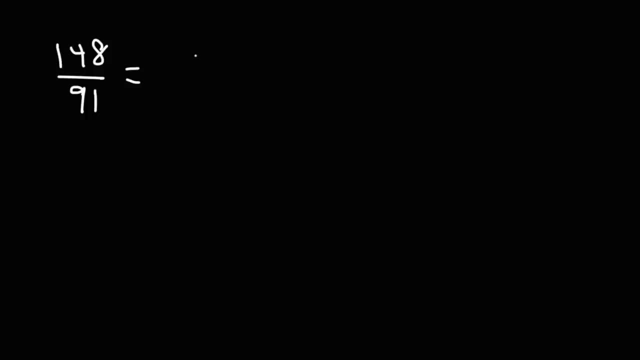 Ninety-one goes into one forty-eight one time. So the highest multiple of ninety-one below one forty-eight is ninety-one. Now, if we subtract one forty-eight by ninety-one, that's going to be fifty-three Fifty-seven. So ninety-one plus fifty-seven is one forty-eight. 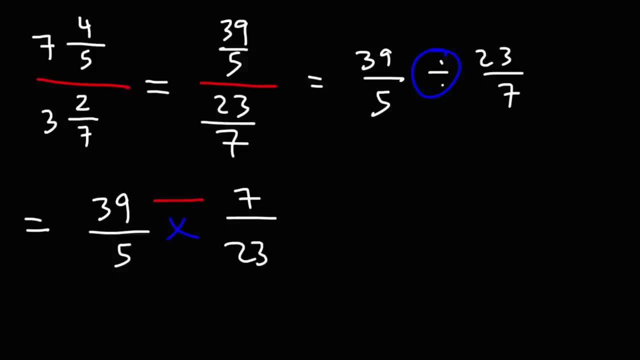 across. So we have 39 times 7, which is 273.. 5 times 23.. 5 times 20 is 100.. 3 times 5 is 15.. So this is 115.. So now you know how to divide two mixed. 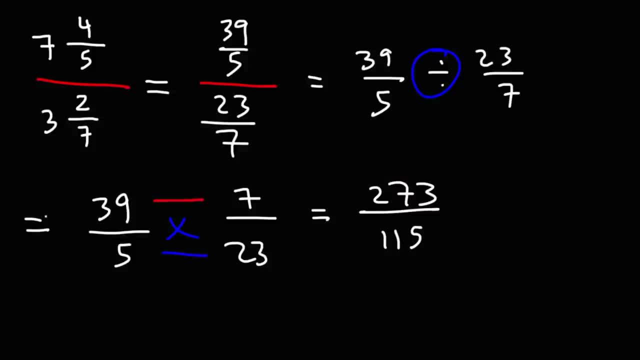 numbers. But you know what, Since the original problem was a mixed number, let's convert this improper fraction back into a mixed number. 115 goes into 273. two times 115 times 2 is 230.. If we subtract 273 by 230,. 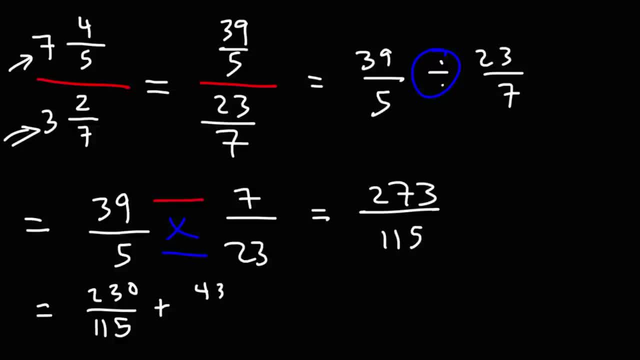 that's going to be 43.. So these are the two numbers that I want to break up: 273 into 230 plus 43.. Now we know that 230 divided by 115 is 2.. So we get 2 plus 43 over 115.. 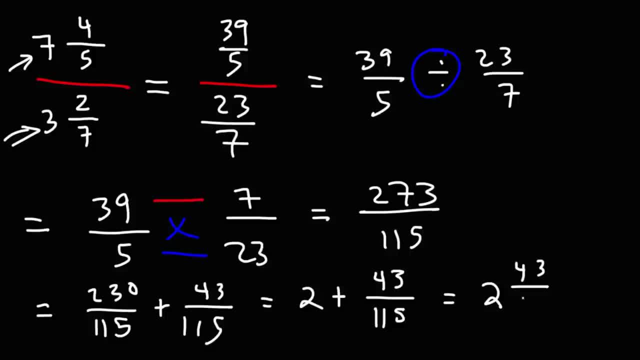 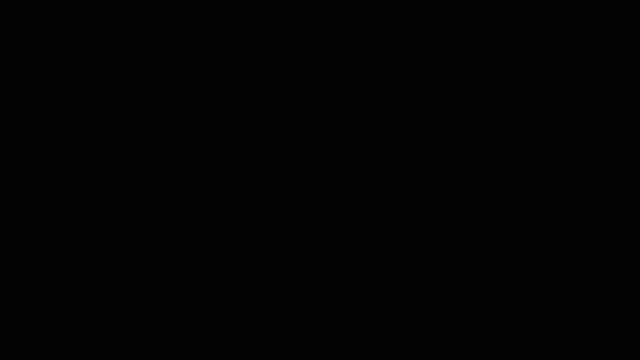 And so our final answer as a mixed number is 243 over 115.. Now going back to the previous problem, where we had our answer as 148 over 91.. Let's convert that into a mixed number as well. 91 goes into 148 one time. 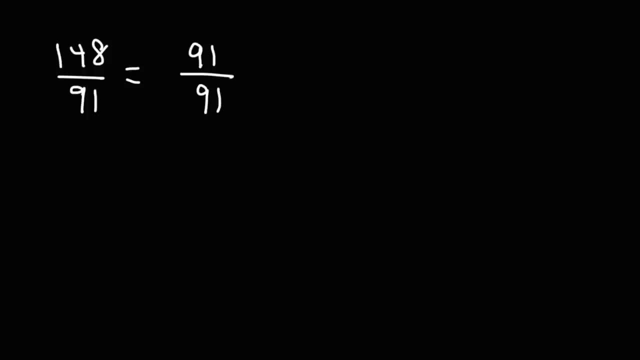 So the highest multiple of 91 below 148 is 91.. Now if we subtract 148 by 91, that's going to be 57. So 91 plus 57 is 148.. 91 divided by itself becomes 1.. 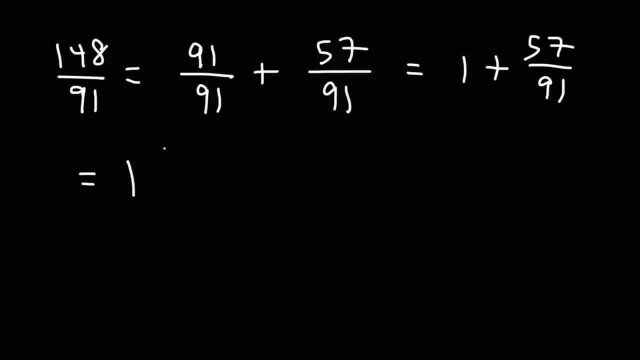 So the final answer, as a mixed number, is 157 over 91.. Now let's talk about how to convert a fraction into a decimal. So what is the decimal value of 3 over 4?? In order to convert a fraction into a decimal, 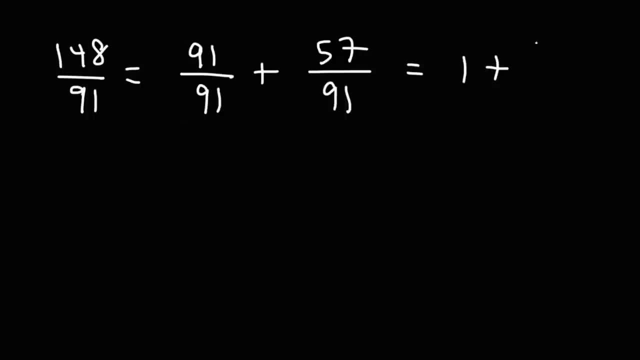 Ninety-one divided by itself becomes one. So the final answer, as a mixed number, is one: fifty-seven over ninety-one. Now let's talk about how to convert a fraction into a decimal. So what is the decimal value of three over four In order to convert a fraction into a decimal? 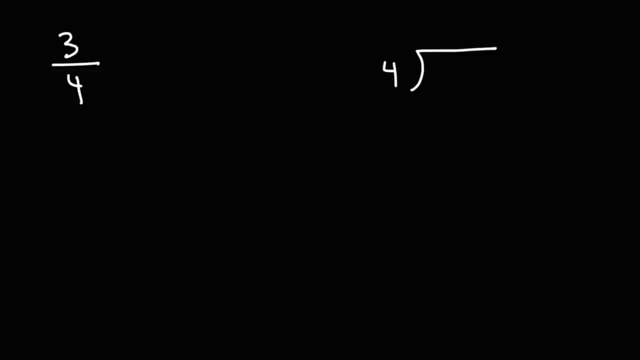 you could use division. So we're dividing three by four. Now, four doesn't go into three, At least nicely. So what we're going to do is we're going to add a decimal point and a zero. Now we're going to treat three point zero as if it's thirty. 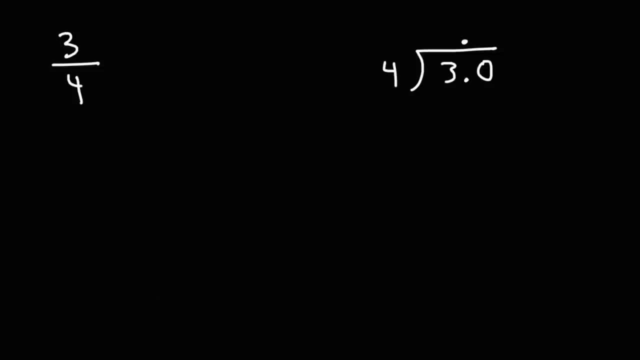 And we're going to put a decimal point here as well. How many times does four go into thirty? Four goes into thirty seven times. If you're not sure about this, what you can do is you can write a list of the multiples of four. 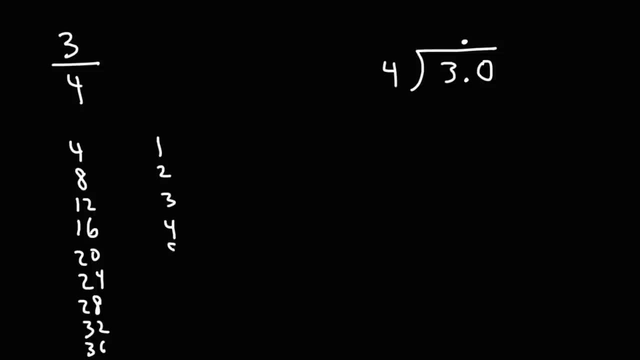 This is one, two, three, four, five, six, seven, eight, nine. The highest multiple of four under thirty is seven, I mean it's twenty-eight, And four times seven is twenty-eight, So four goes into thirty seven times. 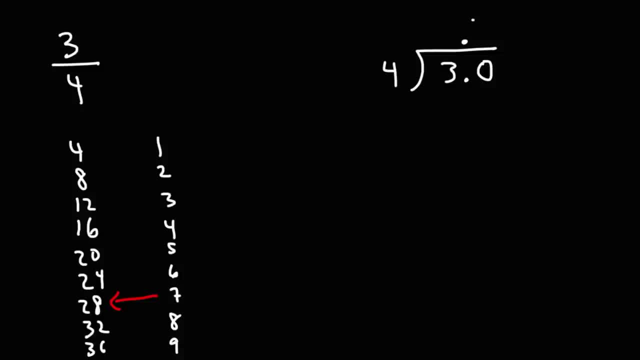 Or we could say: four goes into three point zero. point seven times Four times seven is twenty-eight. So four times point seven is two point eight. If we subtract these two we're going to get point two, And then we're going to add a zero. 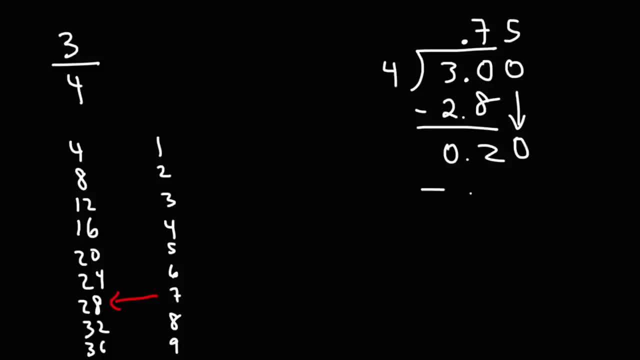 Now four goes into twenty five times. Now the remainder is zero. The answer is what we have here: Three over four is equal to point seven, five as a decimal. So that's how you can convert a fraction into a decimal. It's by using long division. 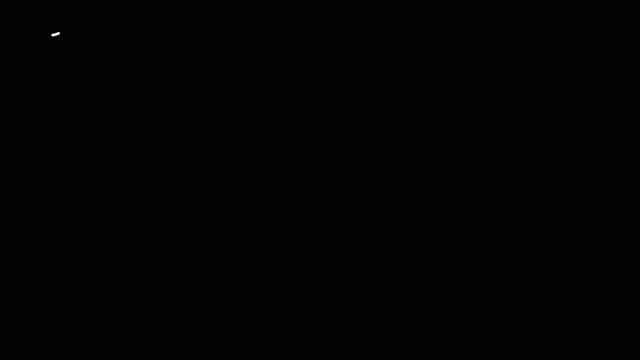 Let's try another example. Let's convert seven over eight into a decimal. Actually, let's say three and seven, eighths. Let's use a mixed number. Let's convert this mixed number into a decimal value. So keep in mind: this is three plus seven over eight. 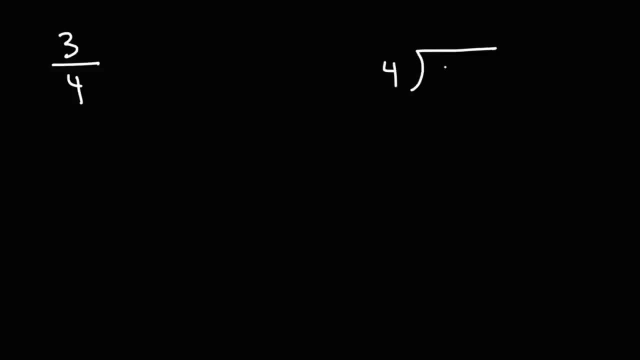 you could use division. So we're dividing 3 by 4.. Now, 4 doesn't go into 3, at least nicely. So what we're going to do is we're going to add a decimal point and a 0. Now we're going to treat 3.0 as if. 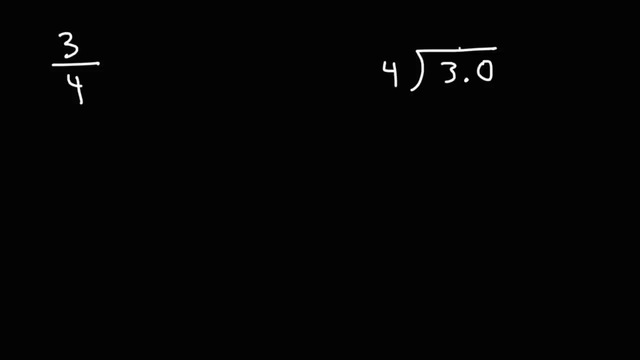 it's 30. And we're going to put a decimal point here as well. How many times does 4 go into 30?? 4 goes into 30, 7 times. If you're not sure about this, what you can do is: 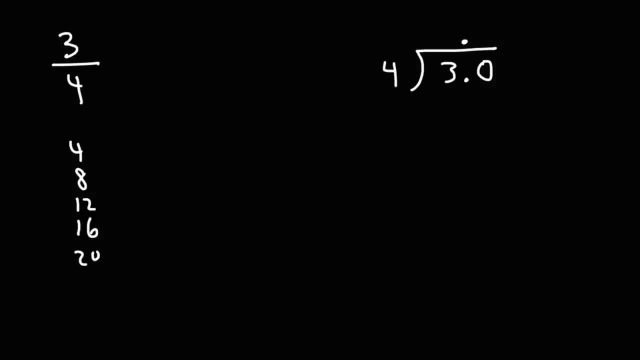 you can write a list of the multiples of 4.. This is 1,, 2,, 3,, 4,, 5,, 6,, 7,, 8,, 9.. The highest multiple of 4 under 30 is 7.. I mean it's. 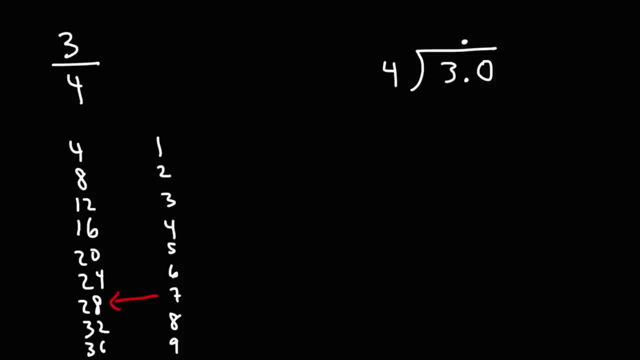 28.. And 4 times 7 is 28.. So 4 goes into 30 7 times. Or we could say 4 goes into 3.0, 0.7 times. 4 times 7 is 28.. 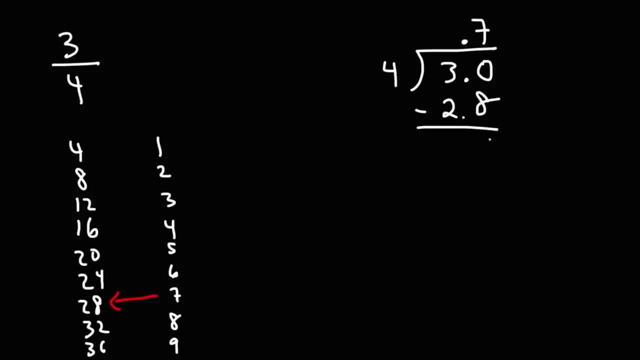 So 4 times 0.7 is 2.8.. If we subtract these two, we're going to get 0.2.. And then we're going to add a 0.. Now 4 goes into 20, 5 times. 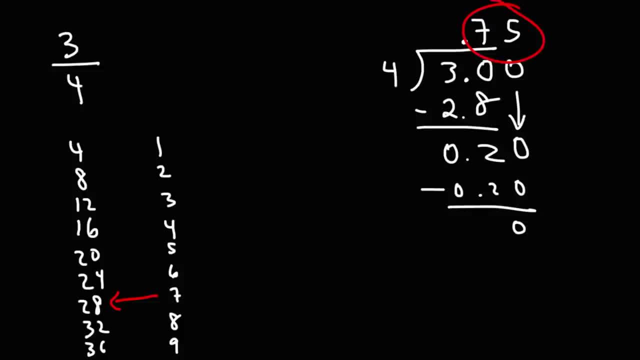 Now the remainder is 0.. The answer is what we have here: 3 over 4 is equal to 0.75 as a decimal. So that's how you can convert a fraction into a decimal. It's by using long division. 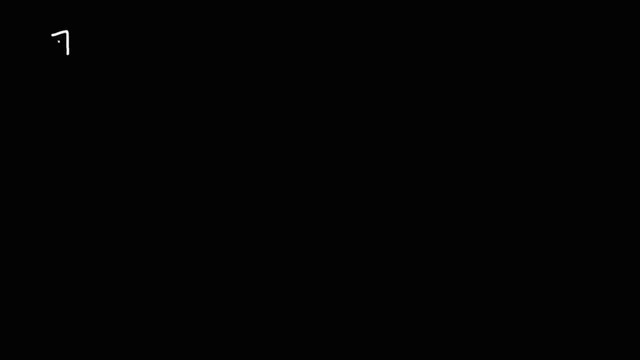 Let's try another example. Let's convert 7 over 8 into a decimal. Actually, let's say 3 and 7 eighths. Let's use a mixed number. Let's convert this mixed number into a decimal value. So keep in mind, this is 3 plus. 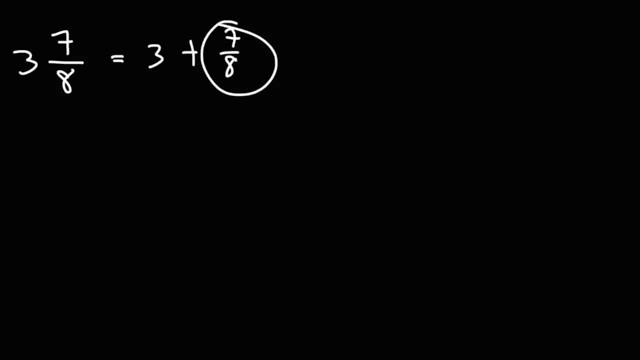 7 over 8.. Now the fractional part. we're going to convert that to a decimal using long division, So we're going to put the denominator on the outside. 8 doesn't go into 7 nicely, So we're going to use 7.0.. 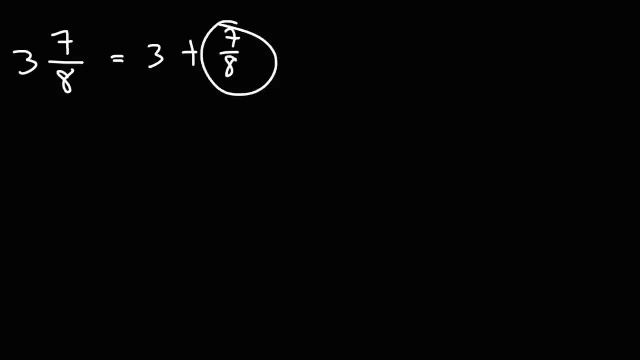 Now the fractional part. we're going to convert that to a decimal using long division, So we're going to put the denominator on the outside. Eight doesn't go into seven nicely, So we're going to use seven, point. oh. Now how many times does eight go into seventy? 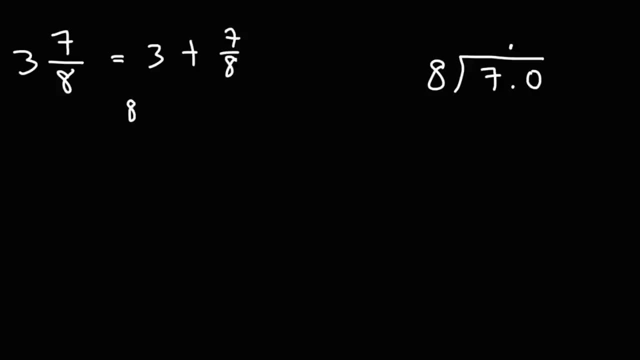 If you're not sure, you can write out the multiples of eight And you really don't need to go past nine. The highest multiple of eight under seventy is sixty-four. So we can say eight goes into seventy. eight times Eight times eight is sixty-four. 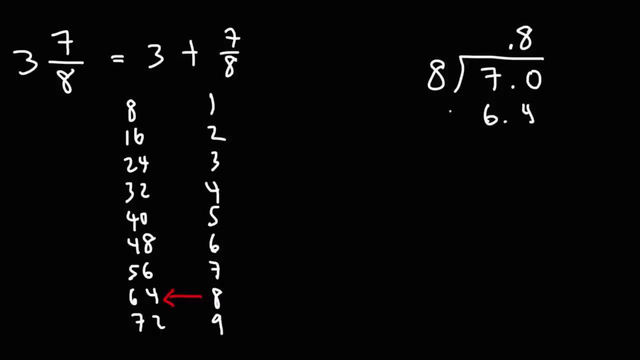 So eight times point eight is six point four. Seventy minus sixty-four is six. So seven point oh minus six point four is point six. Now let's bring down a zero. How many times does eight go into sixty? The highest multiple of eight under sixty is fifty-six. 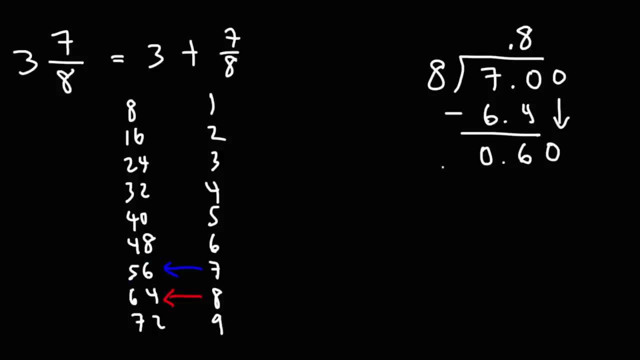 So we can say: eight goes into sixty. seven times Eight times point zero, seven, That's going to be point fifty-six. And now we can subtract sixty by fifty-six, We're going to get four. And then let's bring down another zero. 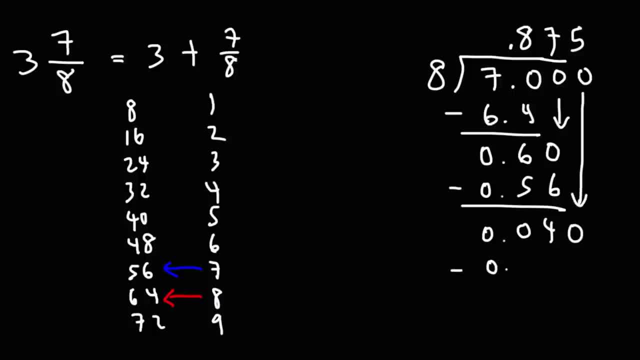 Eight goes into forty five times, And now we have a remainder of zero. So this is going to be the value of seven over eight. So this becomes three plus. We're going to replace this with that number. So it's three plus point eight, seven, five. 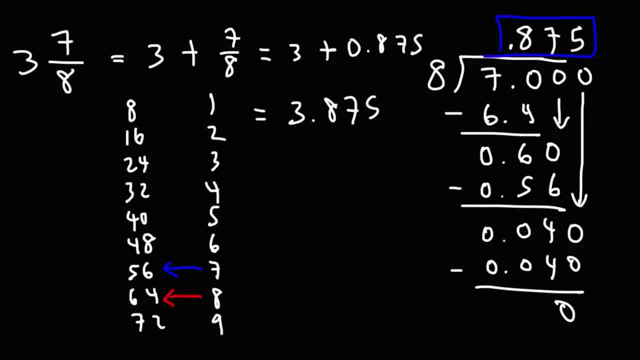 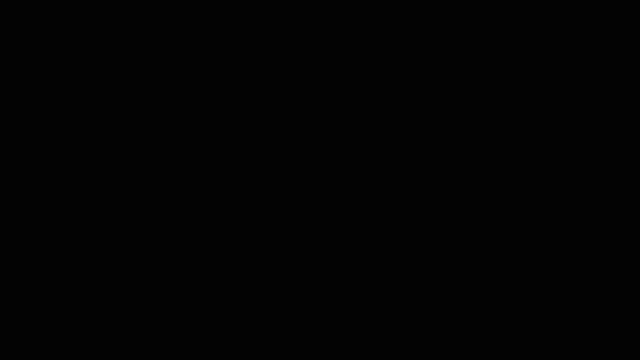 So we get three point eight, seven, five. So that is the value of this particular mixed number. Now it helps to know the common values of some fractions. One over two is point five. One over three is point three. repeated One over four is point two, five. 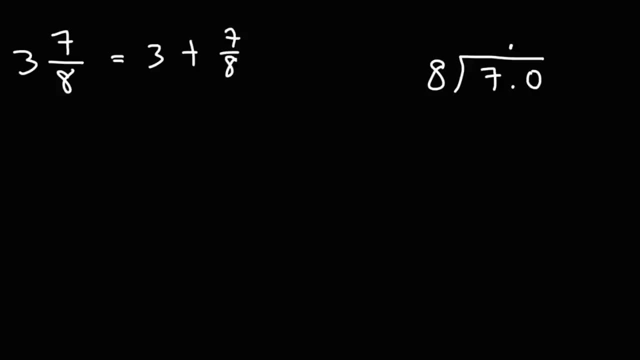 Now, how many times does 8 go into 70?? If you're not sure, you can write out the multiples of 8. And you really don't need to go past 9.. The highest multiple of 8 under 70 is 64.. 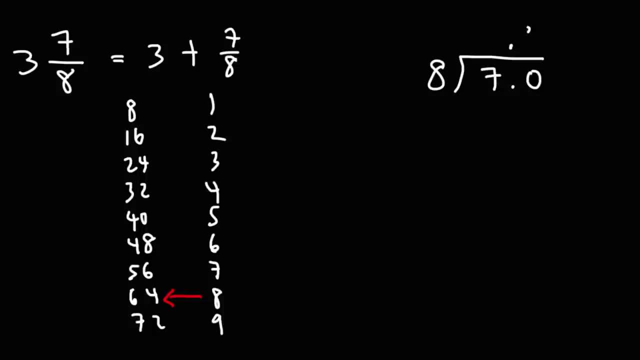 So we can say: 8 goes into 70. 8 times 8 times 8 is 64,, so 8 times .8 is 6.4.. 70 minus 64 is 6.. So 7.0 minus 6.4 is .6.. 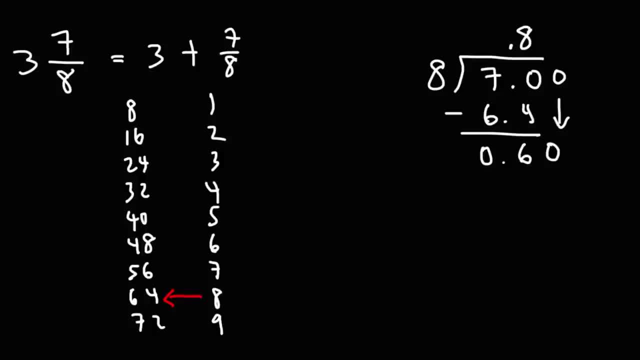 Now let's bring that to 0.. How many times does 8 go into 60?? The highest multiple of 8 under 60 is 56.. So we can say 8 goes into 60 7 times, 8 times .07. 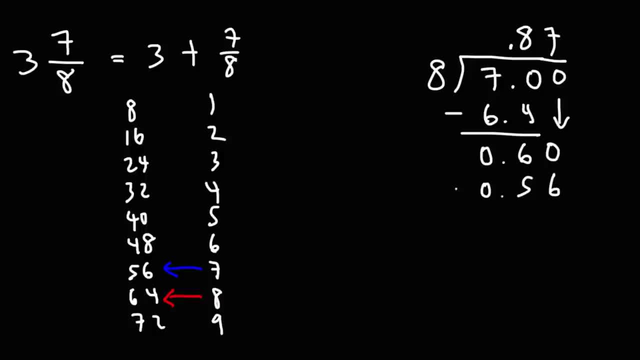 that's going to be .56.. And now we can subtract 60 by 56, we're going to get 4.. And then let's bring down another 0.. 8 goes into 40 5 times, And now we have a remainder of 0.. 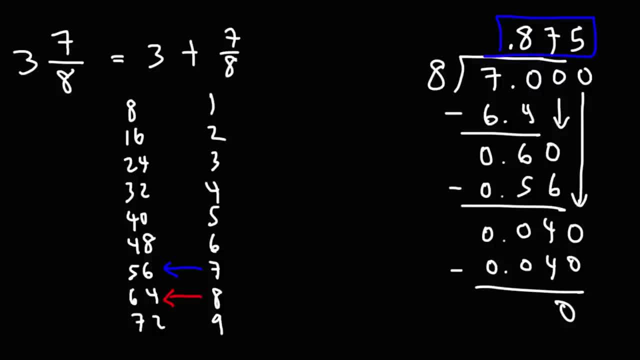 So this is going to be the value of 7 over 8.. So this becomes 3 plus. we're going to replace this with that number, So it's 3 plus .875. So we get 3.875.. So that is the value of. 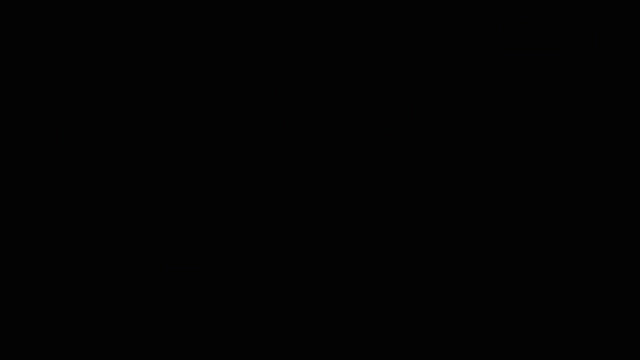 this particular mixed number. Now it helps to know the common values of some fractions. 1 over 2 is .5. 1 over 3 is .3. repeating 1 over 4 is .25. 1 over 5 is .20. 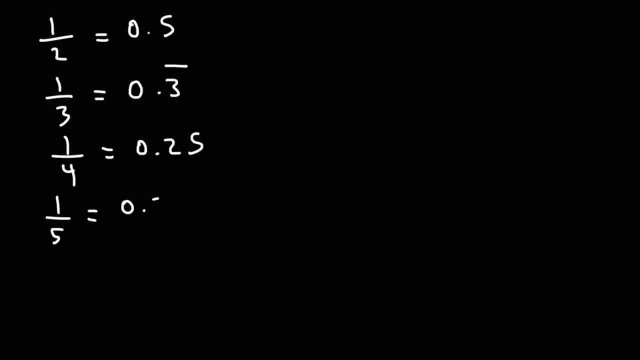 One over five is point twenty or point two. One over eight is point one, two, five And one over ten is point one. If you know those, then you can quickly find the value of other fractions. And one over twenty is point zero, five. 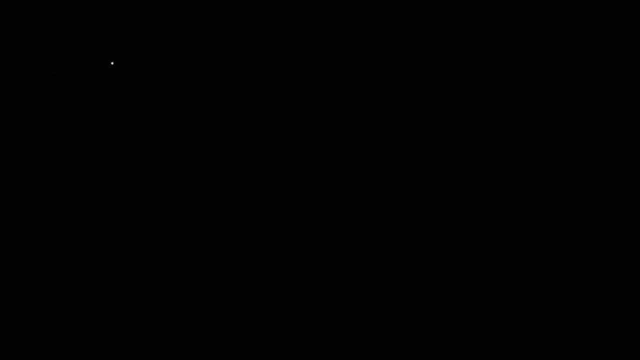 So for instance, let's say, if we want to find the value of three over four, Three over four is three times one fourth. And we know one over four is point two, five. So three times point two, five Is point seven, five. 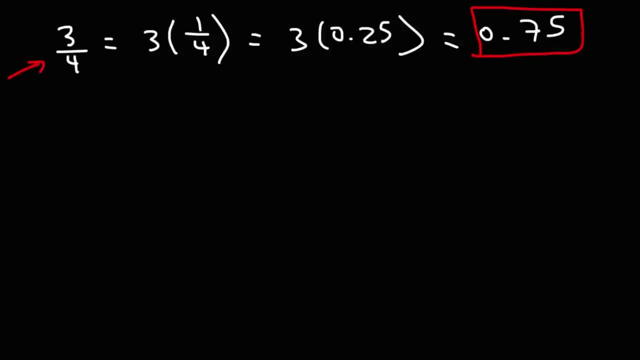 So that's a quick and simple way to convert this into a decimal. if you want to avoid long division, Let's try another example. Let's say, if we want to find the value of four over five, This is four times one over five. 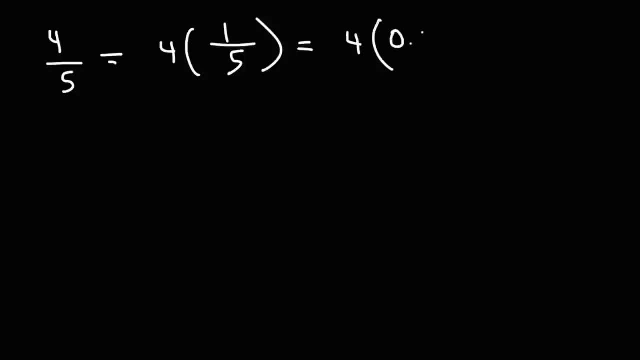 Now, if you remember that one over five is point two or point twenty, And four times point two is point eight. So four over five is point eight. Now let's say if we want to find the value of five And let's say three tenths. 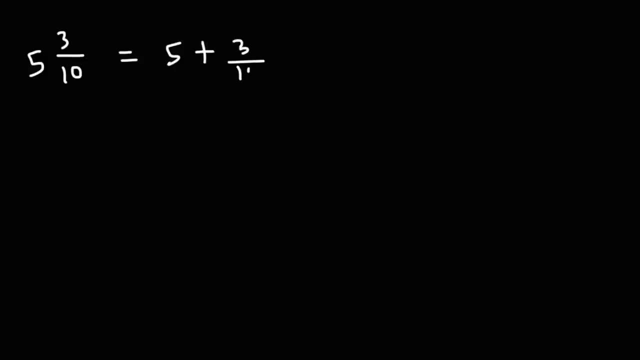 This is going to be five plus three over ten And three over ten. we can write that as three times: one over ten. One over ten is point one. Three times point one is point three. So we have five plus point three, Which is five point three. 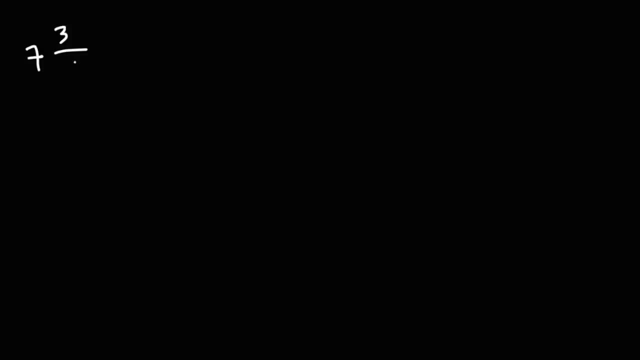 Now let's try another example. Let's say we have seven and three eighths. Go ahead and convert that mixed number into a decimal. This is going to be seven plus three over eight. We're going to write this as seven plus three times one over eight. 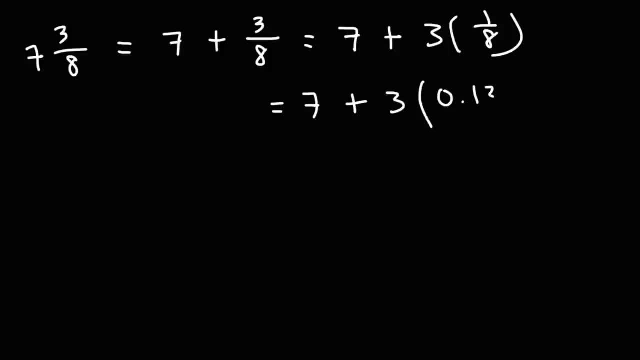 And one over eight as a decimal. if you remember, it's point one, two, five, Three times point one. two, five, Three times point one is point three, And twenty five times three is seventy five. So this is going to be point three, seven, five. 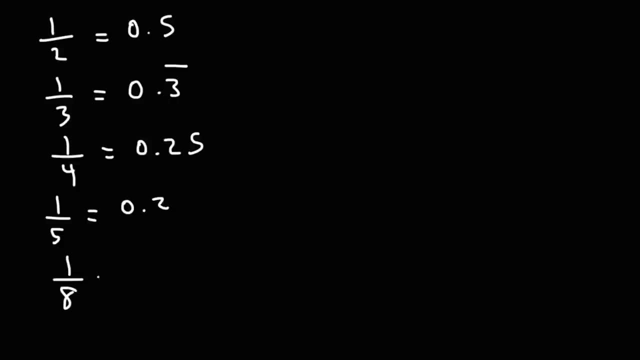 or .2. 1 over 8 is .125 and 1 over 10 is .1.. If you know those, then you can quickly find the value of other fractions. And 1 over 20 is .05.. So for instance, let's say: if we want to, 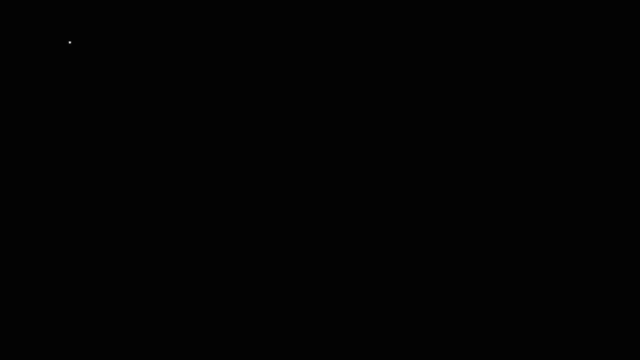 find the value of 3 over 4.. 3 over 4 is 3 times 1. fourth, And we know 1 over 4 is .25.. So 3 times .25 is .75.. So that's a quick and simple way to convert. 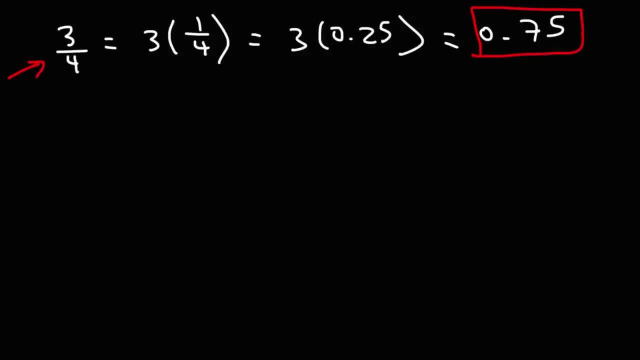 this into a decimal. if you want to avoid long division, Let's try another example. Let's say, if we want to find the value of 4 over 5. This is 4 times 1 over 5.. Now, if you remember that, 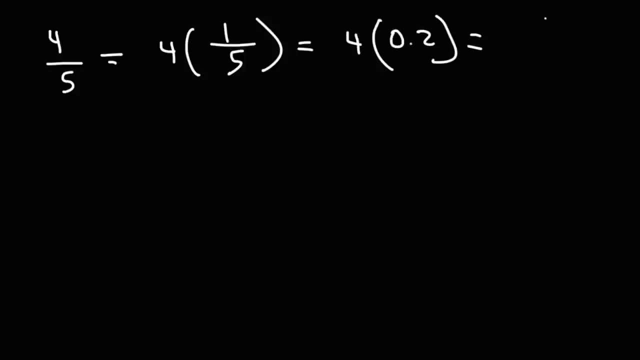 1 over 5 is .2 or .20, and 4 times .2 is .8.. So 4 over 5 is .8.. Now let's say, if we want to find the value of 5, and let's say 3 tenths. 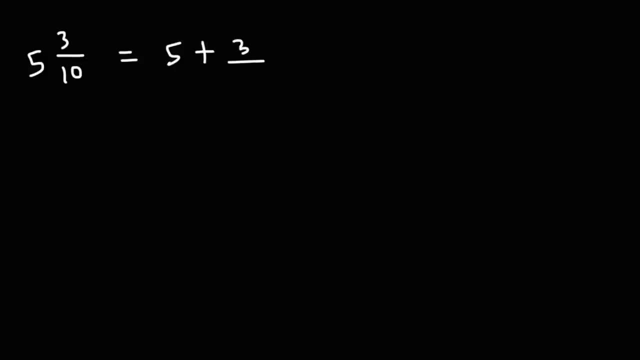 This is going to be 5 plus 3 over 10.. And 3 over 10, we can write that as 3 times 1 over 10.. 1 over 10 is .1.. 3 times .1 is .3.. 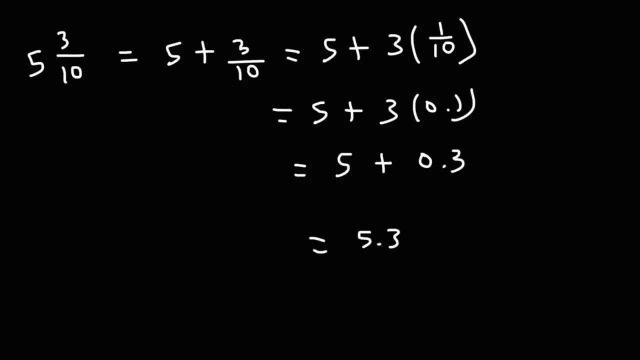 So we have 5 plus .3, which is 5.3.. Now let's try another example. Let's say we have 7 and 3 eighths. Go ahead and convert that mixed number into a decimal. This is going to be 7. 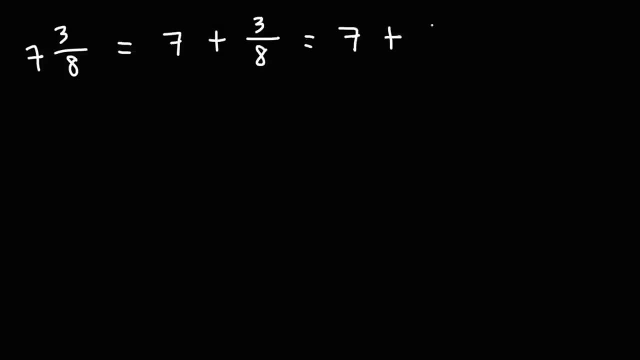 plus 3 over 8.. We're going to write this as 7 plus 3 times 1 over 8.. And 1 over 8 as a decimal. if you remember, it's .125.. 3 times .125.. 3 times .1 is .3.. 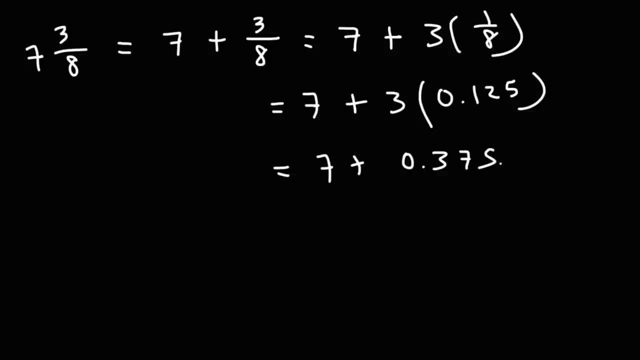 And 25 times 3 is 75.. So this is going to be .375.. So this is the value of 7 and 3 eighths, It's 7.375.. So that's a quick and simple way to convert. 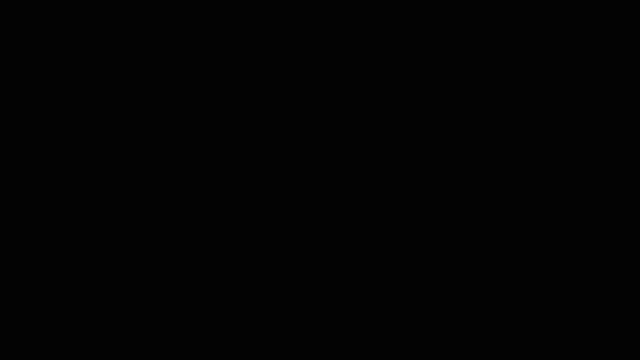 common fractions into decimals. Now sometimes you need to be able to convert a percentage into a decimal. So, for instance, how would you convert 75% into a decimal? You can actually either divide 75 by 100 or move the decimal to units. to the left. 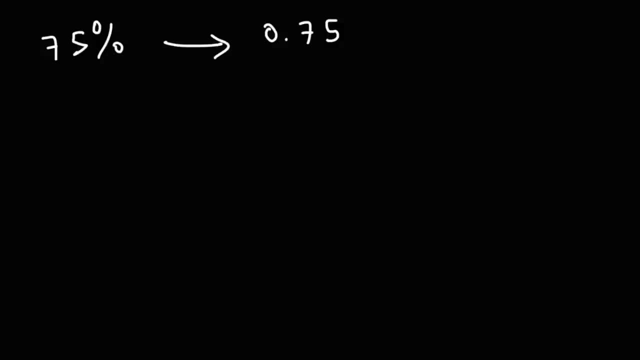 Either case, it's .75.. So, with that in mind, go ahead and convert these values, these percentages, into decimals: 146%, 67%, 15%, 8%, 4.2%, and let's say .25.. .56%. 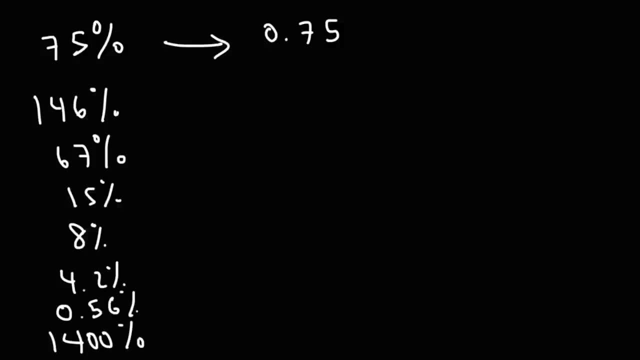 And then 1400%. Go ahead and convert those percentages into decimals. So if we move the decimal .2 units to the left, this is going to be 1.46.. 67% is .67.. 15% is .15.. 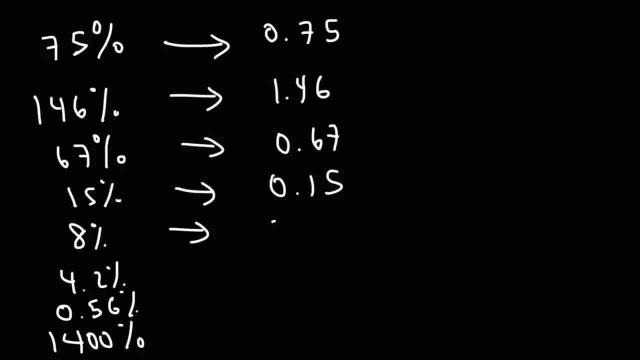 8%. if you move it 2 to the left or divide 8 by 100, you're going to get .08.. 4.2% is .042.. .25.. .56%, That's .0056.. 1400%. 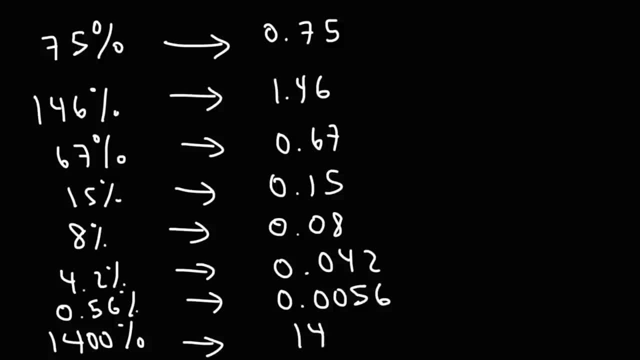 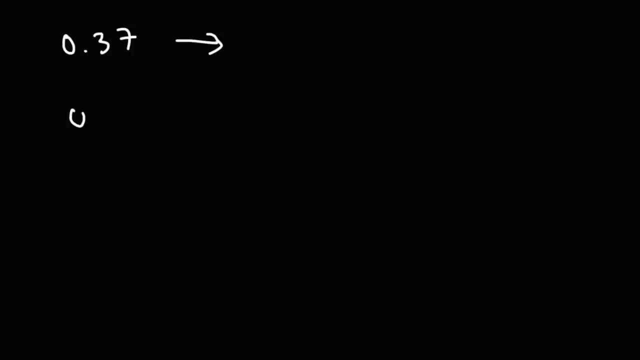 If you move it 2 units to the left, that is the decimal point you get 14.. So that's how you can convert a percentage into a decimal value. Now go ahead and convert the following decimal values into percentages In order to convert a decimal back to a percentage: 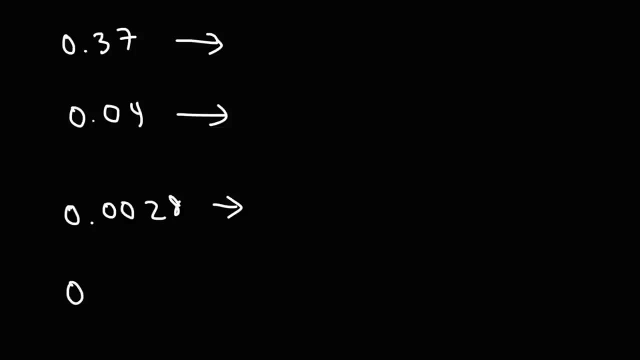 multiply by 100, or move the decimal point 2 units to the right. So .37 is 37%, .04 is 4%- .0028,. if you multiply that by 100, you're going to get .28%- .468,. 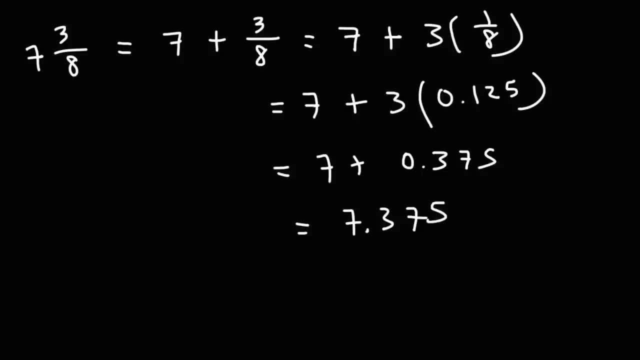 So this is the value of seven and three eighths. It's seven point three seven five. So that's a quick and simple way to convert common fractions into decimals. Now, sometimes you need to be able to convert a percentage into a decimal. 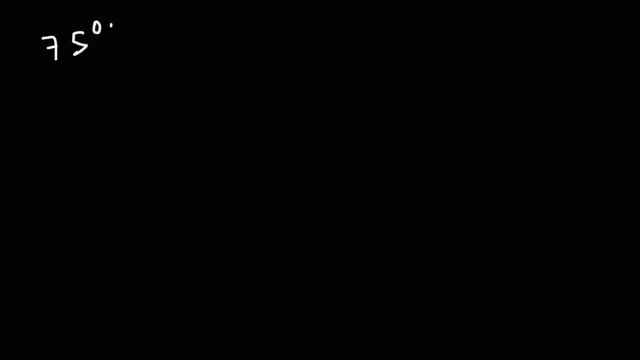 So, for instance, How would you convert seventy five percent into a decimal? You can either divide seventy five by a hundred or move the decimal to units to the left. Either case, it's point seven five. So, with that in mind, go ahead and convert these values, these percentages, into decimals. 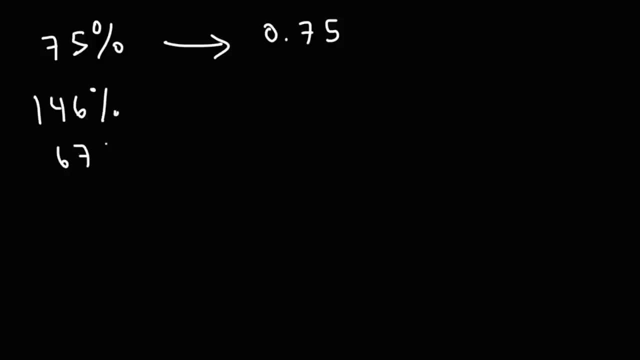 A hundred forty six percent, Sixty seven percent, Fifteen percent, Eight percent, Four point two percent, And let's say point fifty six percent, And then fourteen hundred percent. Go ahead and convert those percentages into decimals. So if we move the decimal point two units to the left, 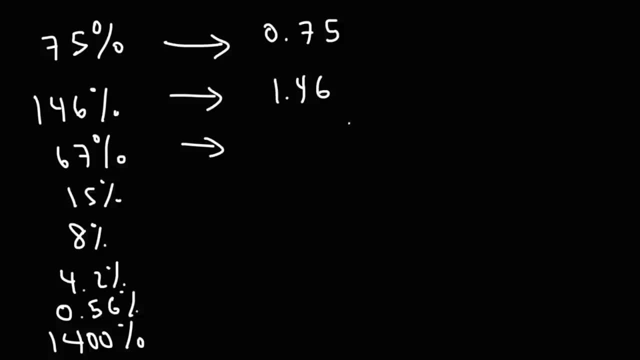 This is going to be one point four. six. Sixty seven percent is point sixty seven. Fifteen percent is point fifteen Eight percent. if you move it two to the left or divide eight by a hundred, You're going to get point zero, eight. 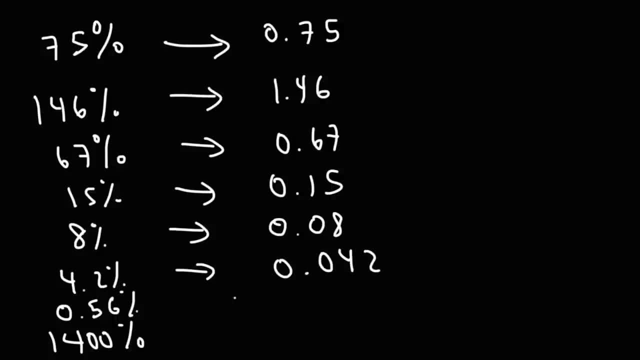 Four point two percent is point zero. four. two Point fifty six percent, That's point zero. zero. five, six, Fourteen hundred percent. If you move it two units to the left, That is the decimal point, You get fourteen. So that's how you can convert a percentage into a decimal value. 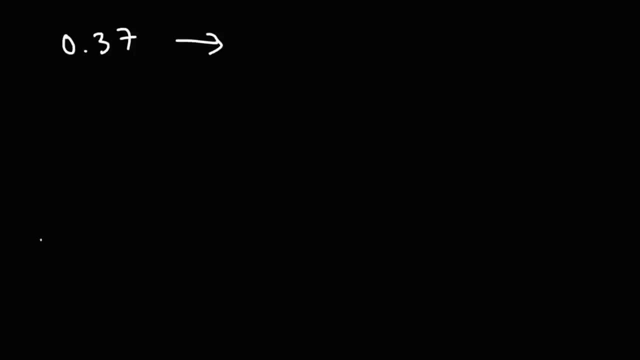 Now go ahead and convert The following decimal values into percentages. In order to convert a decimal back to a percentage, Multiply by a hundred Or move the decimal point two units to the right. So point three seven is thirty seven percent. Point zero four is four percent. 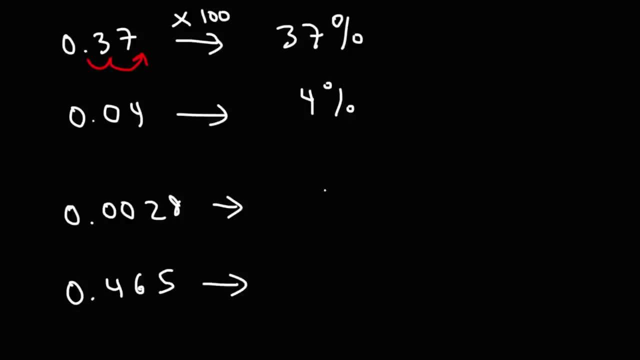 Point zero, zero, two, eight. If you multiply that by a hundred, You're going to get point twenty eight percent. Point four, six, five, That's forty six point five percent. So that's how you can Interconvert between decimal values and percentages. 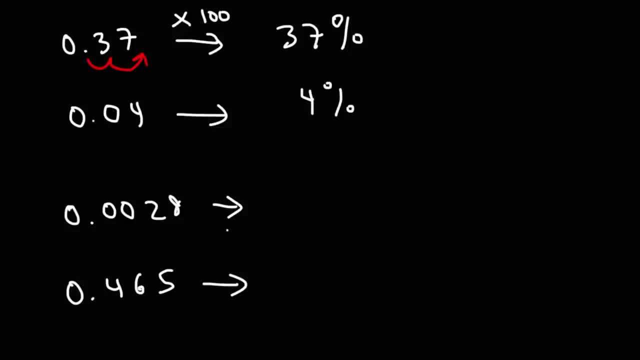 you're going to get .268.. .268,, you're going to get .268.. .268,, you're going to get .268.. .265, that's 46.5%. So that's how you can interconvert between decimal values and percentages. 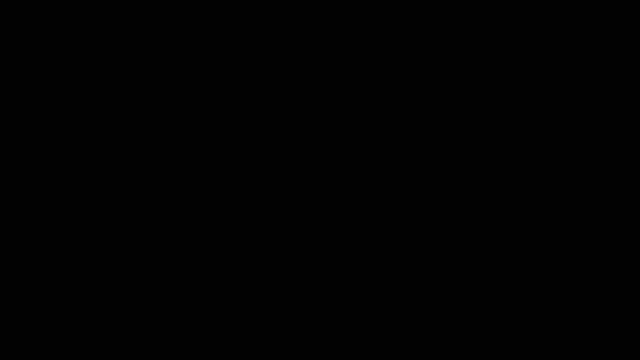 But now let's talk about how we can convert a decimal number into a fraction. So let's say we have .2.. We know that .2 is 1 over 5.. But how can we show our work to convert this decimal value into a fraction? 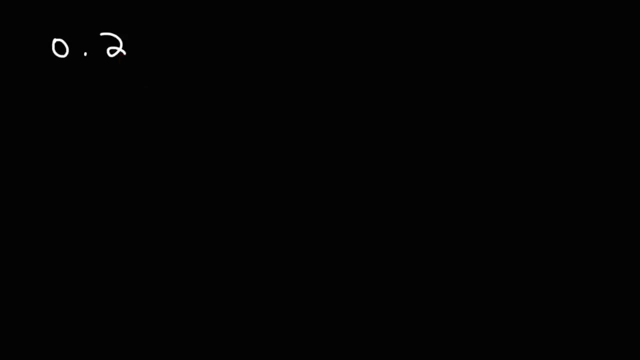 So notice that this is rounded to the nearest tenth. Therefore, put it over 1, and multiply the top and bottom by 10.. .2 times 10 is 2., And 1 times 10 is 10.. And then all you've got to do 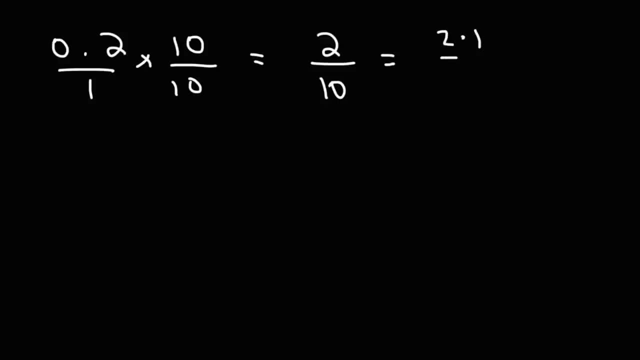 is reduce the fraction. 2 is 2 times 1.. 10 is 2 times 5.. So we can cancel the 2, and we're going to get 1 over 5.. So 1 over 5 is .2.. 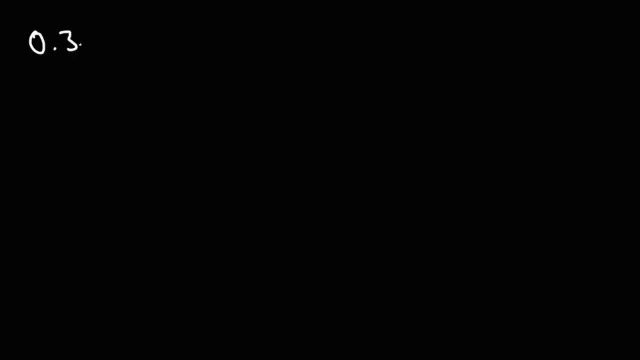 Go ahead and try this one. Convert .3 into a fraction, So we're going to put this over 1, and multiply the top and bottom by 10.. .3 times 10 is 3.. 1 times 10 is 10.. 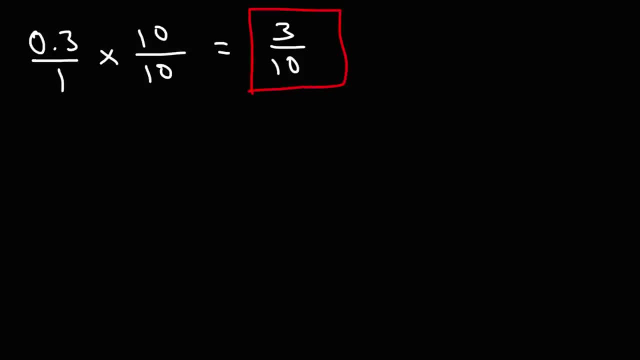 And we can't reduce this fraction, so it's simply 3 over 10.. Now, what about this one, .24? How can we convert that into a fraction? So, like before, we're going to put this over 1.. But notice that .24. 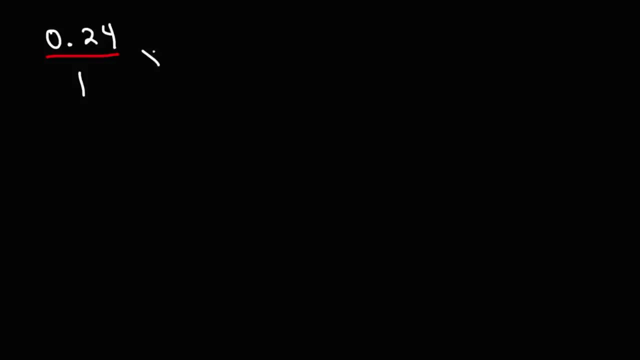 is rounded to the nearest hundredth. So to get rid of the decimal we need to multiply it by 100. this time, That is 100 over 100.. .24 times 100.. Whenever you multiply a number by 100, move the decimal 2 units to the right. 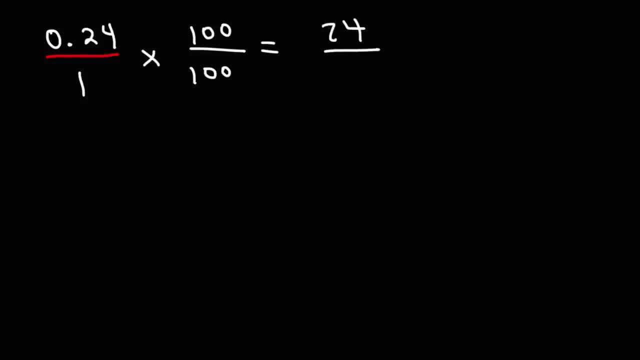 So this becomes 24.. On the bottom we have 1 times 100, which is 100.. So now all we need to do is reduce the fraction So 24, we can write that as 4 times 6.. 100 is 4 times 25.. 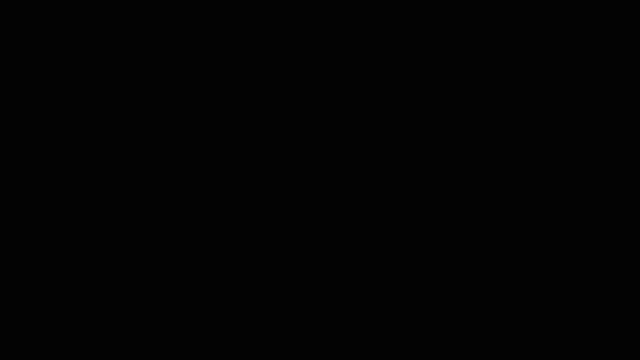 But now let's talk about how we can convert A decimal number into a fraction. So let's say we have point two, We know that point two is one over five, But how can we show our work to convert this decimal value Into a fraction? 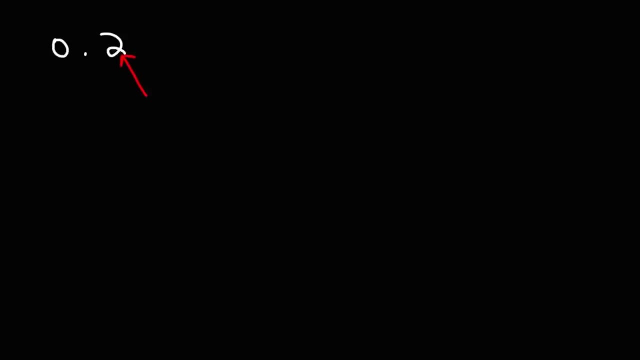 So notice that this is rounded to the nearest tenth. Therefore, put it over one And multiply the top and bottom by ten. Point. two times ten is two, And one times ten is ten, And then all you got to do is reduce the fraction. 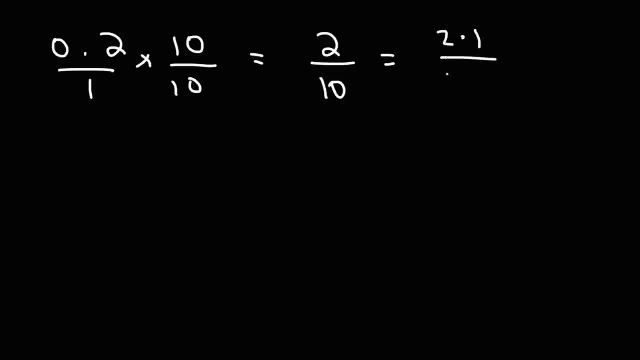 Two is two times one, Ten is two times five. So we can cancel the two And we're going to get one over five. So one over five is point two. Go ahead and try this one. Convert point three Into a fraction. 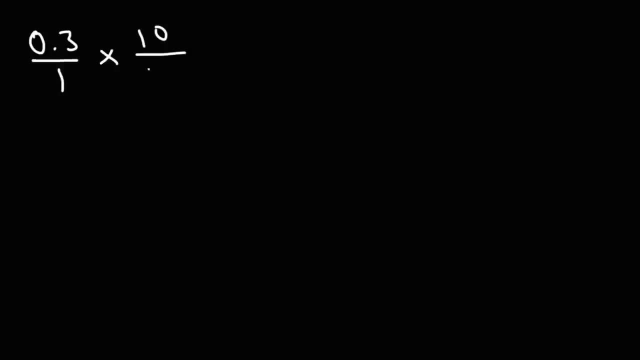 So we're going to put this over one And multiply the top and bottom by ten. Point. three times ten is three, One times ten is ten, And we can't reduce this fraction. So it's simply three over ten. Now what about this one? 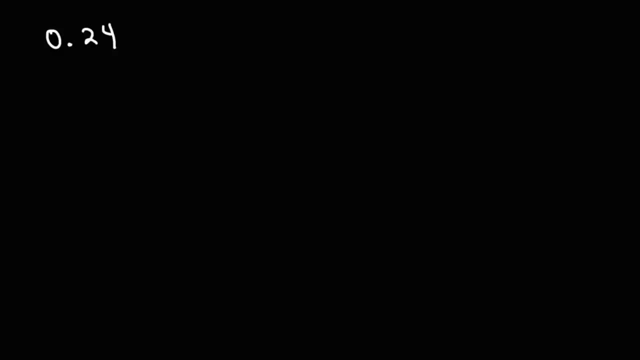 Point twenty four. How can we convert that into a fraction? So, like before, we're going to put this over one. But notice that point twenty four is rounded to the nearest hundredth. So to get rid of the decimal We need to multiply it by a hundred this time. 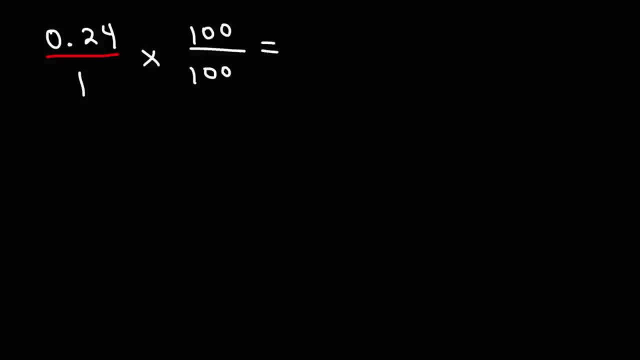 That is a hundred over a hundred. Point twenty four times a hundred. Whenever you multiply a number by a hundred, Move the decimal two units to the right, So this becomes twenty four. On the bottom we have one times a hundred, Which is a hundred. 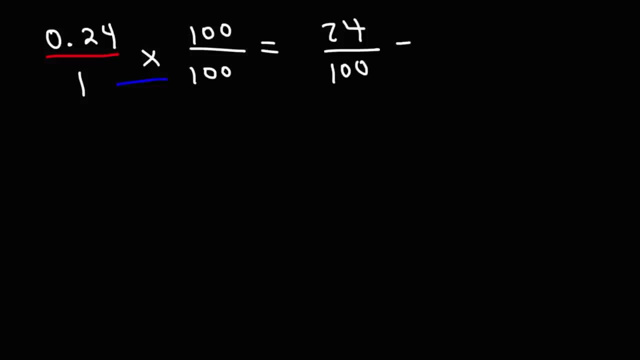 So now all we need to do is reduce the fraction So twenty four. we can write that as four times six. A hundred is four times twenty five. We can cancel the four And we're left with our final answer, Which is six over twenty five. 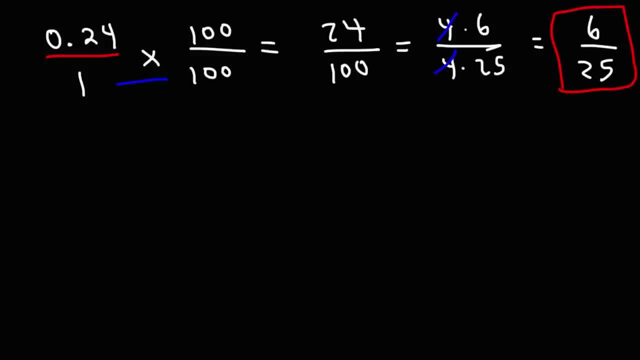 So that's how we can convert point twenty four into a fraction. Try this: one. Point thirty six. So let's put this over one And let's multiply By a hundred over a hundred. So point thirty six times a hundred Is thirty six. 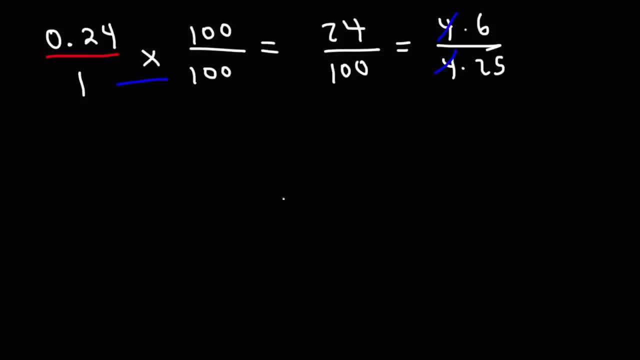 We can cancel the 4, and we're left with our final answer, which is 6 over 25.. So that's how we can convert .24 into a fraction. Try this one: .36. So let's put this over 1.. 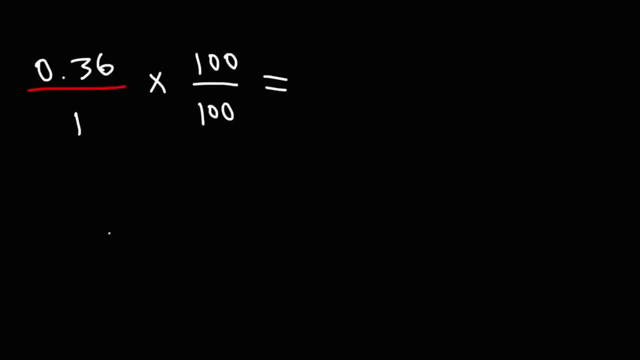 And let's multiply by 100 over 100.. So .36 times 100 is 36., And then 1 times 100 is 100.. And now, how should we break up these numbers? Well, 36,. we can write that as: 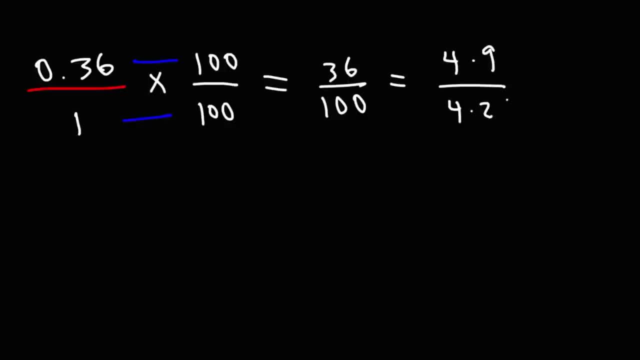 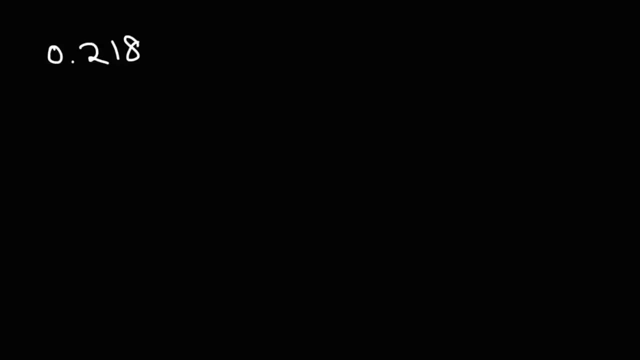 Now what about .218?? What is .218 as a fraction? What is .218 as a fraction? Now? this time this one is rounded to the nearest thousandth, So we're going to multiply it by 1000 over 1000. 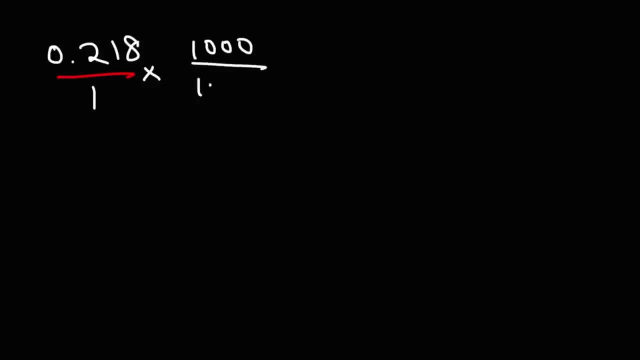 by 1000 over 1000 to get rid of the decimal. .218 times 1000 is 218.. And 1 times 1000 is 1000.. Now if you're not sure how to break up the numbers, if they're both even, you could simply: 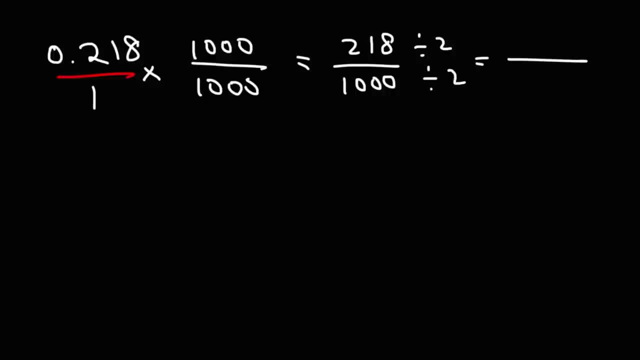 divide by 2.. What's half of 218?? Half of 200 is 100.. Half of 18 is 9. So that's 109.. Half of 1000 is 500.. And we can't reduce it any further. 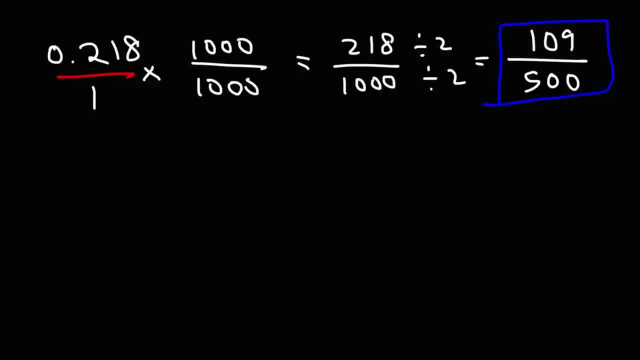 than this. So the answer is 109 over 500.. So the answer is 109 over 500.. Now let's try another example. Now let's try another example .314. Go ahead and convert that into a fraction. So, just like before. 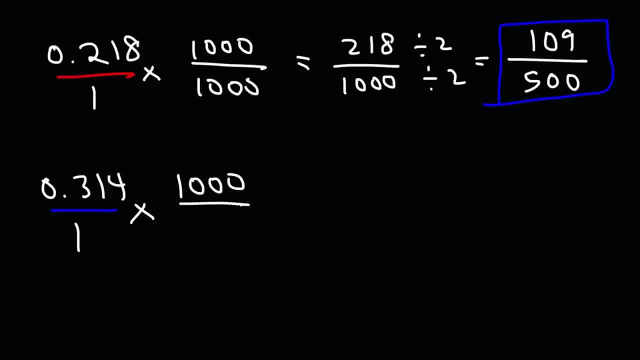 we're going to multiply by 1000 over 1000.. .314 times 1000 is 314.. is 314.. Now let's divide by 2.. Half of 314. 314 divided by 2 is 157.. 300 divided by 2. 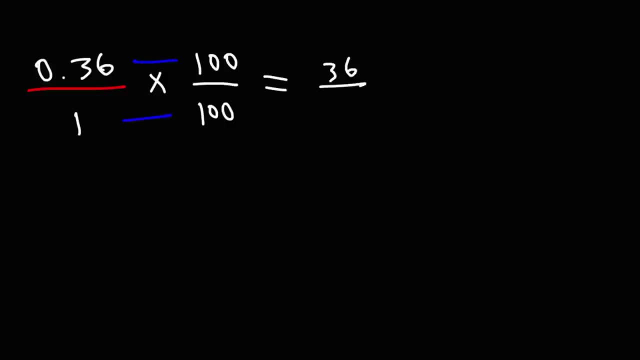 And then one times a hundred is a hundred. And now, how should we break up these numbers? Well, thirty six, We can write that as four times nine. A hundred, We can write that as four times twenty five. So the final answer is going to be nine over twenty five. 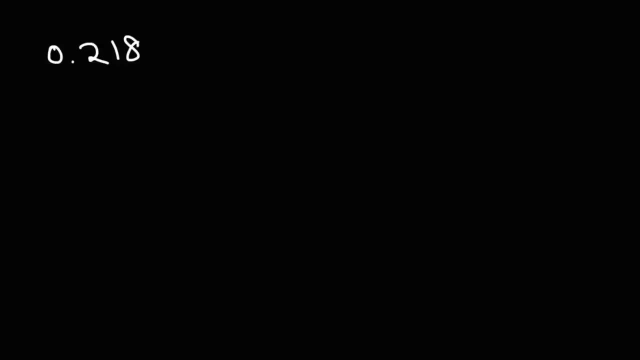 Now what about point two, one eight. What is point two? one eight as a fraction? Now, this time This one is rounded to the nearest thousandth, So we're going to multiply it By a thousand over a thousand To get rid of the decimal. 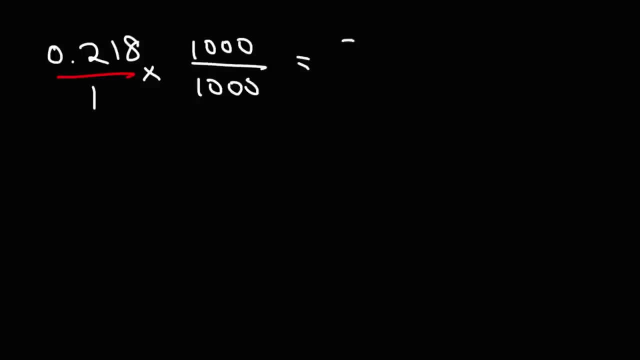 Point two: one eight times a thousand is two hundred eighteen, And one times a thousand is a thousand. Now, if you're not sure how to break up the numbers, If they're both even, you could simply divide by two. What's half of two eighteen? 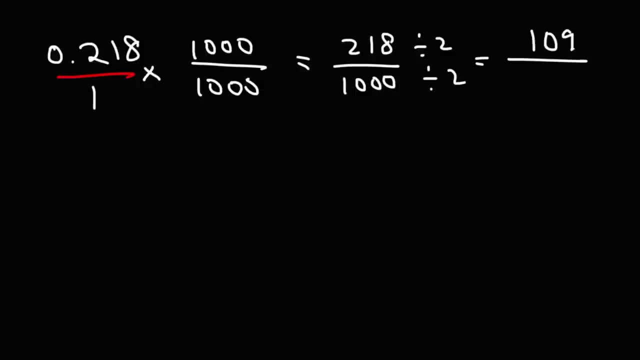 Half of two hundred is a hundred. Half of eighteen is nine, So that's one, oh nine. Half of a thousand is five hundred, And we can't reduce it any further than this. So the answer is a hundred and nine over five hundred. 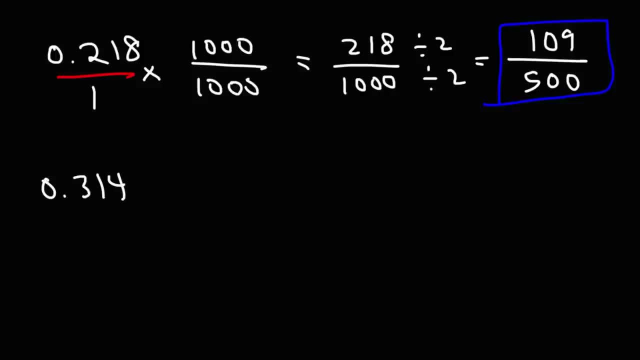 Now let's try another example: Point three, one, four. Go ahead and convert that into a fraction. So, just like before, we're going to multiply By a thousand over a thousand. Point three, one, four times a thousand is three hundred fourteen. Now let's divide by two. 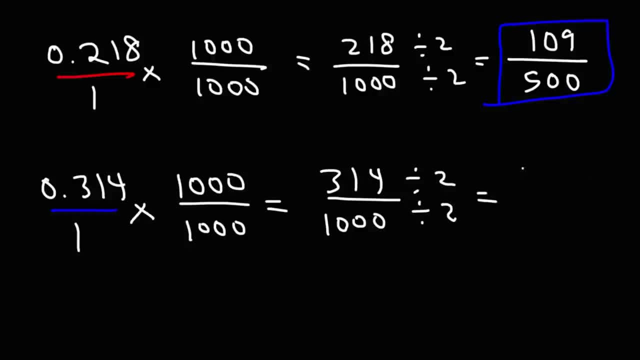 Half of three, fourteen, Three. fourteen divided by two is one fifty seven. Three hundred divided by two is one fifty, And then fourteen divided by two is seven. When you add one, fifty and seven, you get one fifty seven. And we know half of a thousand is five hundred. 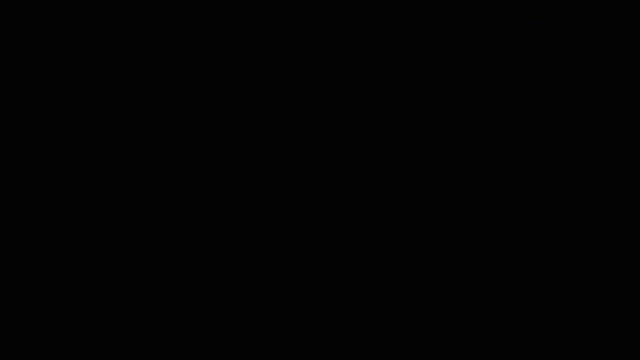 So this is going to be one fifty seven over five hundred. Now, how would you convert point two, repeating, into a fraction? Now, this goes on forever. This is point two, two, two, two, two, two, and it keeps on going. How would you convert that into a fraction? 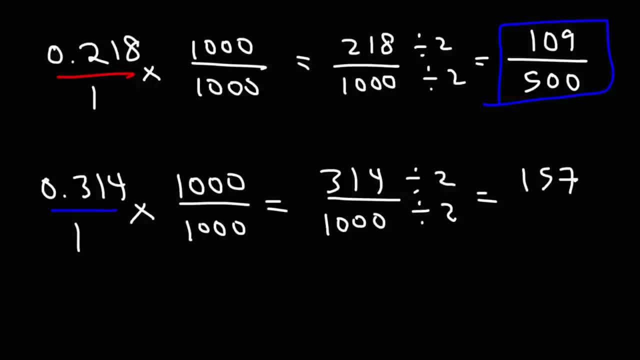 is 150. And then 14 divided by 2 is 7.. When you add 150 and 7, you get 157. And we know half of 1000 is 500. So this is going to be 157 over 500.. 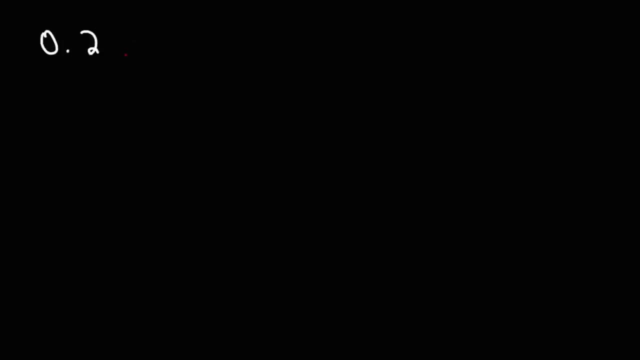 Now how would you convert .2 repeating into a fraction? Now, this goes on forever. This is .222222 and it keeps on going. How would you convert that into a fraction? .2 repeating is simply 2 over 9.. .4 repeating. 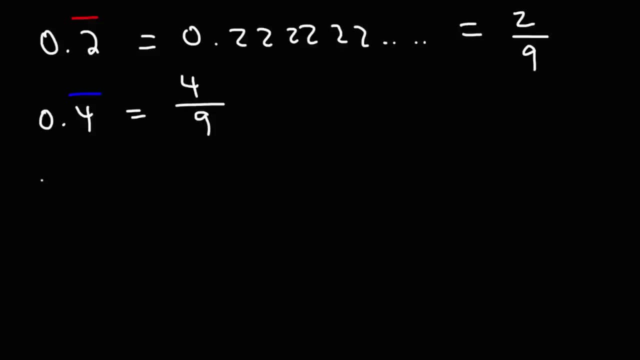 is simply 4 over 9.. .5- repeating is simply 5 over 9.. .3- repeating this one is 3 over 9, but you can reduce it If you divide by 3, top and bottom, this becomes 1 over 3.. 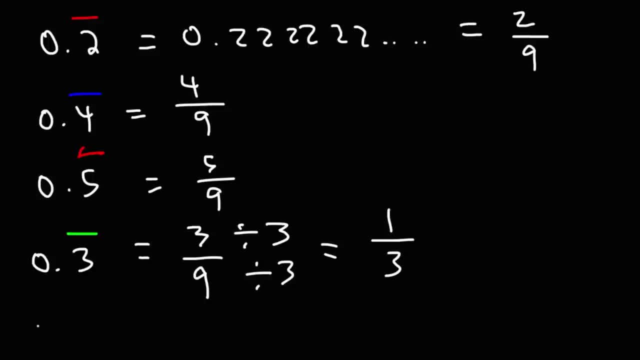 So .3- repeating- is 1 over 3.. .6- repeating this initially is 6 over 9, but you can reduce that 6 is 2 times 3.. 9 is 3 times 3.. So if you cancel a 3,, 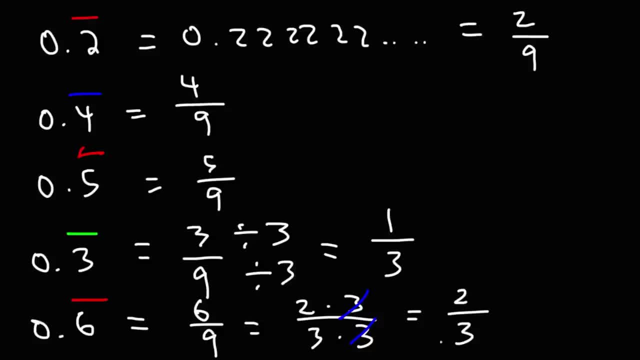 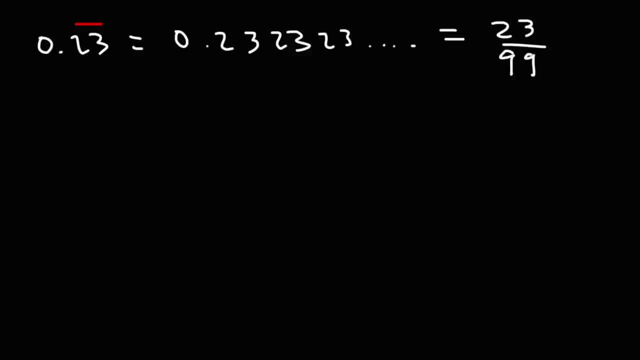 .6 repeating reduces to 2 over 3.. Now what about .23 repeating? So this is .23,, 23,, 23 and so forth. This is 23 over 99.. .36 repeating: this is 36 over 99.. 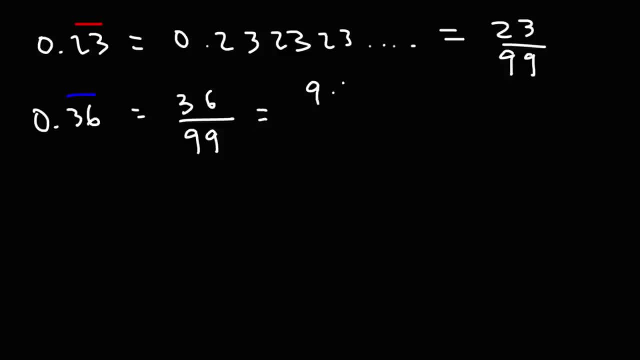 But this one we can simplify: 36 is 9 times 4.. 99 is 9 times 11.. So we can cancel a 9.. Thus, .36 repeating reduces to 4 over 11.. Now, what about this one? 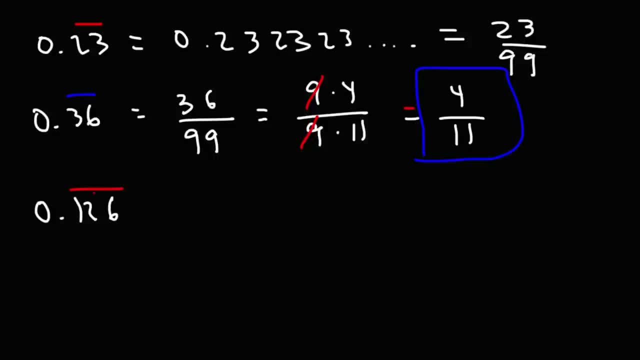 .126 repeating. What can we do with that? So here we have 3 numbers that are repeating. This is going to be 126 over 999.. Now how can we reduce 126 over 999? 126 is divisible by 3.. 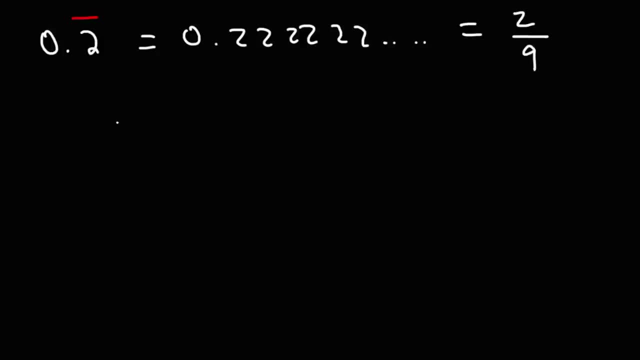 Point two, repeating, is simply two over nine. Point four, repeating, is simply four over nine. Point five, repeating, is simply five over nine. Point three, repeating This one, is three over nine, but you can reduce it If you divide by three The top and bottom. 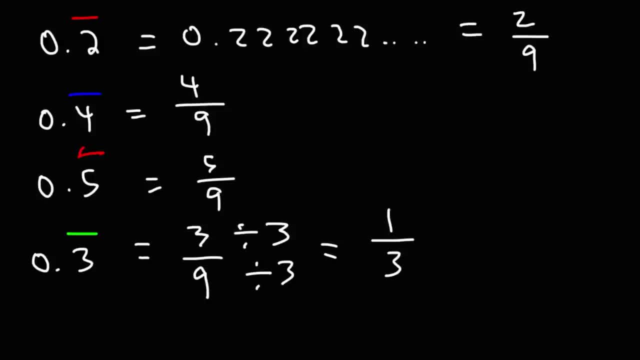 This becomes one over three. So point three, repeating, is one over three. Point six: repeating This initially is six over nine. But you can reduce that Six is two times three, Nine is three times three. So if you cancel with three, 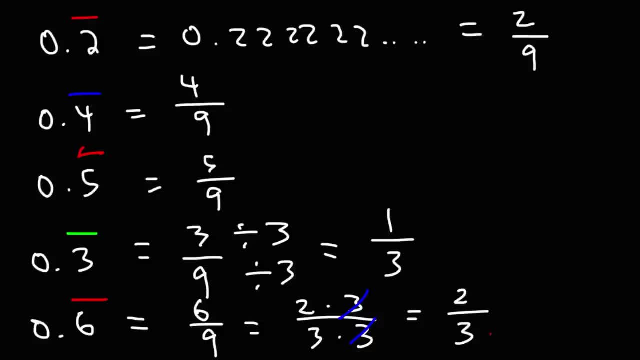 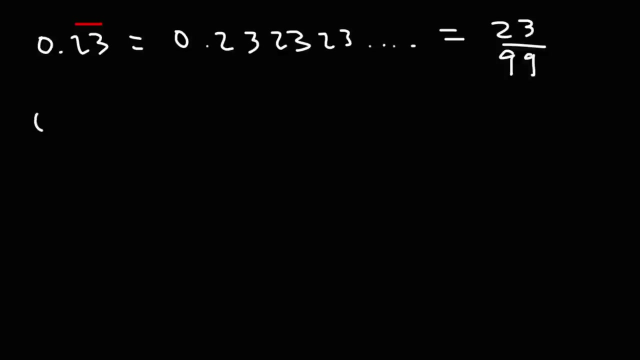 Point six, repeating reduces to two over three. Now, what about point twenty three, repeating? So this is point two, three, Two, three, Two, three and so forth. This is twenty three over ninety nine. Point three six, repeating: This is thirty six over ninety nine. 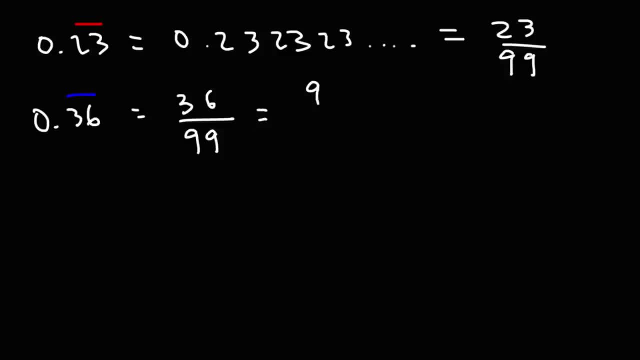 But this one we can simplify. Thirty six is nine times four. Ninety nine is nine times eleven, So we can cancel a nine. Thus point three. six repeating reduces to four over eleven. Now, what about this? one Point one, two, six repeating. 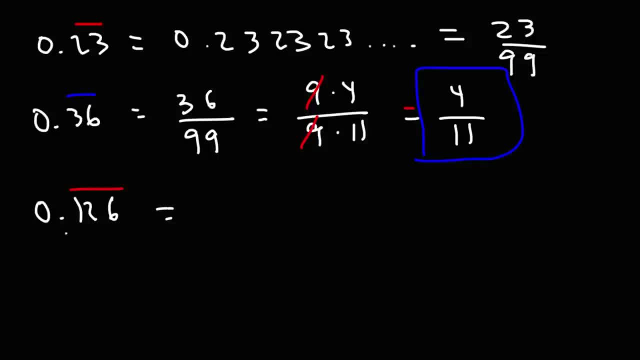 What can we do with that? So here we have three numbers that are repeating. This is going to be a hundred twenty six over nine hundred ninety nine. Now how can we reduce one twenty six over nine nine nine? One twenty six is divisible by three. 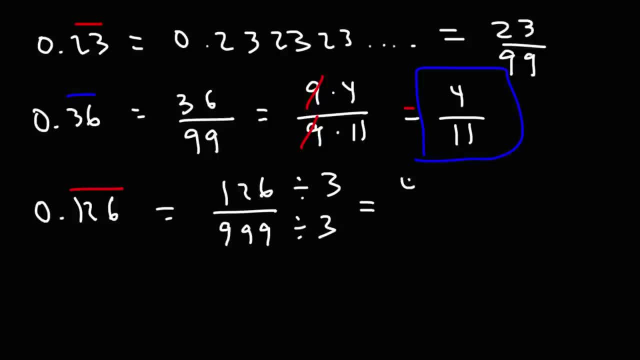 A hundred twenty divided by three, Or twelve divided by three is four. Six divided by three is two. So one twenty six divided by three is forty two. Nine hundred ninety nine divided by three is three hundred thirty three, And it turns out that we can divide both numbers by three again. 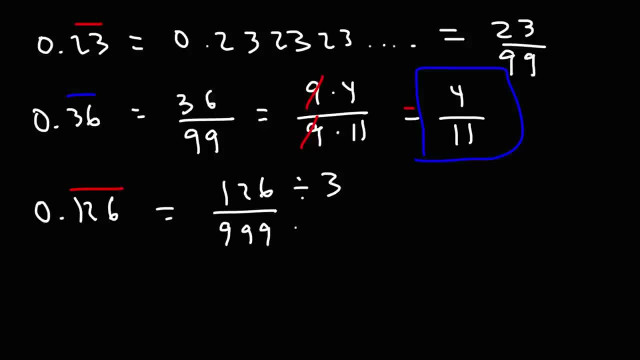 120 divided by 3, or 12 divided by 3 is 4.. 6 divided by 3 is 2.. So 126 divided by 3 is 42.. 999 divided by 3 is 333.. And it turns out that 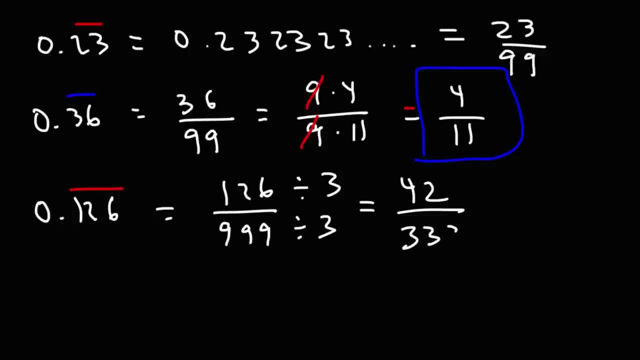 we can divide both numbers by 3 again: 42 divided by 3 is 999. divided by 3 is 333.. 42 divided by 3 is 14.. 333 divided by 3 is 111.. So the final answer. 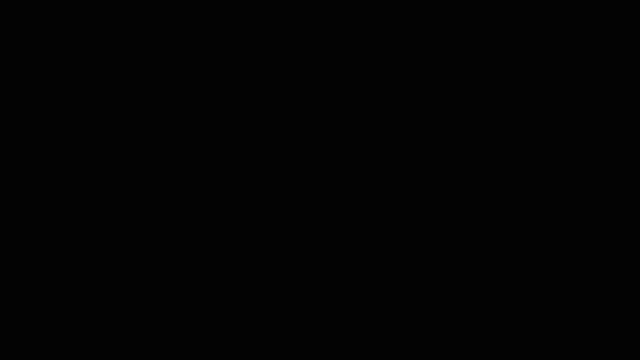 is 14 over 111.. Let's try another one like that. Let's reduce .315, repeating, So first we can write this as 315 over 999.. 300 is divisible by 3, and so is 15.. Therefore 315 must be. 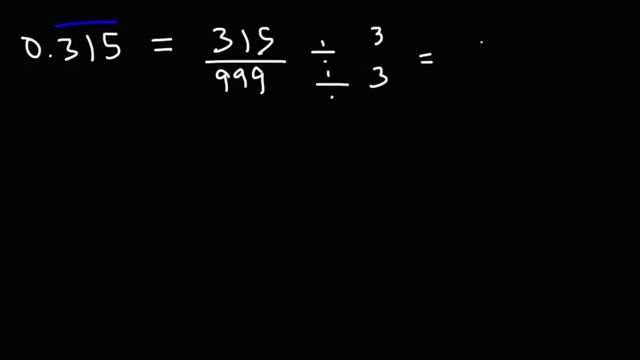 divisible by 3.. 300 divided by 3 is 100.. 15 divided by 3 is 5.. So 315 divided by 3 is 105.. And we know this is going to be 333.. Now, 105,. 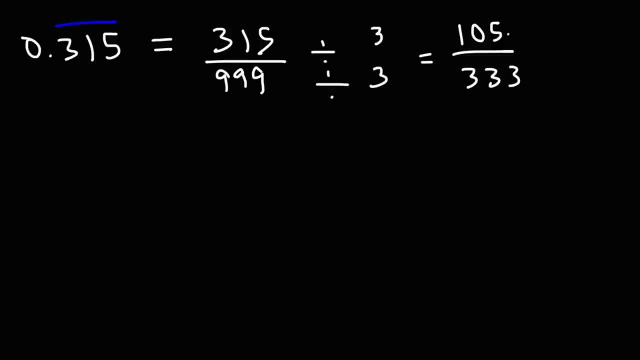 what can we do with that? 105 is also divisible by 3.. 105 divided by 3 is 35.. 333 divided by 3 is 111.. And this is as far as we can go for this example. So it's. 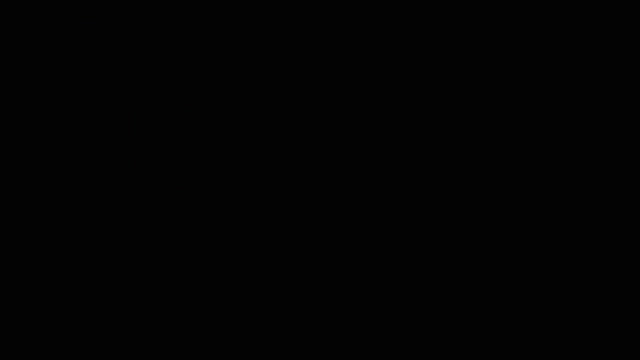 35 over 111.. Now what about this one? .43.. But only the 3 is repeating, So this is .433333.. How can we turn that into a fraction? Well, we need to separate the repeating decimal from the non-repeating part. 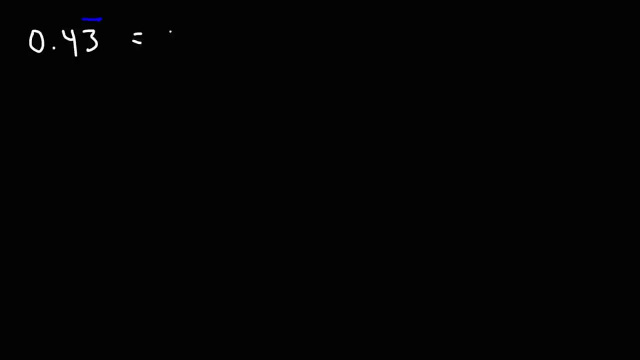 To do that subtract Let's add a few 3's. So this is going to be .33333 plus another number. This is the repeating part. What is the other number? The other number has to be .1.. .3 repeating plus .1 is: 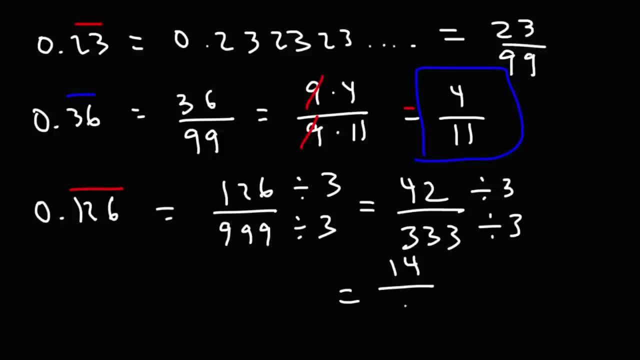 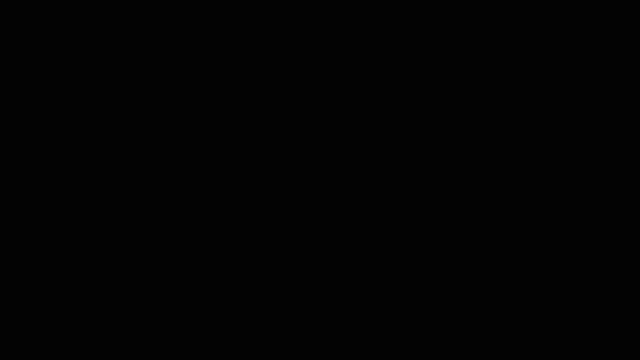 Forty two divided by three is fourteen. Three hundred thirty three divided by three is one eleven. So the final answer is fourteen over one eleven. Let's try another one like that. Let's reduce point three one, five, repeating. So first we can write this as three hundred fifteen over nine, nine, nine. 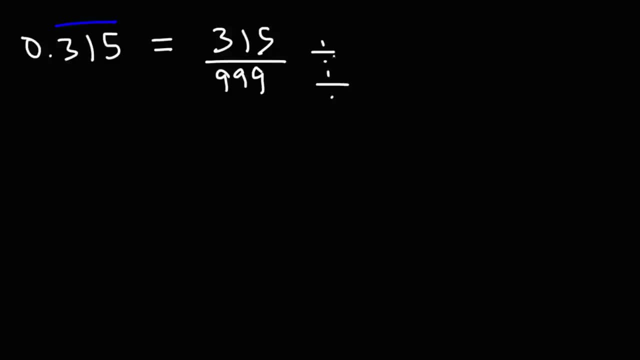 Three hundred is divisible by three, and so is fifteen. Therefore, three fifteen must be divisible by three. Three hundred divided by three is a hundred. Fifteen divided by three is five. So three fifteen divided by three is one, oh five. And we know this is going to be three hundred thirty three. 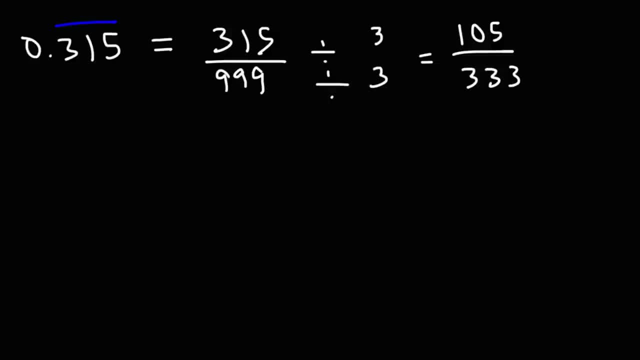 Now one oh five. what can we do with that? One oh five is also divisible by three. One oh five divided by three is thirty five. Three thirty three divided by three is one eleven. And this is as far as we can go for this example. 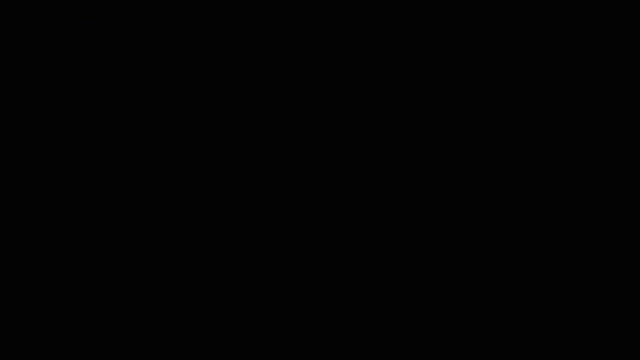 So it's thirty five over one eleven. Now what about this one? Point four, three. But only the three is repeating. So this is point four: three, three, three, three, three. How can we turn that into a fraction? Well, we need to separate the repeating decimal from the non-repeating part. 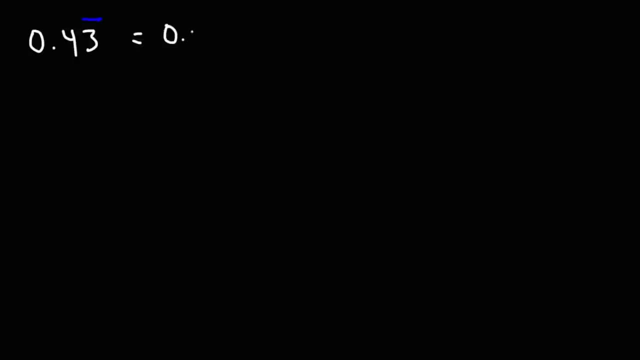 To do that subtract, Let's add a few threes. So this is going to be point three: three, three, three, three plus another number. This is the repeating part. What is the other number? The other number has to be point one. 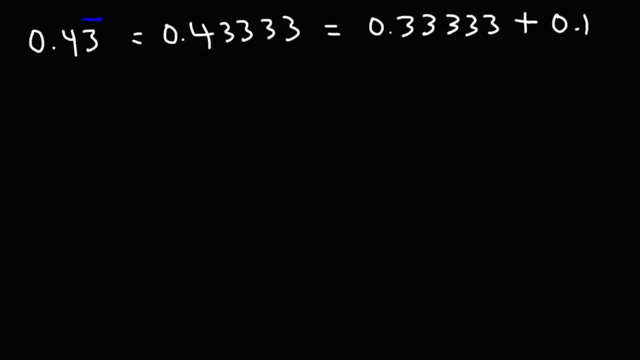 Point three repeating plus point one, is going to be point four, with three repeating, And if you add these two you're going to get this number. So another way to get this number Is to take this number and subtract it by point three, three, three, three, three. 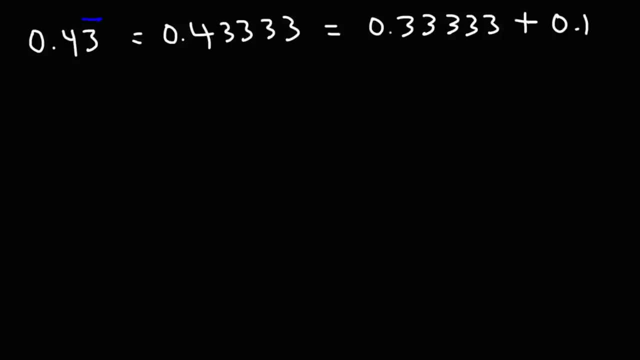 going to be .4, with 3 repeating, And if you add these two you're going to get this number. So another way to get this number is to take this number and subtract it by .33333.. And make sure you end up at the same spot. 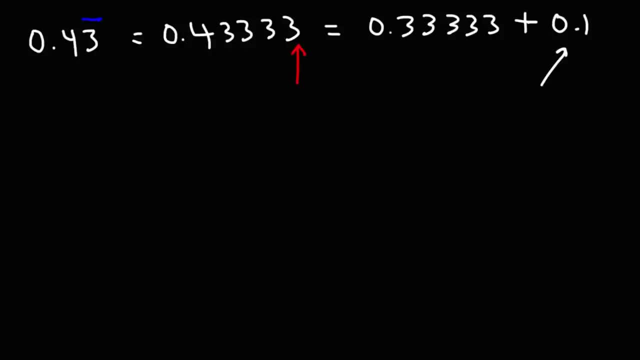 So let's say, if you round this to the 5th digit after the decimal point, you want to stop here, at the 5th digit after the decimal point, Because if you add another 3, you're not going to get .1.. 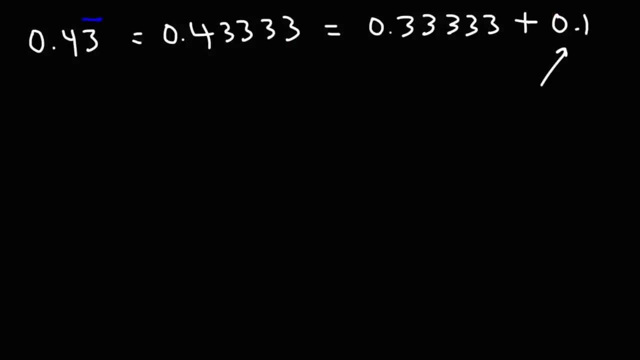 So in your calculator, if you type in .433 and then 33, and subtract that by .33333, you're going to get .1.. Now so let's write the exact values here. So .4, 3 repeating is .3 repeating. 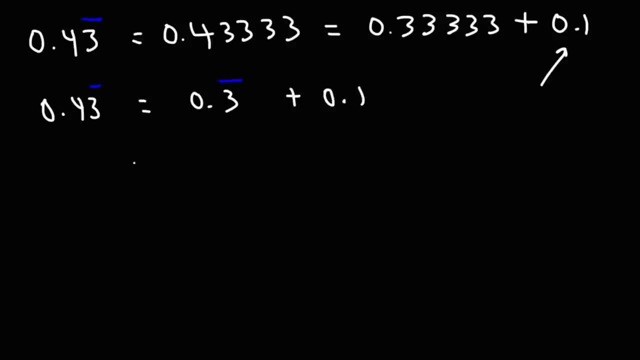 plus .1.. .3, repeating: we know it's 1 over 3.. .1,, we know it's 1 over 10.. So now we need to combine these two fractions. So let's multiply this one by 10 over 10,. 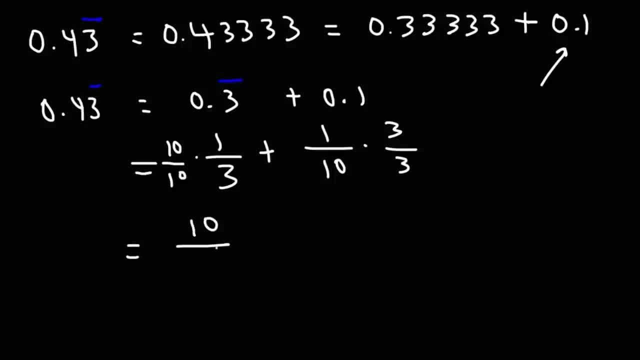 and the other one by 3 over 3.. So we get 10 over 30 plus 3 over 30. And this becomes 13 over 30. If you type this in your calculator: 13 divided by 30, you're going to get .43 repeating. 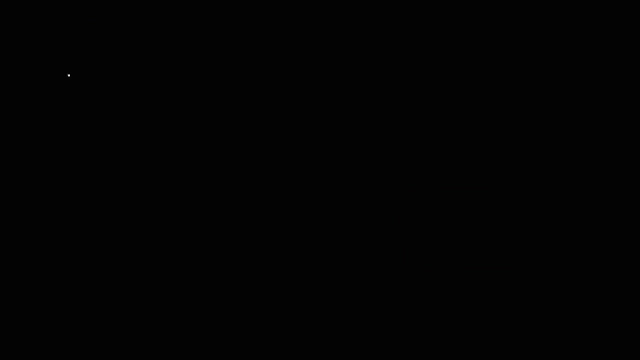 So that's how you can check your work. Let's try another example. Let's say we have .63, 23 repeating. Go ahead and convert this decimal into a fraction, So the repeating part is .23.. To find the non-repeating. 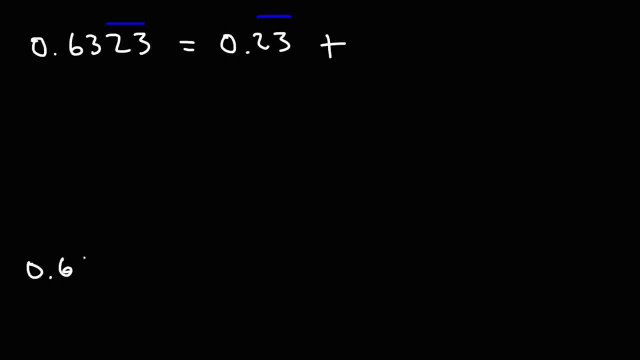 part. type this in your calculator: .6, 23, 23,, and subtract it by the repeating part, So we have a total of 6 digits after the decimal. So we're going to subtract it by .23, 23, 23,, the same number. 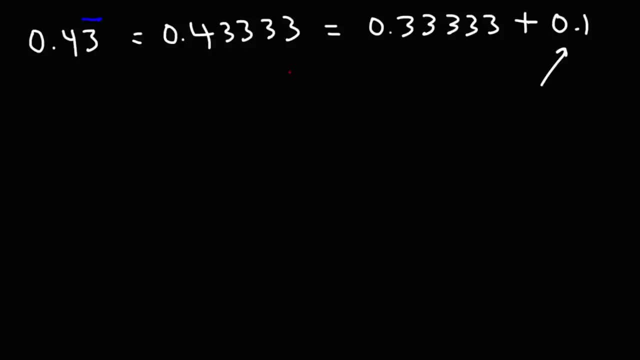 And make sure you end up at the same spot. So let's say, if you round this to the fifth digit after the decimal point, You want to stop here at the fifth digit after the decimal point, Because if you add another three you're not going to get point one. 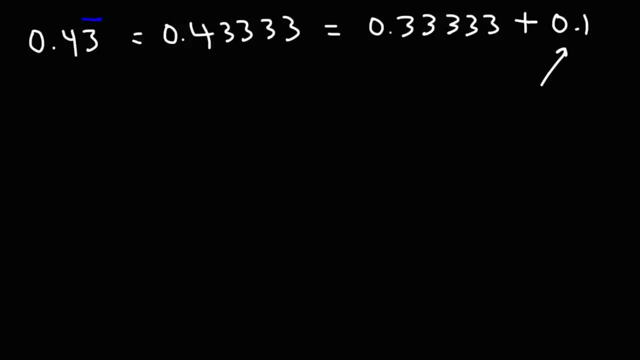 So in your calculator if you type in point four, three, three And then three, three, And subtract that by point three, three, three, three, three, You're going to get point one Now. so let's write the exact values here. So point four, three repeating is point three repeating plus point one. 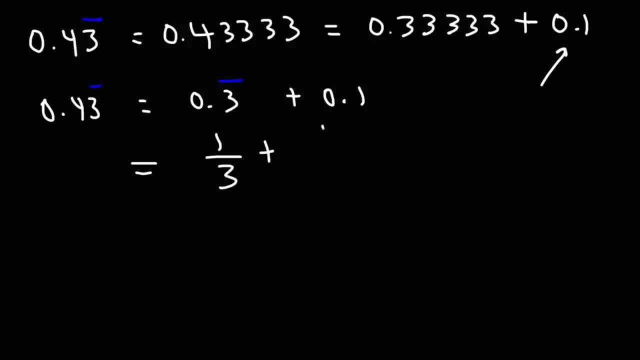 Point three, repeating: we know it's one over three. Point one: we know it's one over ten. So now we need to combine these two fractions. So let's multiply this one by ten over ten And the other one by three over three. 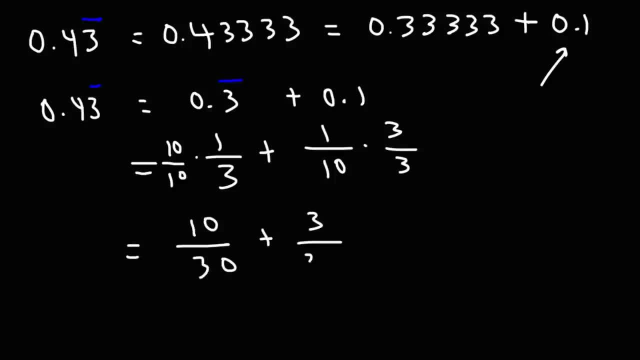 So we get ten over thirty Plus three over thirty, And this becomes thirteen over thirty. If you type this in your calculator, Thirteen divided by thirty, You're going to get point four, three repeating. So that's how you can check your work. 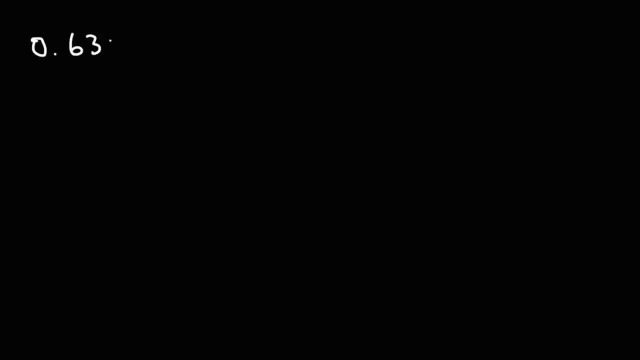 Let's try another example. Let's say we have point six, Six, three, Two, three repeating. Go ahead and convert this decimal into a fraction. So the repeating part is point twenty three. To find the non repeating part, Type this in your calculator. 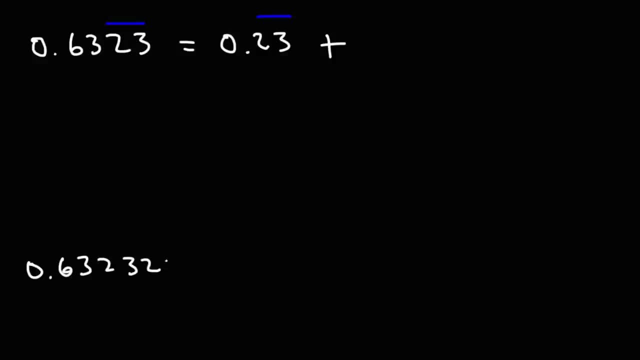 Point six, three, two, three, two, three, And subtract it by the repeating part, So we have a total of Six digits After the decimal. So we're going to subtract it by point two, three, two, three, two, three, The same number of digits. 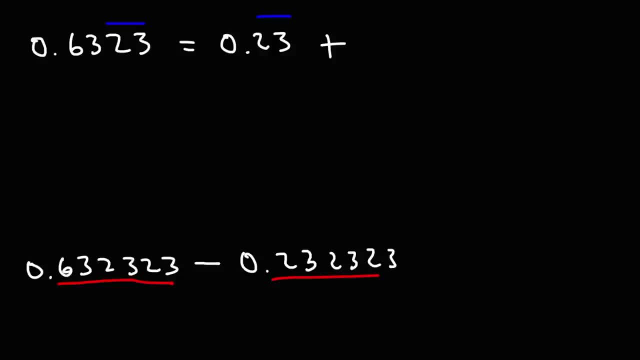 And you really don't need to use your calculator to see the answer. This part will cancel with this part. So what you're really doing is Point sixty three Minus point twenty three. Sixty three minus twenty three is forty, So we get point four. 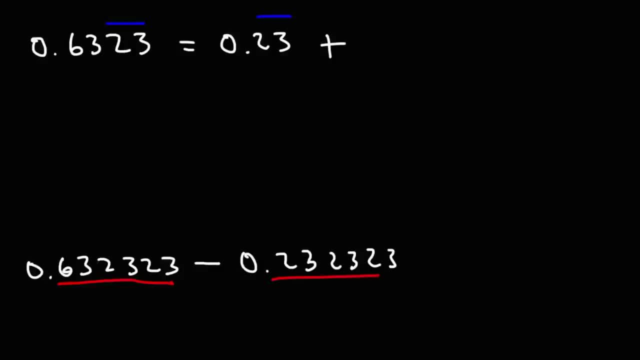 of digits And you really don't need to use your calculator to see the answer. This part will cancel with this part. So what you're really doing is .63 minus .23.. 63 minus 23 is 40.. So we get .4.. 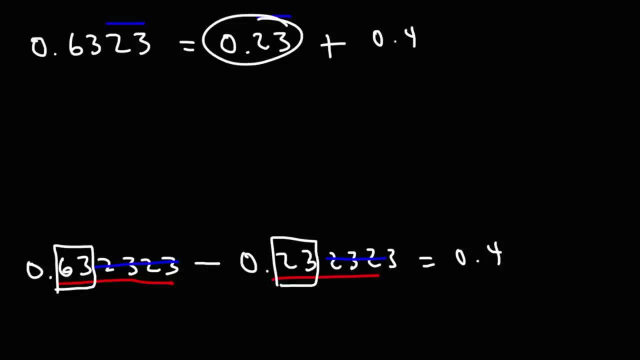 So this is .2 repeating, .23 repeating plus .4.. If you just focus on this part here, if you add those two, you get .63.. So .23 repeating is 23 over 99.. .4 is 4 over 10.. 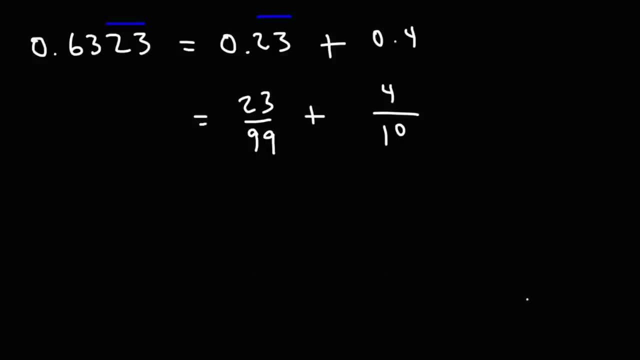 So what we need to do now is we need to add those two fractions. So I'm going to multiply this one by 10 over 10, and the other one by 99 over 99.. 10 times 23 is 230.. 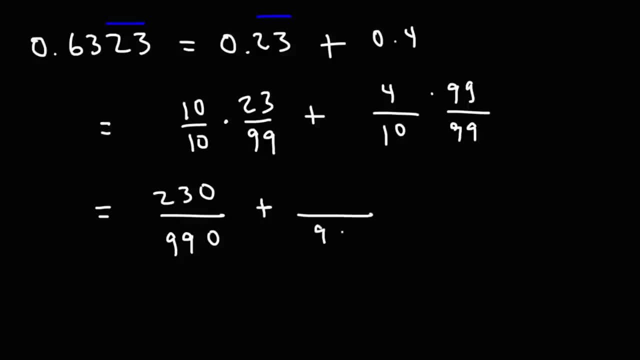 The common denominator will be 990.. Now, 4 times 99 is 100 minus 1.. Think of 99 as 100 minus 1.. 4 times 100 is 400.. 4 times negative 1 is negative 4.. 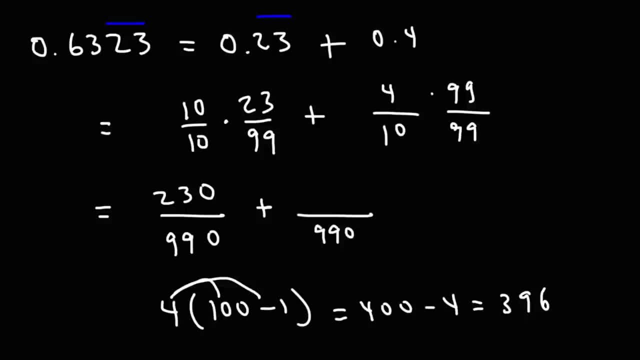 So this is 396. And that's what 4 times 99 is: It's 396.. So now we need to add 230 plus 396. And so that's going to be 626.. Over 990.. Now we have two even. 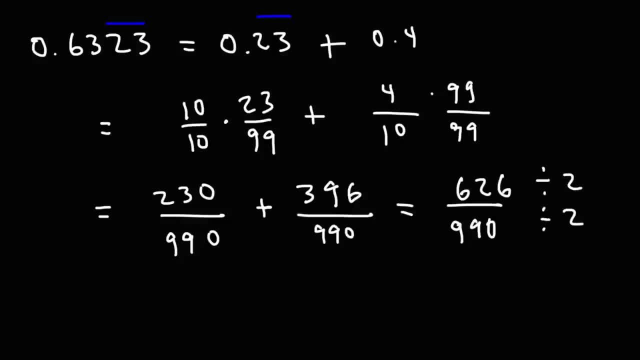 numbers. so let's divide the top and the bottom by 2.. 626 divided by 2 is 313.. 990 divided by 2.. 900 divided by 2 is 450.. 90 divided by 2 is 45.. 450 plus. 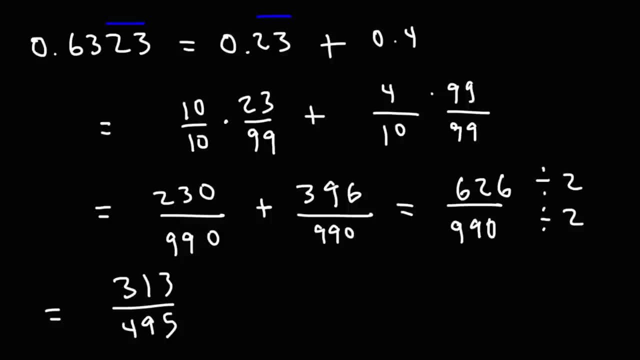 45 is 495.. So this is going to be the final answer. Now let's work on one more example. Let's say we have 0.58 and 1, 3 repeating. Go ahead and convert this into a fraction. So let's begin by writing. 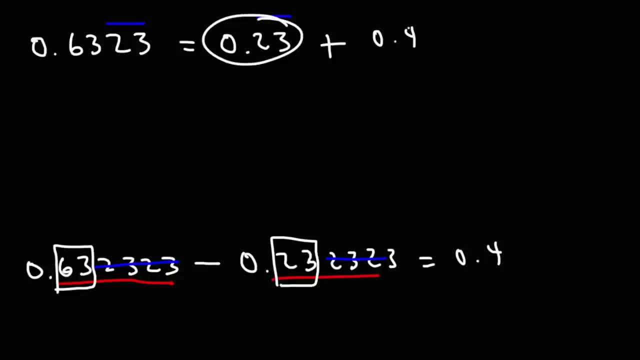 So this is Point two repeating. Point two, three repeating Plus point four. If you just focus on this part here, If you add those two, you get point sixty three. So point twenty three, repeating Is twenty three over ninety nine. Point four: 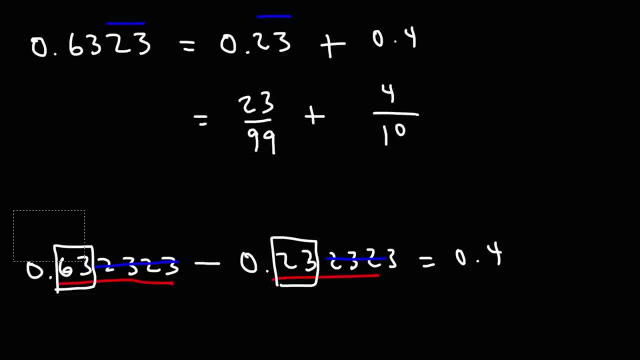 Is four over ten. So what we need to do now Is we need to add Those two fractions. So I'm going to multiply this one by Ten over ten And the other one by Ninety nine over ninety. nine. Ten times twenty three is two thirty. 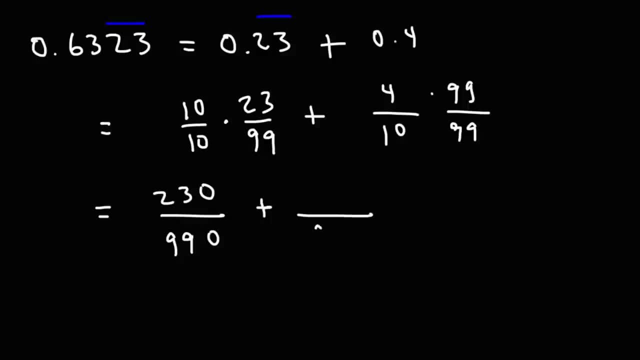 The common denominator will be Nine. ninety, Now four times ninety nine. Think of ninety nine as a hundred Minus one. Four times a hundred Is four hundred. Four times negative one is negative four. So this is three ninety six. 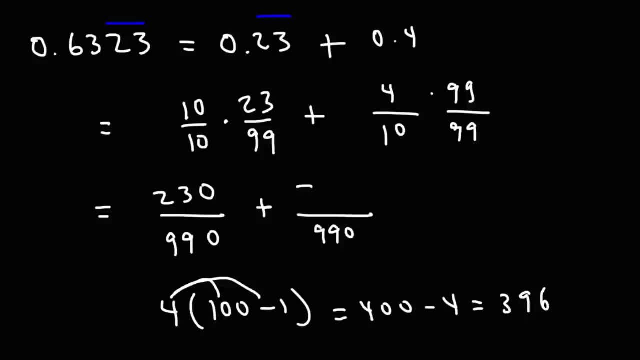 And that's what four times ninety nine is. It's three hundred ninety six. So now we need to add two thirty Plus three ninety six, And so that's going to be six hundred and twenty six Over Nine ninety. Now we have two. 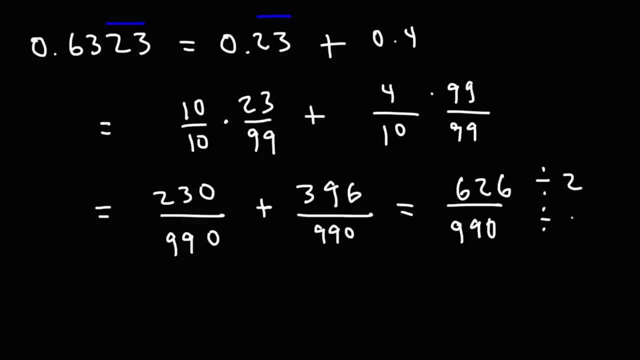 Now we have two even numbers, so let's divide the top and the bottom by 2.. 626 divided by 2 is 313.. 990 divided by 2.. 900 divided by 2 is 450.. 90 divided by 2 is 45.. 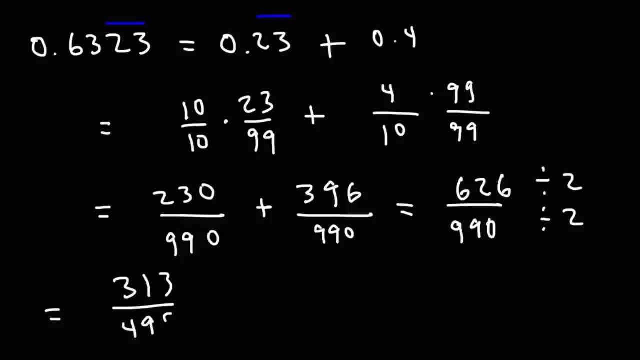 450 plus 45 is 495.. So this is going to be the final answer. Now let's work on one more example. Let's say we have 0.5813 repeating. Go ahead and convert this into a fraction. 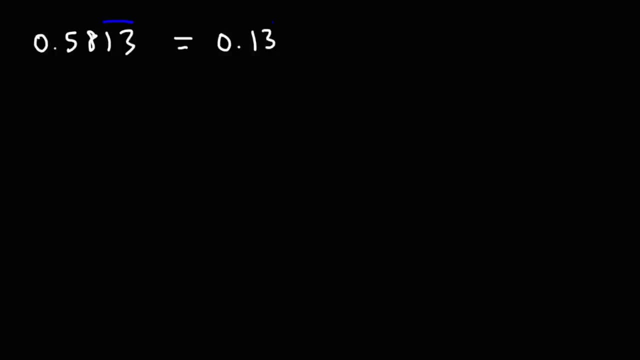 So let's begin by writing the portion that is repeating, that's 0.13.. If we subtract 0.58 by 0.13,, 58 minus 13 is 45. So the missing part is 0.45..